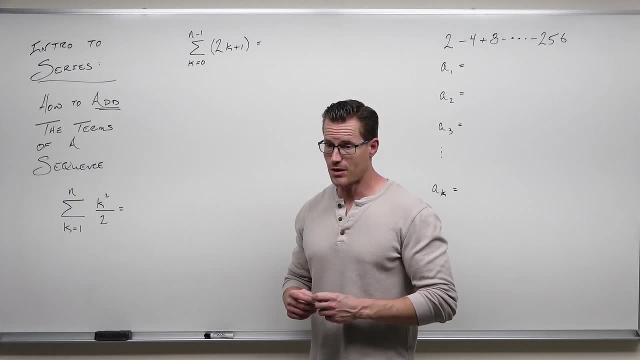 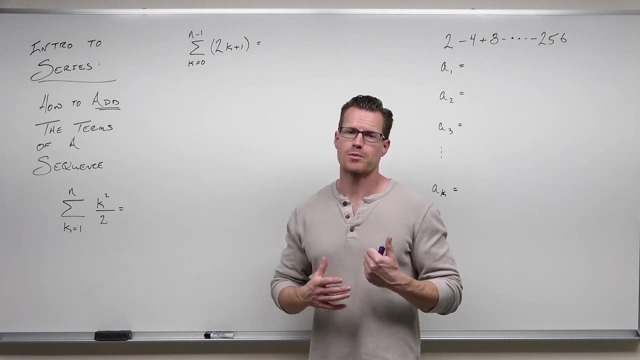 Welcome to another video. In this video we're going to talk about series And with all the time we spent on sequences, it should be a little bit more understandable, because we already really explored a lot of the hardest parts in sequences. How do you take a series and go backwards? What's? 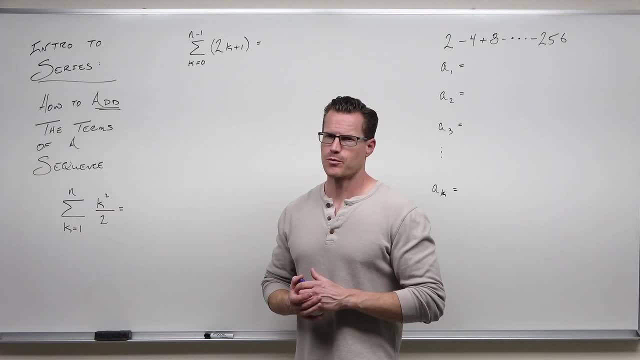 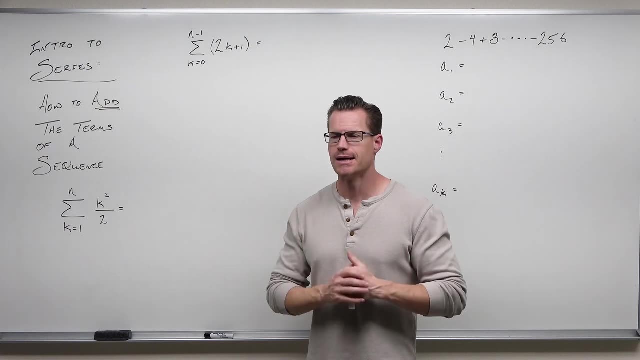 a series mean? What's it based on And are there formulas for it? The formulas are going to make the math so much easier for series. You see, here's what a series does. A series adds up the terms of a sequence, So they are not unrelated things that we have. They're not the same, And 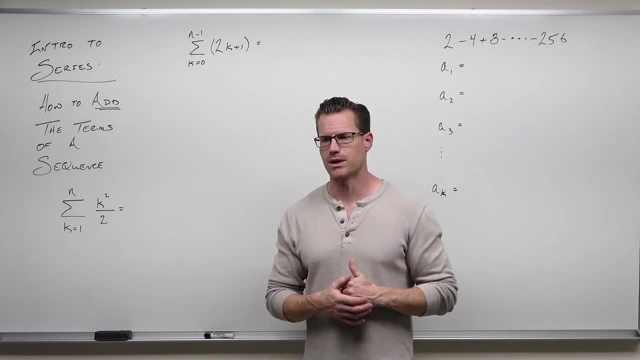 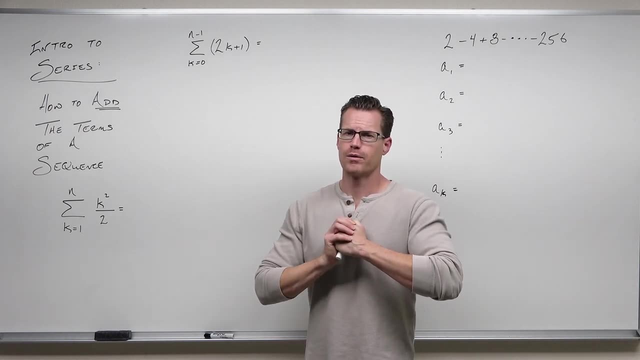 sequences in general are just a list of numbers And that's what we have. We can talk about convergence and divergence and things like that, But a series takes those terms and adds them. Now there's some very interesting things that happen with series, some very predictable. 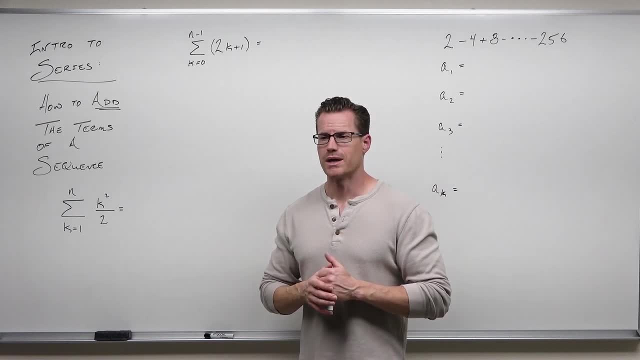 formulas that we can prove by proof by induction. We can prove a lot of these things And I'm going to show you how to do that when we get there and do proofs by induction. That's in a few videos from now, So we're going to be able to prove them. Some very interesting 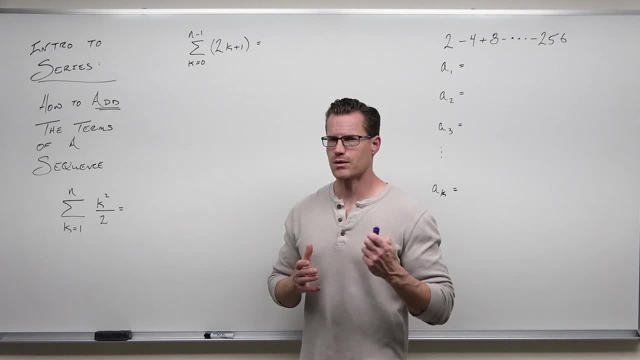 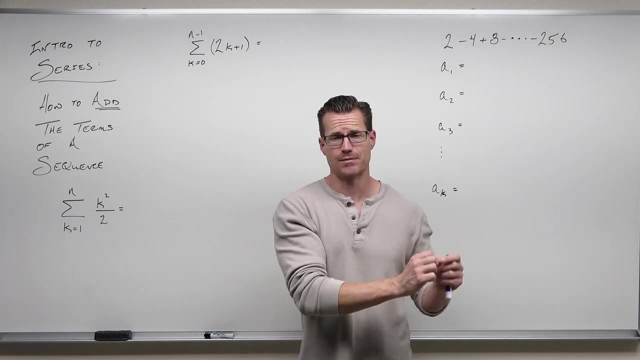 things happen And especially when we get into some calculus like calculus 2, we're going to find that you can actually add an infinite series, an infinite number of terms and get something It converges. There's some very special cases to do that. We talked about that in some geometric 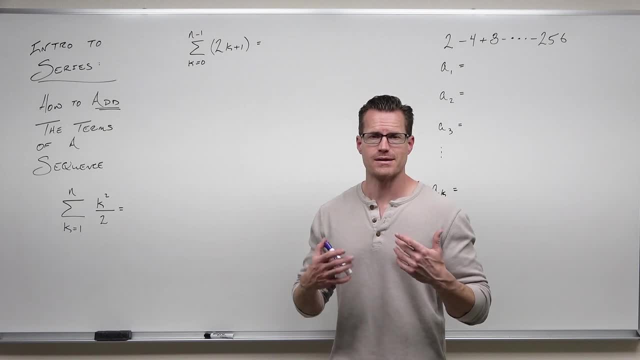 series in just a little while, But some very fascinating things happen. It's really worth our time to understand how a sequence works so that we can understand how a series works, so that we can understand how a series works, So that we can understand how a series works. 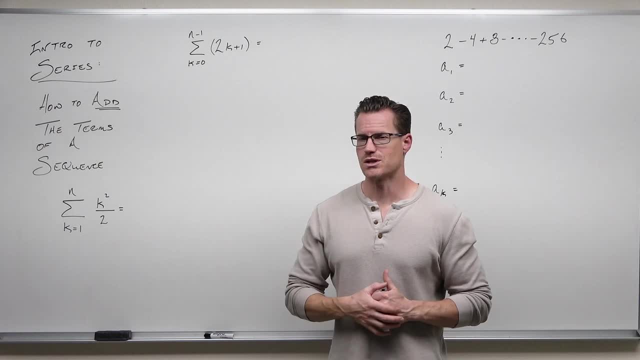 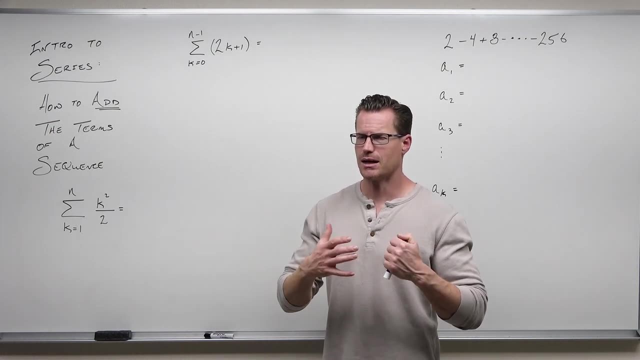 And we can understand a lot about some calculus later and do some very interesting things with it. I won't go into everything that we have, but some very interesting things happen with like pi and e and a lot of these numbers that are transcendental when we view them. 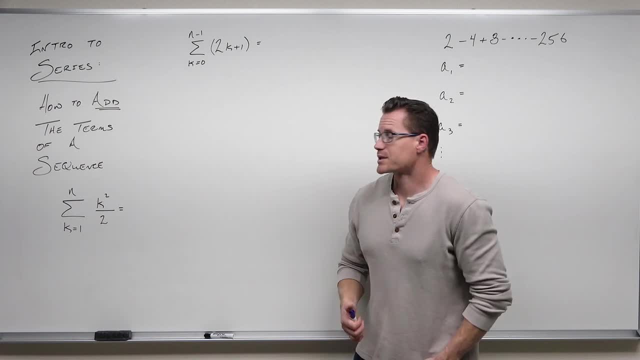 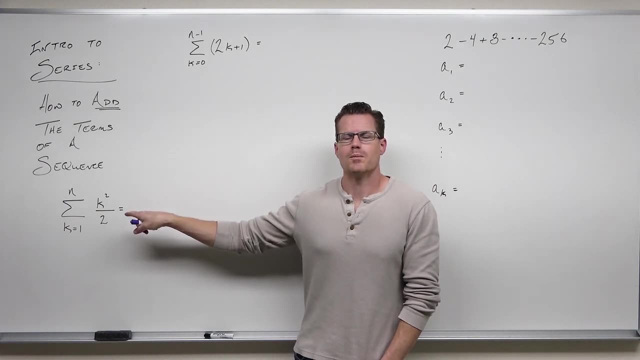 in a type of series. So here's what a series does and how they work. If you've never been exposed to it before, this is what they look like. What in the world does that mean? A series is just taking a sequence and adding up the terms. So here's what this tells you. 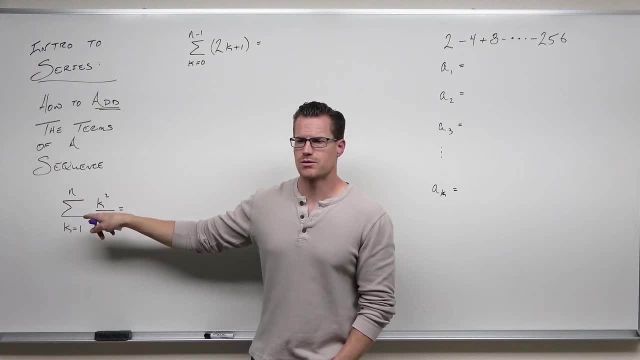 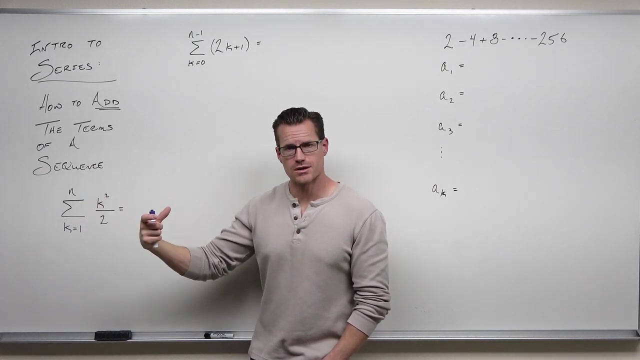 automatically This sigma is. it is a sigma, it's a Greek letter, s and it stands for a sum. Your sequence is right here. If you ignore this, that's just a sequence. In fact, your series tells you where to start and where to end, So your series is built like a sum. 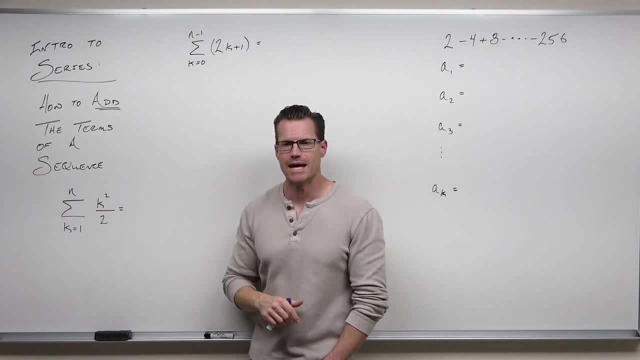 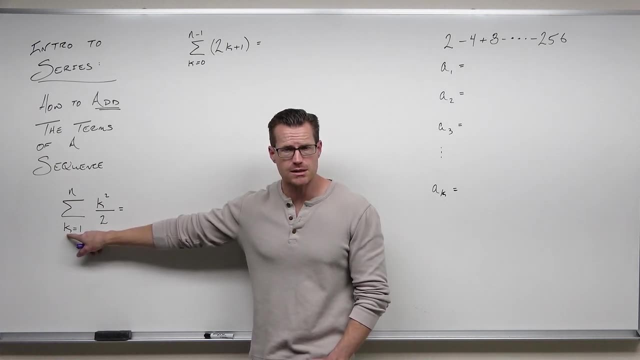 of a sequence. Could you find the first? let's say n terms of this: Well, if the series is telling you where to start, this says: I want you to look for your key. I want you to look for your K. whatever this index is, I want you to look for your K. Here's my K. 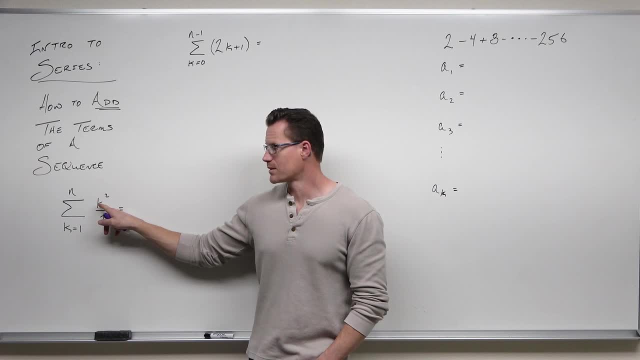 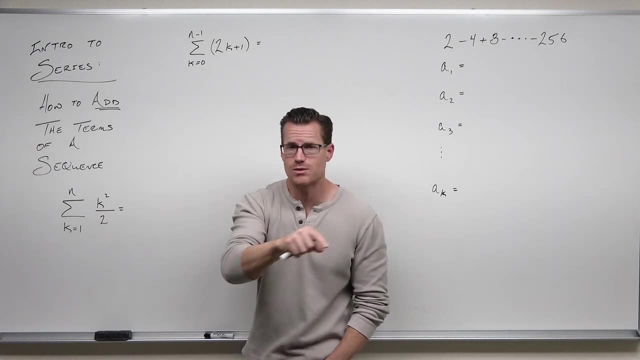 I want you to plug in one. Okay, I'm going to plug in one to this. It's going to give you my first term. Then I'm going to plug in two and three and four and the natural numbers, because it's based on a sequence. You don't plug in like 1.5.. You plug in all. 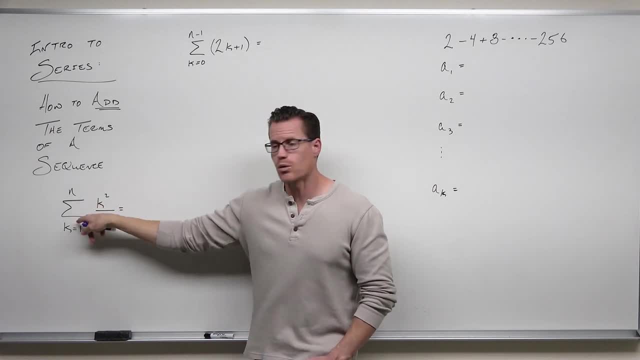 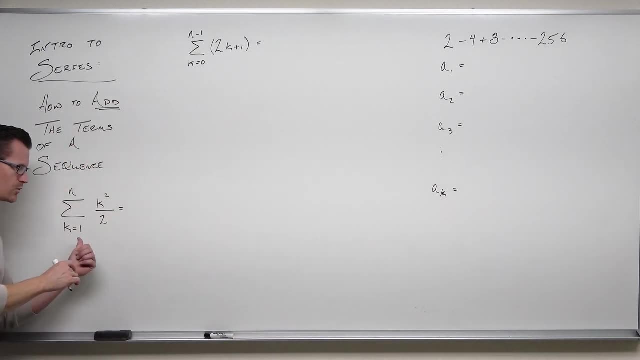 the natural numbers, because it is a sequence. You're just adding or summing it up until you get to that term. So here's what we would do, Starting with whatever this is. it could be zero, It could be one, It could be anything, It could be two, It could be three, It could. 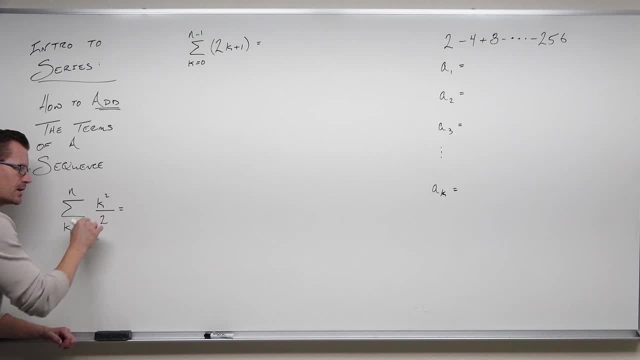 be four, It could be five, It could be six, It could be seven, It could be eight, It could be anything. Just start with what this is and plug it in. So our first term says: replace your index with one, and then two, and then three, until you get to whatever this is Now. 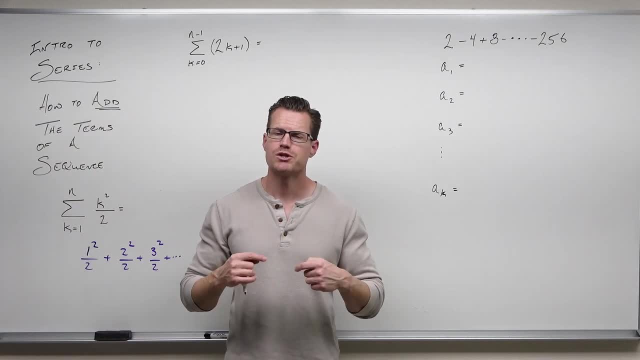 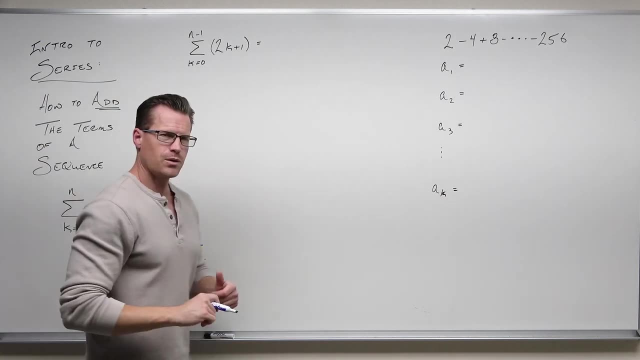 that's an N, So we're not going to be able to stop, but we show that we would do this continuously until we reach the N. Notice that it said. it said the two different letters that we have. This k is the index of your sequence. This n tells you. 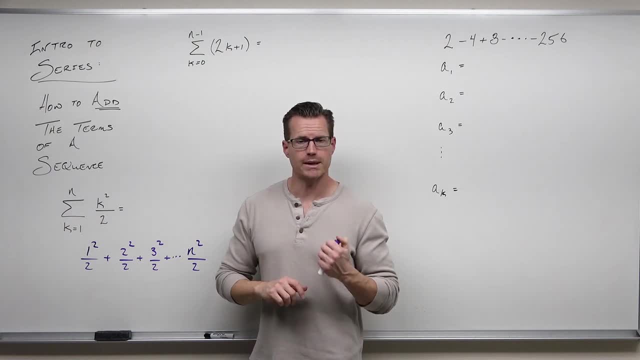 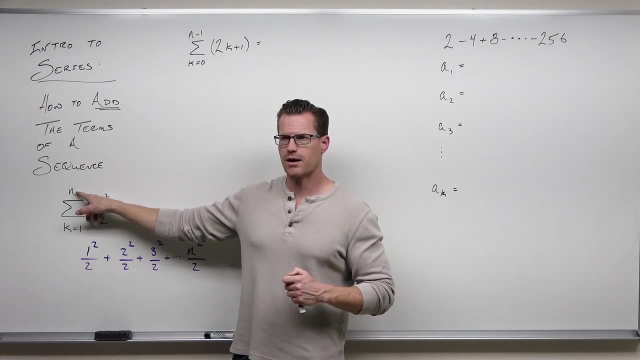 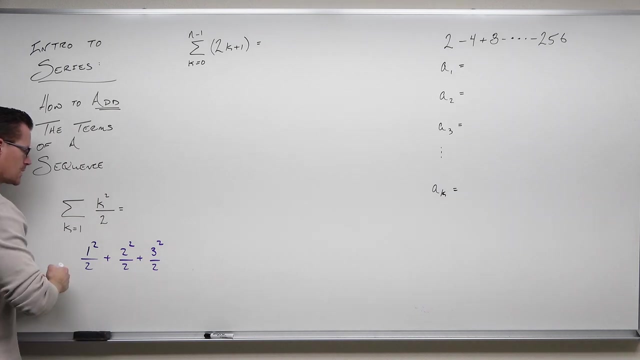 where to stop. Sometimes n is infinity, and it would be an infinite sequence. We get that a little bit later, But most of the time that is going to be an actual number. So what if that was? what if that had been three? If that had been three, it would be exactly this. It would. 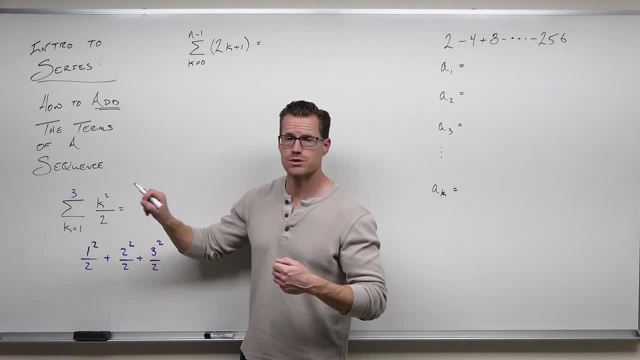 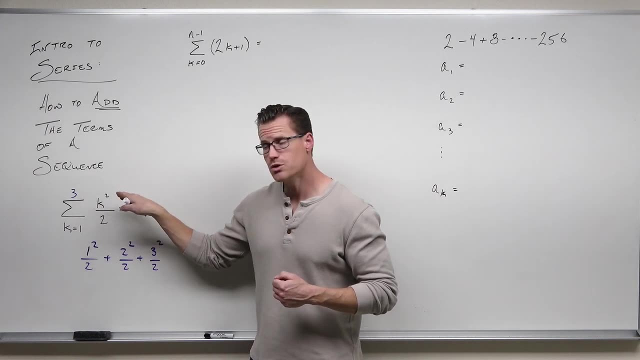 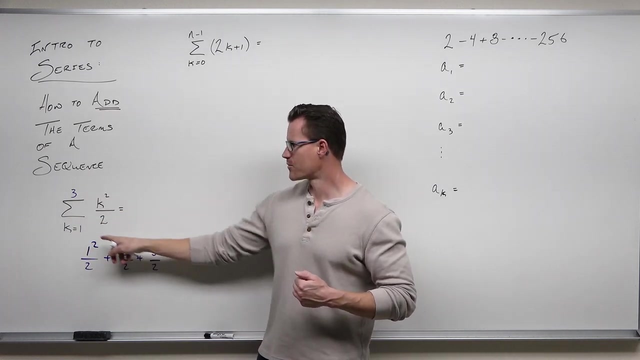 say: you plug in one, then two, then three, then you stop. That is how a series works. It takes these values starting here, plugs them into the sequence that you know how to deal with and stops with that term and then you add it up. So one, two and three from our one, our two and our. 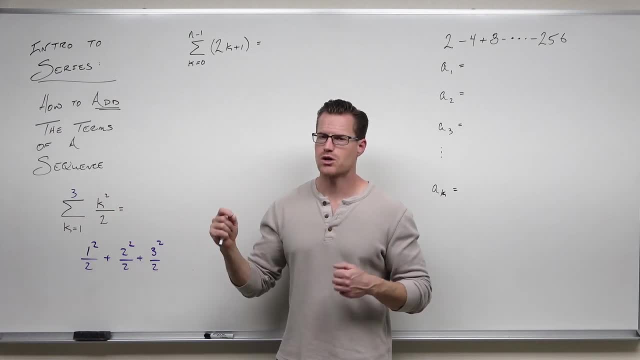 three, If that had been 31,. you do one, two, three, four, five, six, all the way to 31.. You plug them in here and you add the whole thing up. Is it possible? Yes, Is it annoying? Of course, 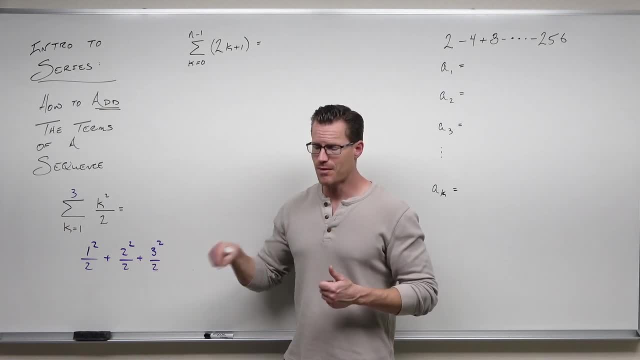 because if you have 31 terms here and you've got to add them up, that's a lot of number crunching. Are there formulas? Thank goodness there are. I'm going to show them to you in just a little while in this video on how you would do this quickly, very quickly, because there's formulas that allow. 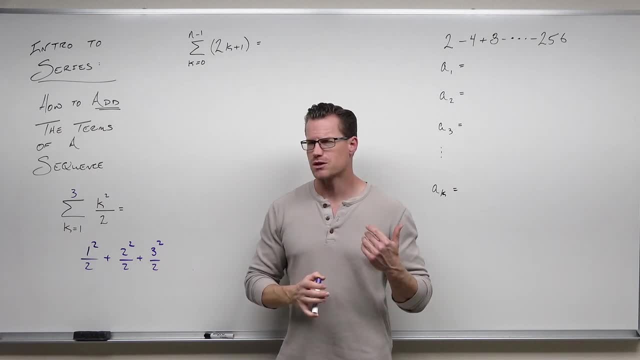 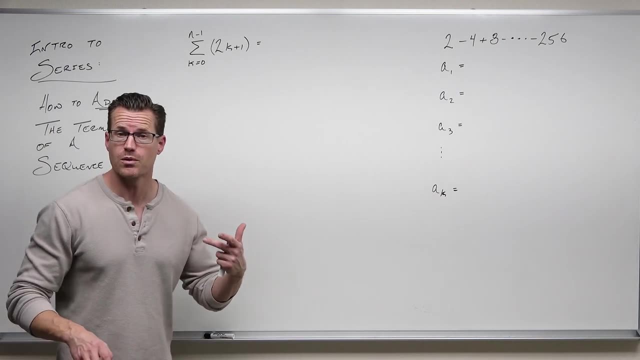 us to do that the k squared, So I'll show you those things when we get there. but in general, that's how the series works. I just intended to give you an example on how you'd find the first number of terms. The actual doing of a series is going to be a little bit different than what you. 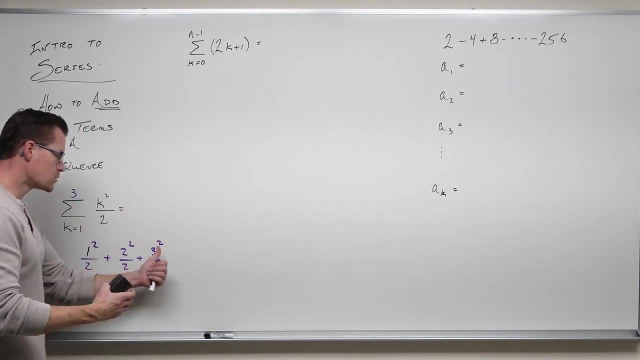 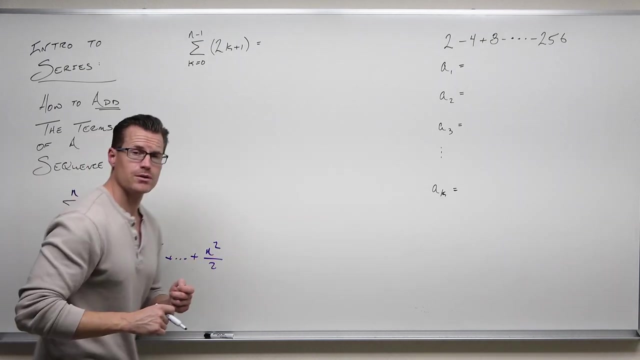 would do if you were doing the math and finding the sum. While you could do it this way, there's better ways. In most cases, there's better ways. If this was left as n, we would have to show that we continue until we reach whatever that number is. That's an important step to do for a proof. 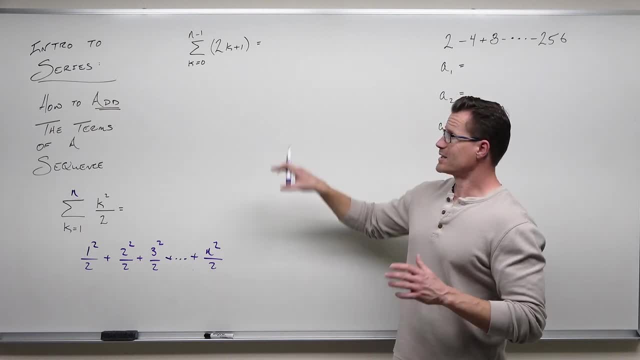 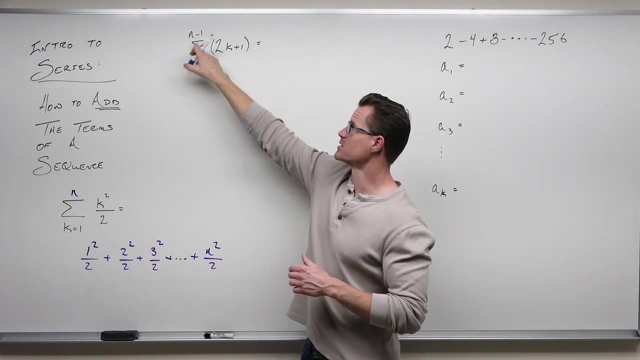 by induction when we finally get there. Okay, let's do one that looks a little bit more complicated. It's not going to be all that bad. This says that here's your series. here's the sequence on which this is built, So you're summing or adding the terms of this sequence. 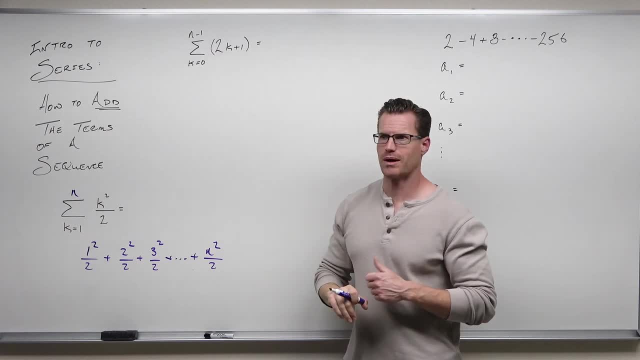 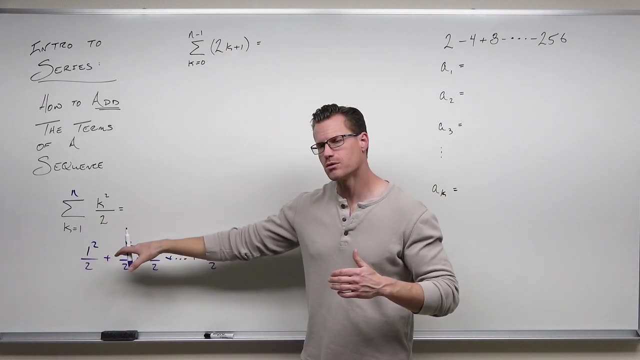 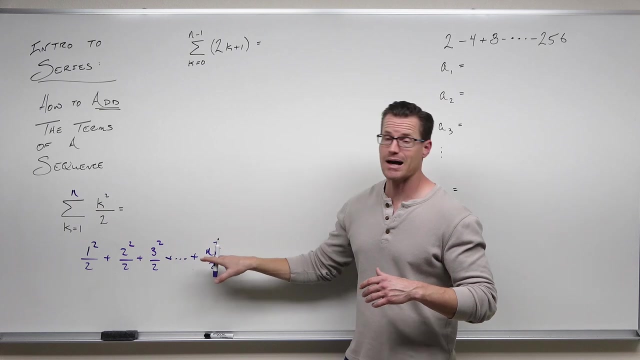 by starting at zero and ending at n minus one. How do I end at n minus one? You just plug in n minus one, just like we just plugged in n. You just start here, show a few terms, then go: yeah, some stuff happens and we end here. How do we end there? I took n and I plugged it in and we 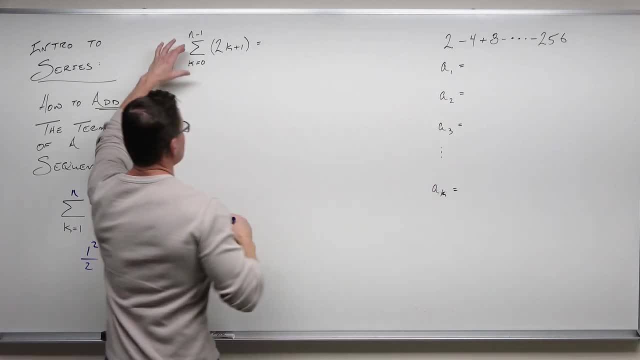 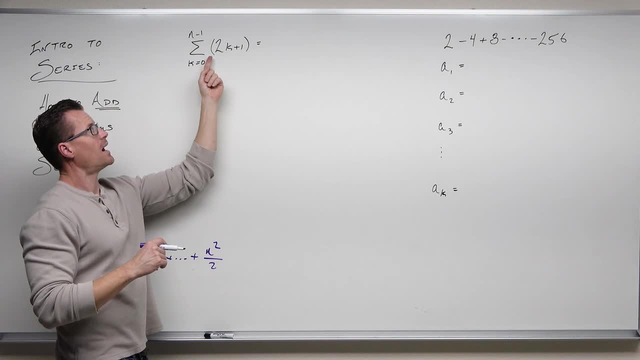 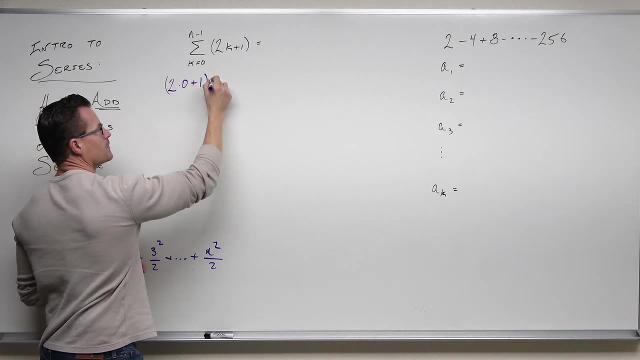 terms of the sequence, by starting at zero. So if I start at zero, I can do two times zero plus one. So if I start at zero, I can do two times zero plus one. The next term would be: I plug in one, then I plug in two, then I plug in three. It would give me. 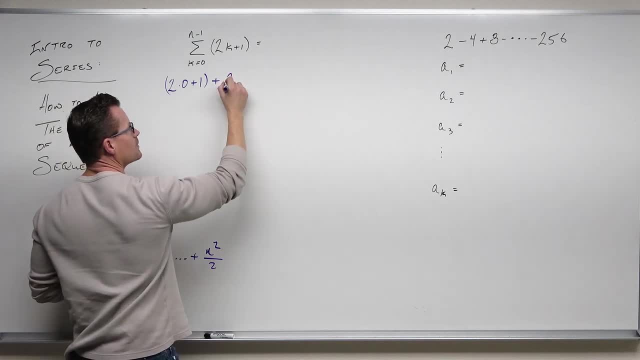 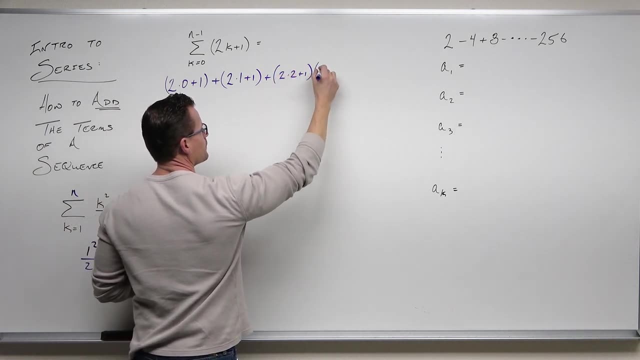 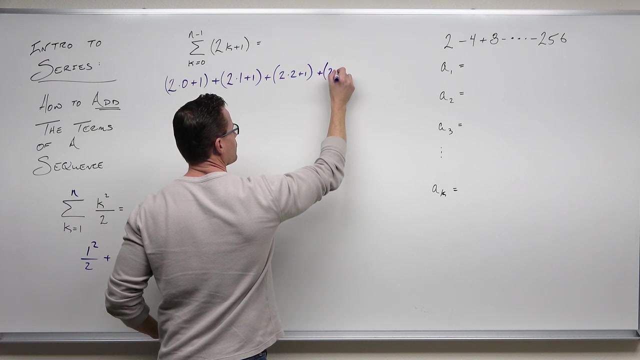 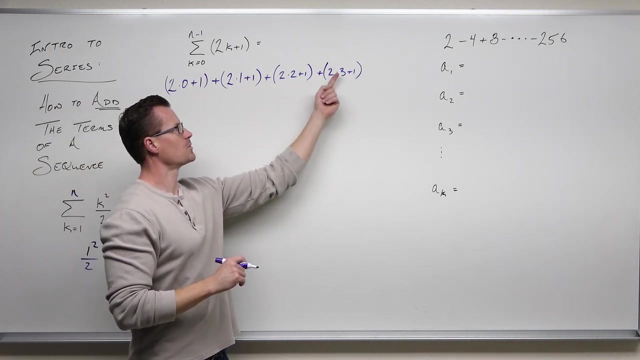 another term for each of those inputs. This is the zeroth term, the first term, second term, third term. You can consider it first term, second term, third term, fourth term, but you notice that you start at zero. so we typically 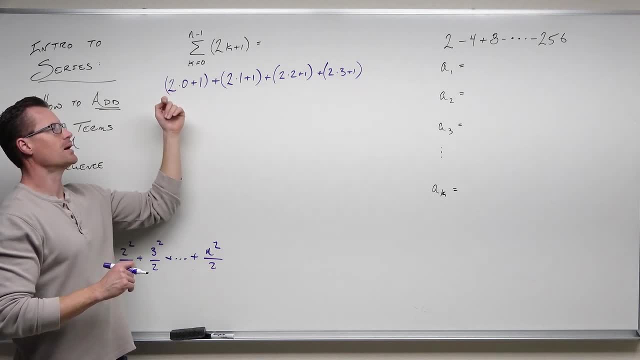 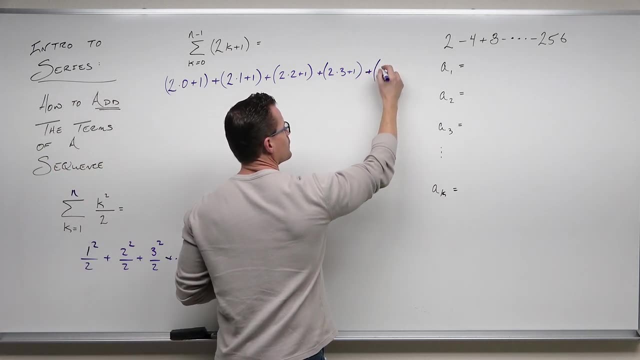 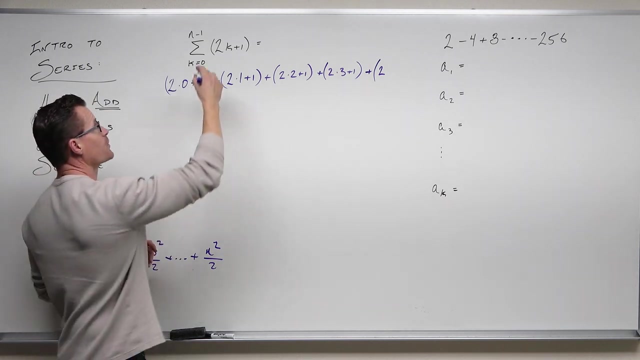 call it that case of zero, or the n sub zero term: n sub one, n sub two, n sub three, And where we would end is: take your two and plug in whatever that is. If we had had just watch this, if we. 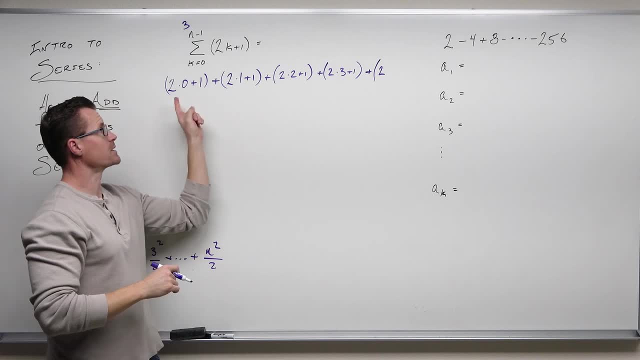 would have had a three here. this is where we would stop. We would plug in zero, one, two and three and we'd be done. That's it. That's all we would stop, or right where we'd stop. 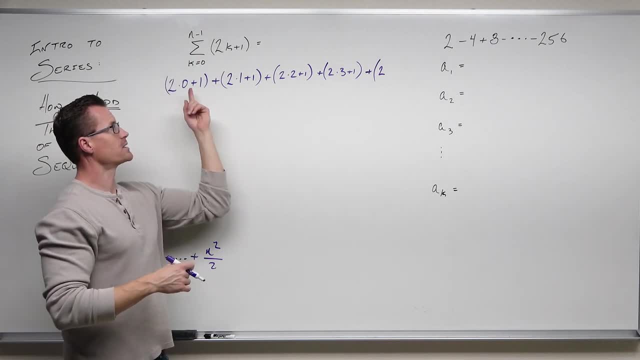 That's all we'd do. But if you have an n minus one, then you're going to go. okay, I'm plugging zero and then one, two, three, four, five, six, blah, blah, blah, blah, blah, blah, blah- going for. 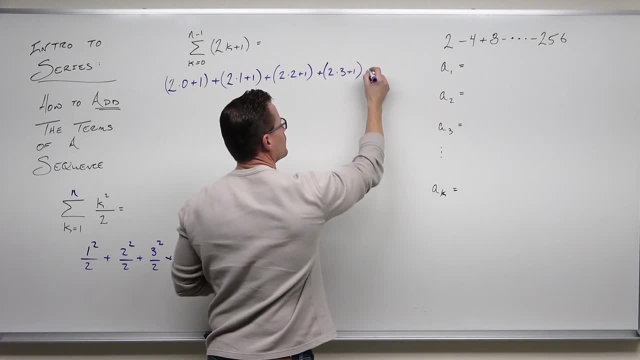 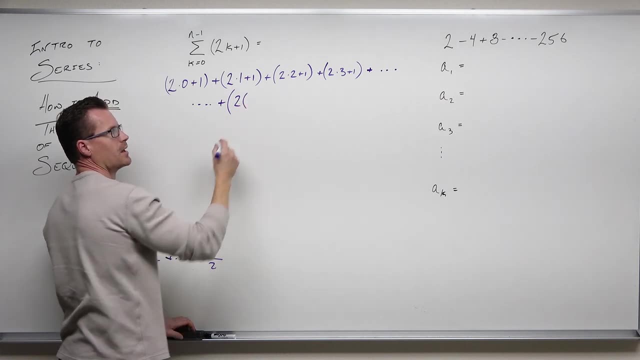 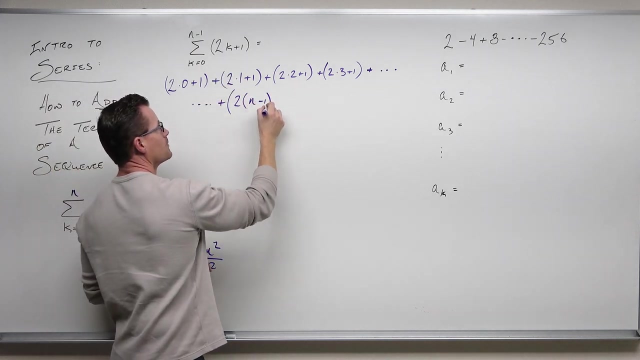 a Right down here Going for a really long time, and then you would have plug in two, or you have a two, plug in your n minus one plus one. It's just an evaluation. Like you plugged in zero and then one and then two. 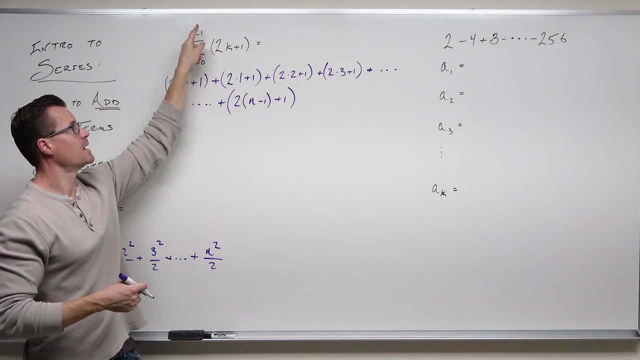 and then three, and then where you stop. So take this, evaluate it. That would be two times n minus one. You plug in zero and then one, and then two, and then three, and then where you stop. So you do have to have parentheses. I hope that you see it as a composition of functions. You're 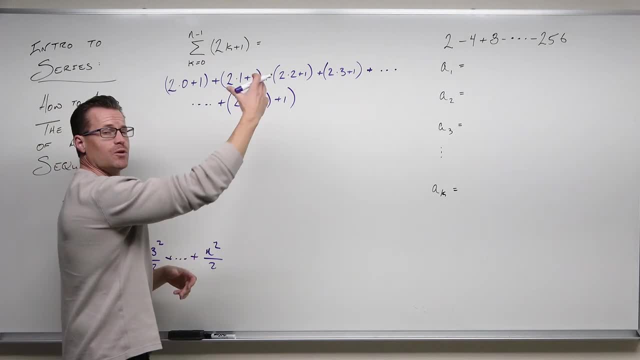 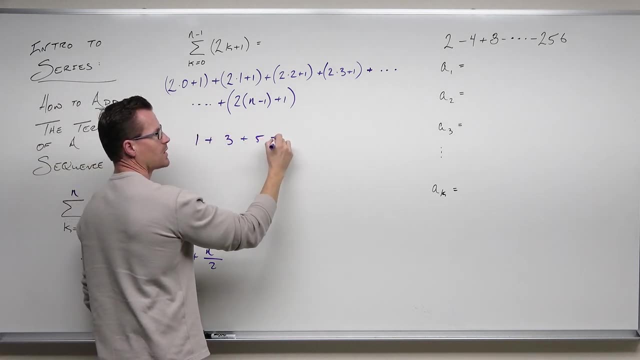 just plugging in one number, It's just n minus one, and you can simplify all this stuff. This would give you one plus three plus five plus seven plus. Look at what this does. This would be 2n minus two plus one. Wait a minute: 2n minus two, because I distributed plus one is 2n minus. 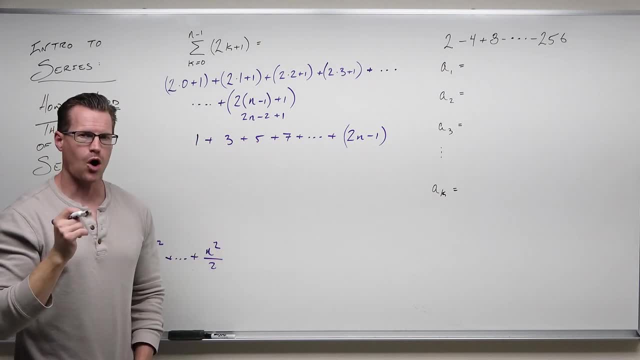 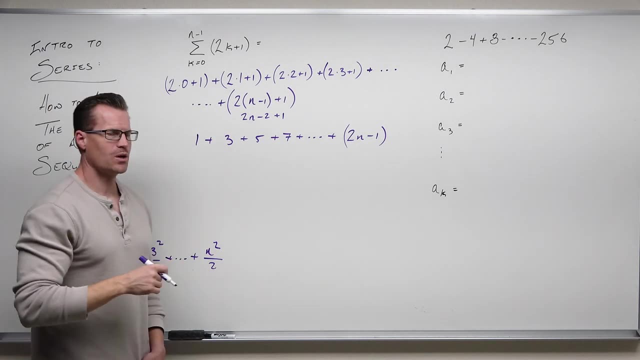 one. Isn't that exactly what we got? We got four odd numbers in the last video for sequences. Yeah, that's it. And this is really interesting because, if you notice this, you can define odd numbers two different ways. You can. 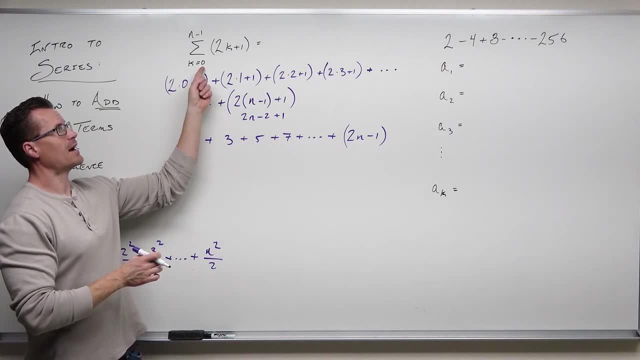 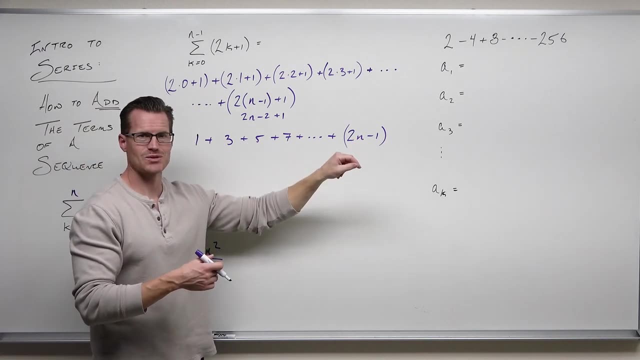 define them by? what if I started at zero? Well then I would have to have two times zero plus one to get one. What if I started at one? Then I have two times one minus one to get one. You can define them two different ways, And some of these series and sequences can be done that way. This defines: 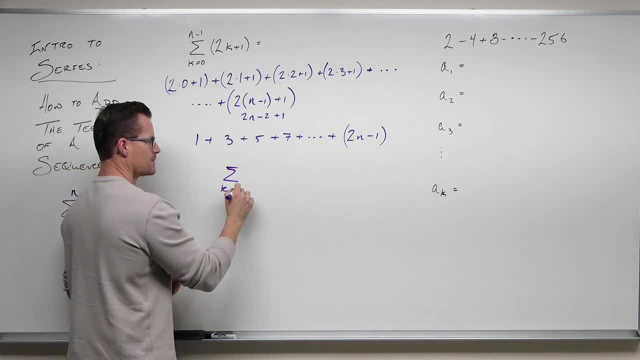 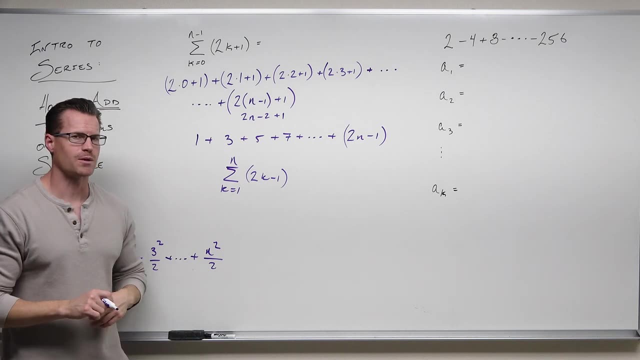 odd numbers the same way, So you can define them two different ways, And some of these series and sequences can be done the same way that this does, If you think about it and you want to do it on your own, I might spend a lot of time on it, but if you think about it, 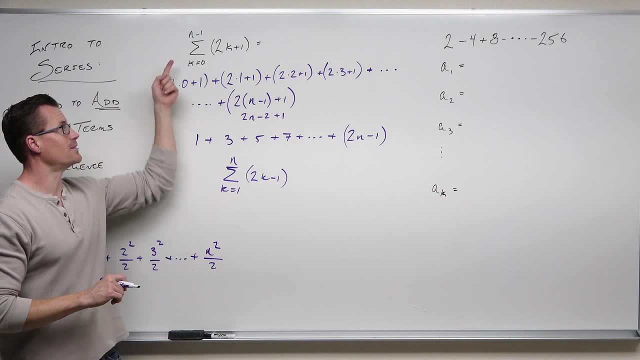 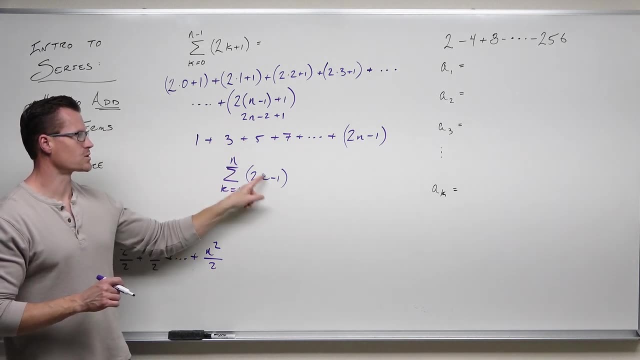 this is going to give you exactly the same thing that this does, Exactly. Plug in one. Two times one minus one is one. Plug in two. Two times two minus one is three. Plug in three, That would five. Plug in seven, That would be. 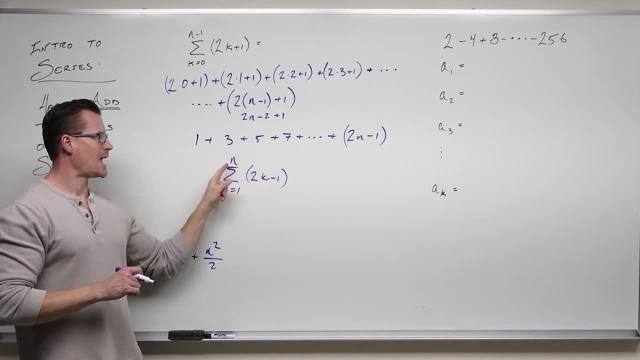 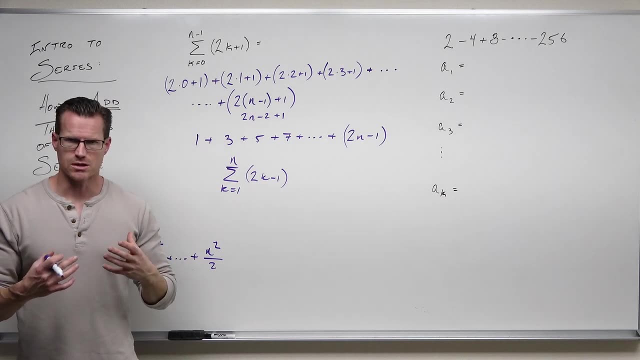 seven. Oh sorry, plug in four, That would be seven. Plug in n. Plug in n, That would be responsible. So we'll n you get 2n minus 1, 2n minus 1.. Same stuff. So this does teach something that says that you can. 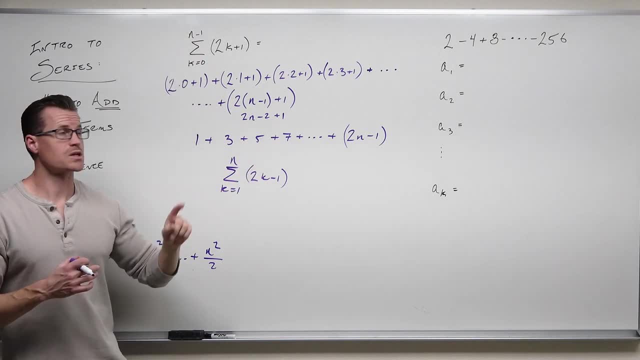 manipulate one series into being something else by altering where you start and where you stop, and it might even change your sequence that you're working with. So I hope that makes sense. I'm trying to teach you some pretty advanced things just by looking through a couple of examples here. 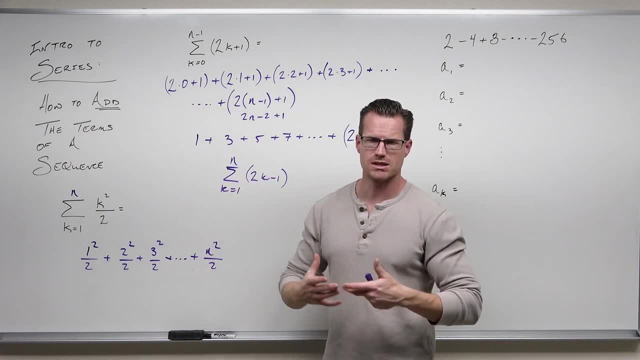 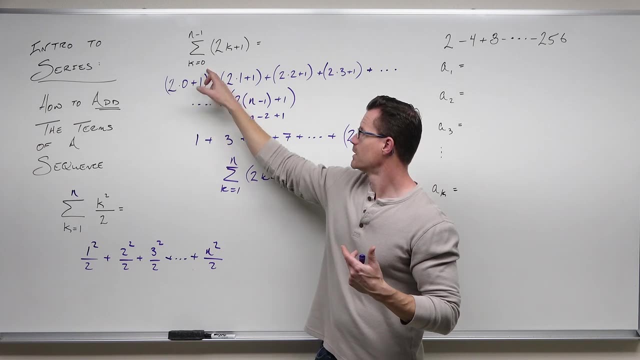 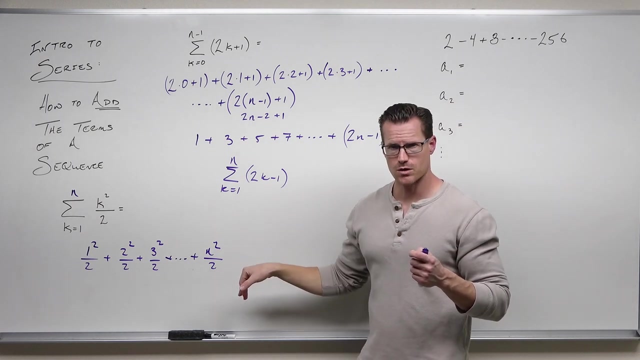 So, in general, a sequence is a series. It's just a sequence added up. The sequence is given to you. it tells you where to start, it tells you where to stop. Those can be finite numbers in which you have a finite number of terms, or they can be left as n. 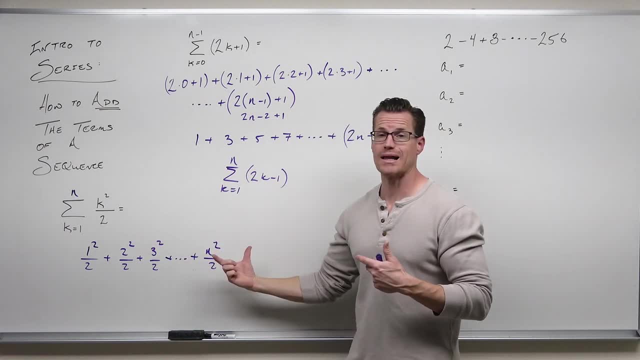 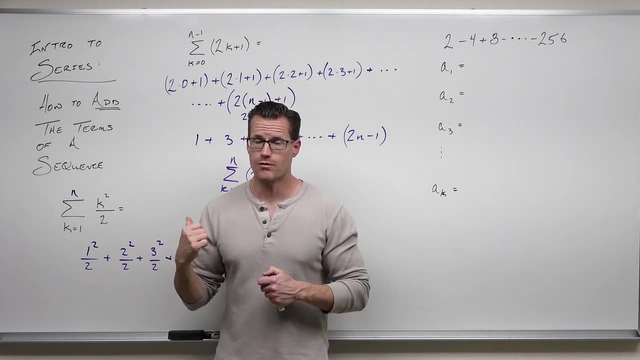 n, n minus 1, in which you have an infinite number of terms and you just show what that last term is by plugging in or evaluating your n. That's all that series do In general. we're going to see that there's some formulas that would solve all of these things for us very nicely. and let us add: 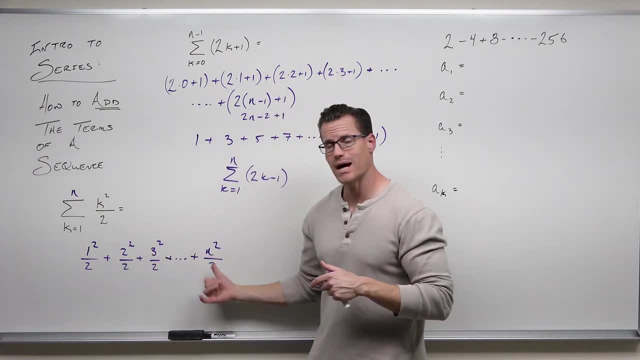 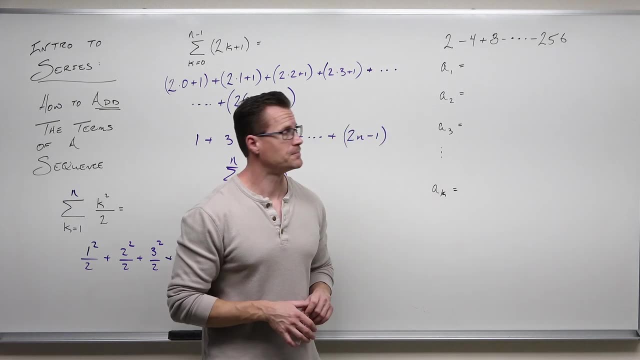 up the terms of your sequence without having to do anything else. So if you're going to do something, you're going to do a whole lot of writing out, because this is annoying and if you went to 50 terms, that'd be crazy. That would take you so much time. We have a better way, All right. another: 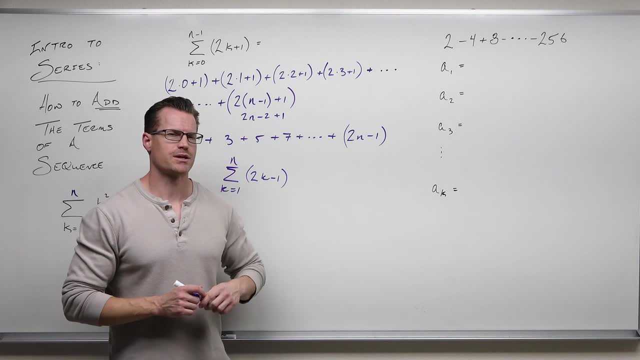 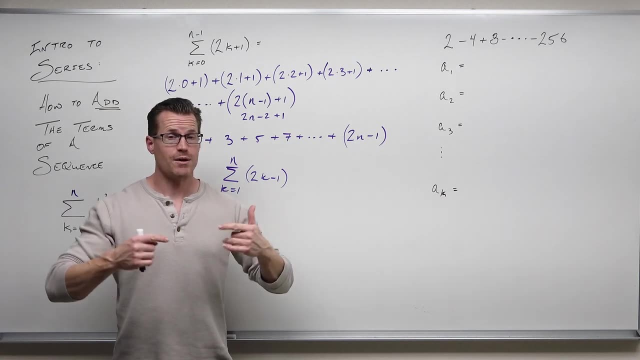 thing that we can do is we can go backwards on a series like we went backwards on a sequence. We can build a series from a sum, and so we're going to show that it is the same exact technique. So if you have not watched the sequence video on how we build a sequence from a list of numbers, 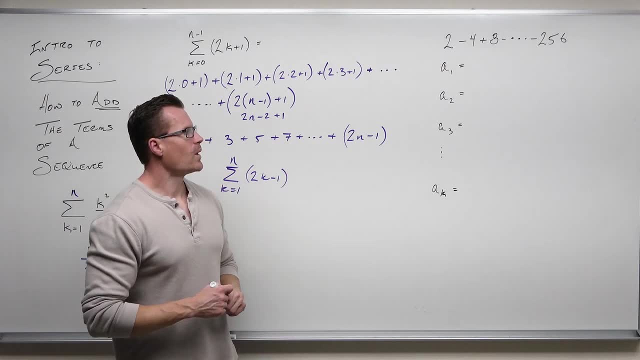 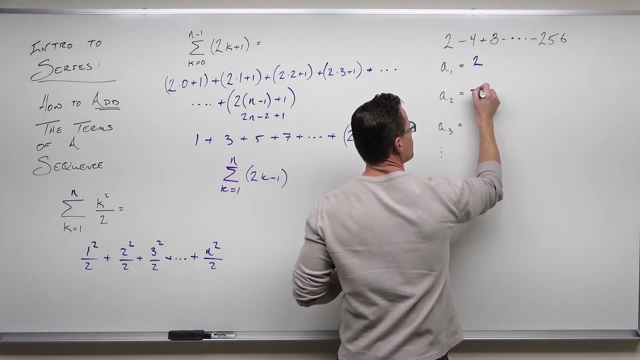 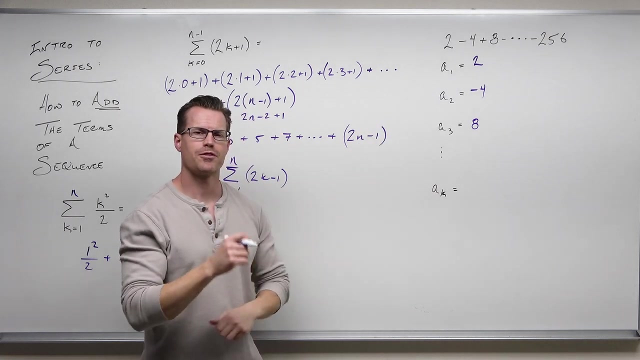 you need to, because we're going to do the same thing here, but quicker. So how we do this? the same exact idea is: take whatever you're given and write the terms down. So we have two, then negative four, then eight, and those are being added. The next term: think about what the next term would be. 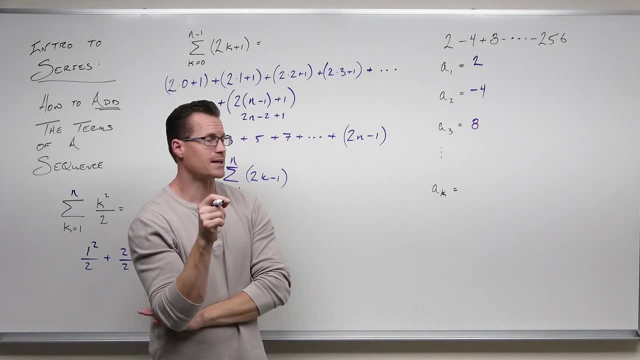 The next term would be: let's see two negative four. oh wait, it's not six, it's eight. These are not just even numbers, because I'd skip one, Two negative four, eight and the next one would: 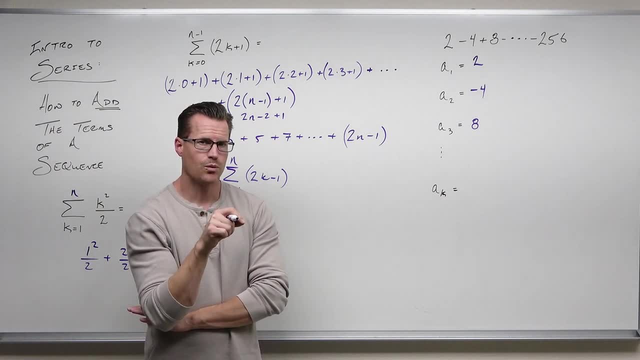 be negative 16.. So, if you remember, what we're trying to do is we're trying to make sure that we're going to make all of these the same form and then figure out the stuff that's not changing in it and then relate it back to our n, our index. Now there is one other thing here. This: 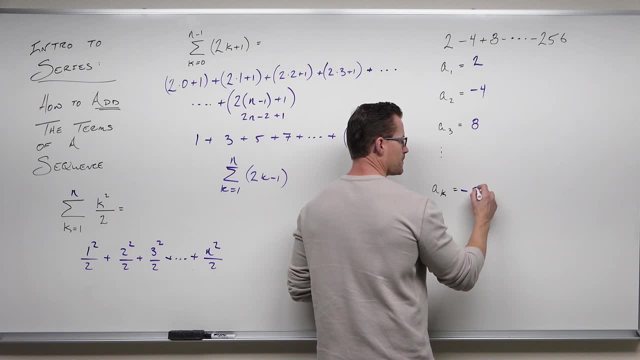 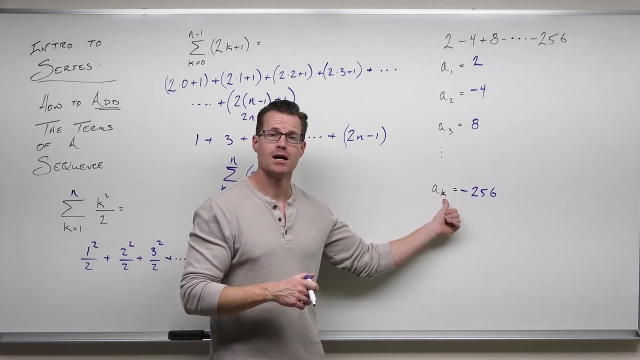 series stops. This series does have something, some number, as a stopping point, So we're going to have to figure this out. We're going to figure out what that k is, because we're going to write our series and have a finite number there. We're going to figure out what that is. It's actually. 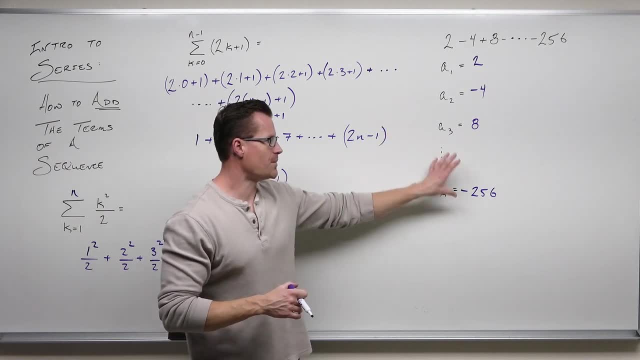 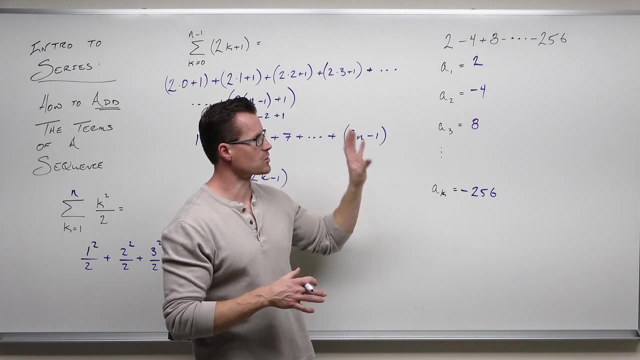 going to be eight, but we'll figure out what that is as we go. We're going to have to relate it back. I'll do a different example, like if you weren't given that, how you would do it, how it would change. but this is the way we go through it. We list our terms out. 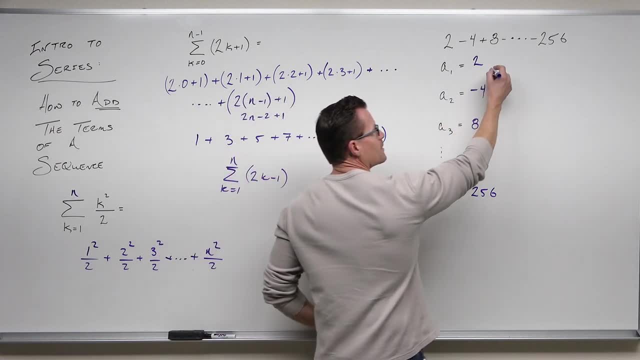 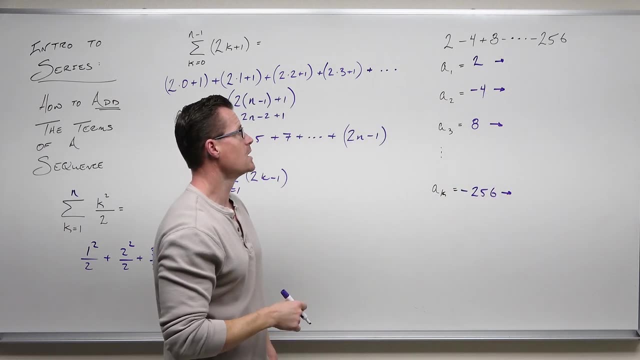 then we try to make them all the same form. What do we mean? Try to make them look like they have the same stuff and represent the stuff. that's the same as unchanging things in your series. So I'm looking at this going: hey, I have a negative here, a negative here and no negatives. 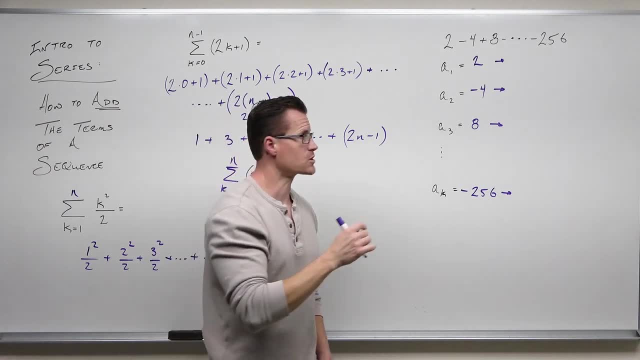 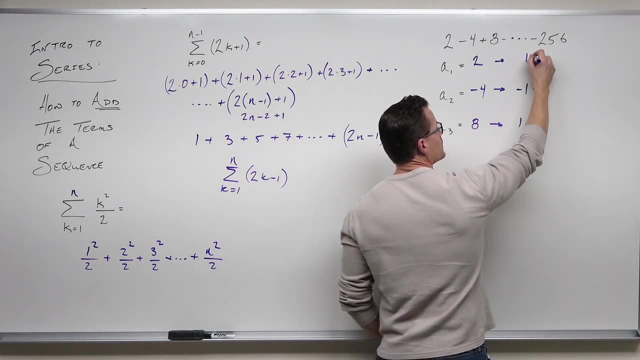 here. I'm going to relate this to a negative one eventually. So I'm going to say this is negative one times four. I'm going to say this is negative one times four. I'm going to say this is negative one times eight. one times two. negative one times 256. 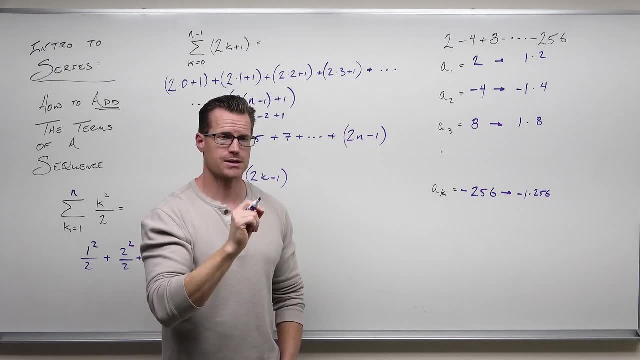 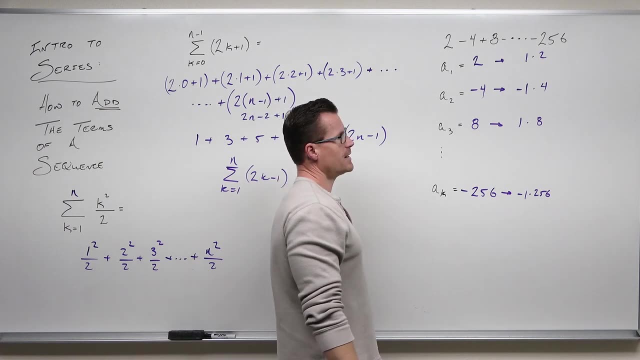 So I know that there's a one in there that's not a negative one in there. that's not changing. My exponent will be changing. We talked about alternation, so we're going to have that in our series. The next thing I do is look at our two, four, eight and 256 and try to relate. 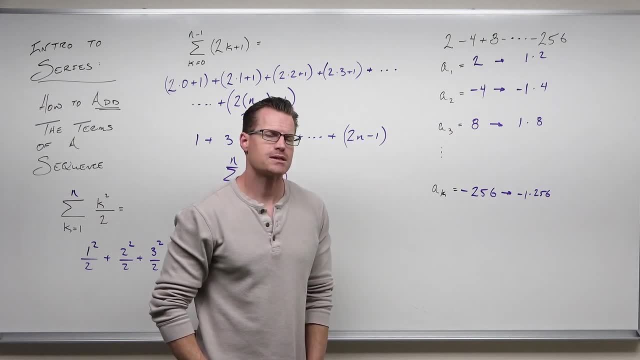 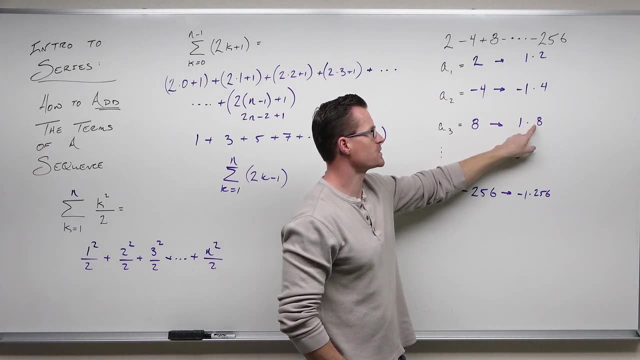 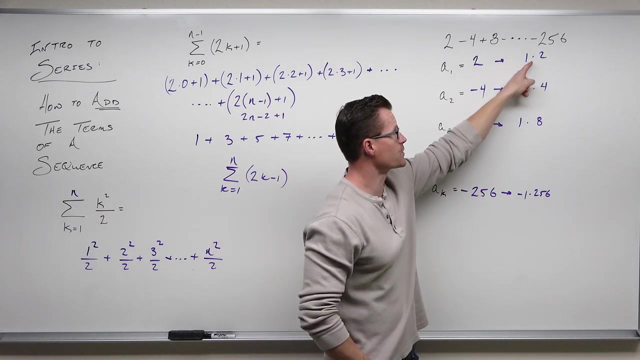 them to the same thing, something that's not changing. Now, this is not even numbers, so it can't just be two times, something like two times one, two times two, two times wait, two times four, two times. that doesn't work, but they are all powers of two, So this is two to the first. 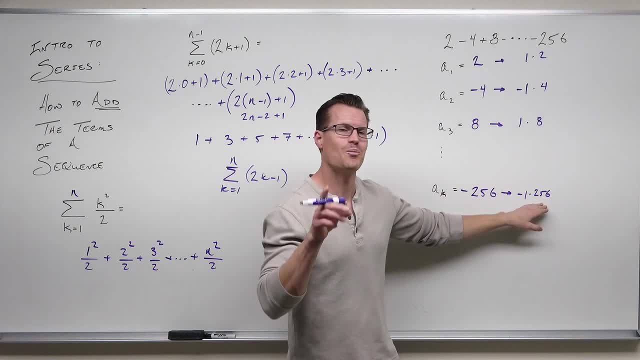 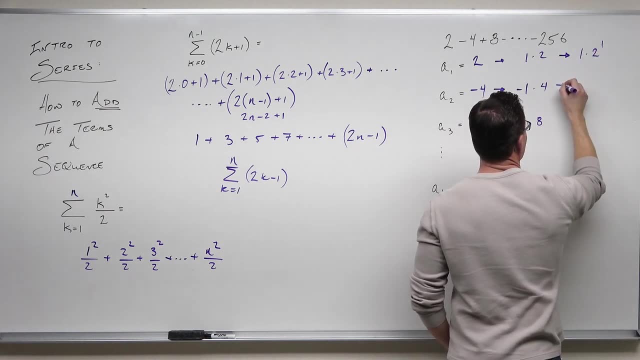 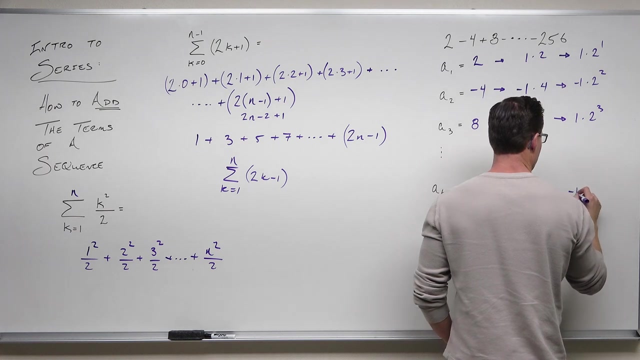 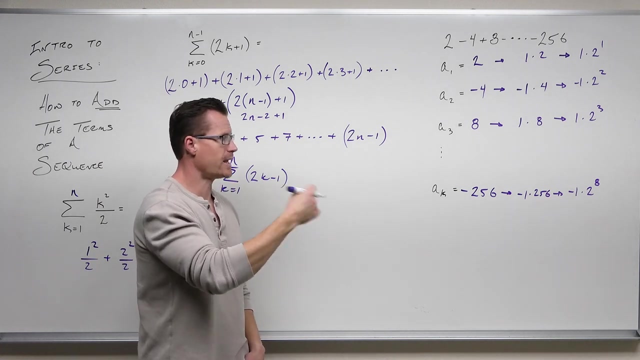 two to the second, two to the third, two to the. you have to figure that out, but it will answer that question for you. So two to the first, two to the second, two to the third, two to the eighth. The next one will. 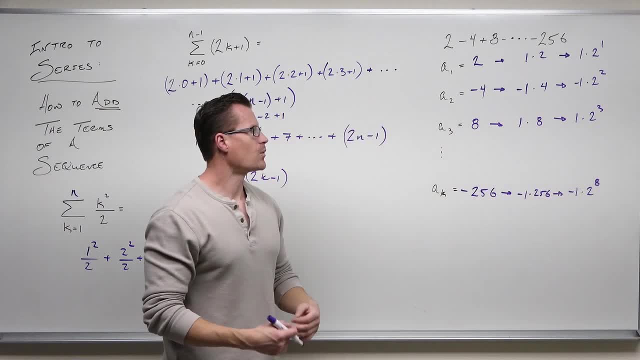 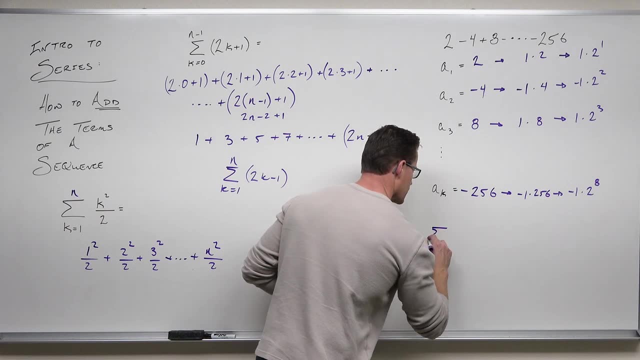 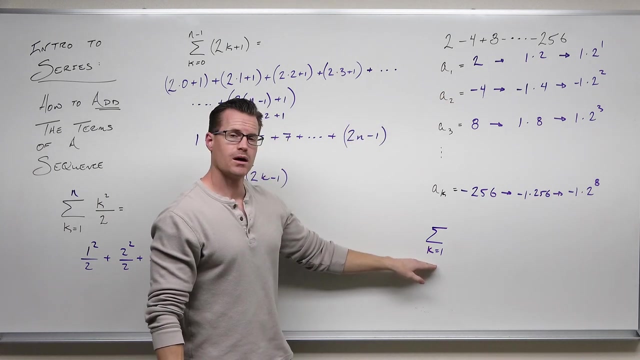 be a negative one times two to the fourth, And now we're ready to start making the jump for our series. So I know it's being added. so that says we have a series. I know I have to start at one, and so we're going to have this case of one. So I know that. 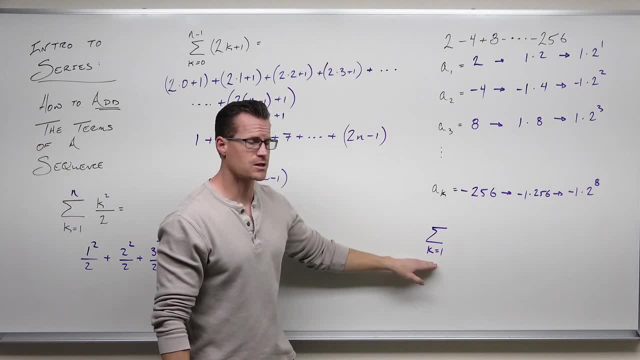 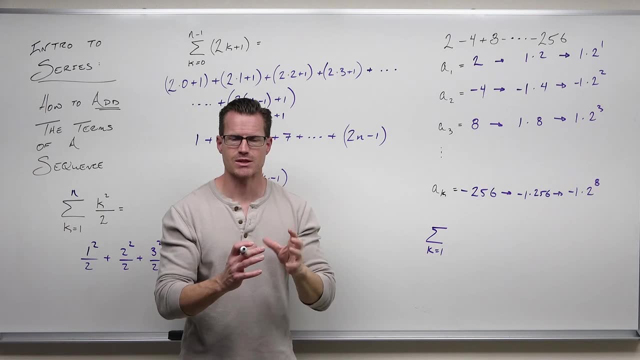 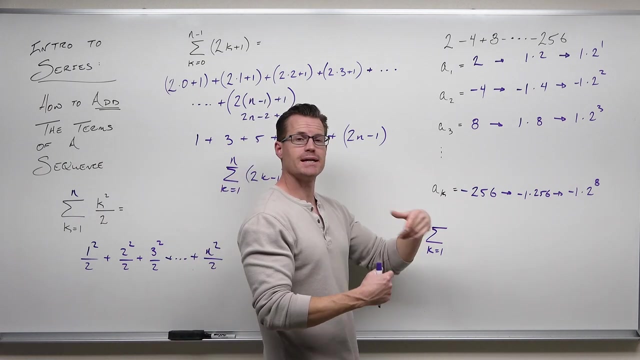 first term is going to be our first term in this series as well. I now need to start representing all of this stuff that's not changing, just like we did a sequence Why? Because a series is based on a sequence. You need to have the same exact sequence, So our sequence should have a negative. 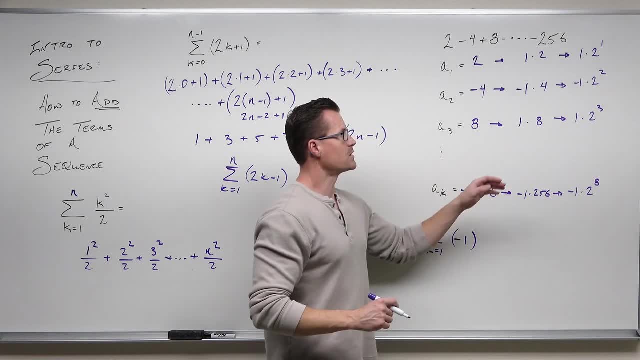 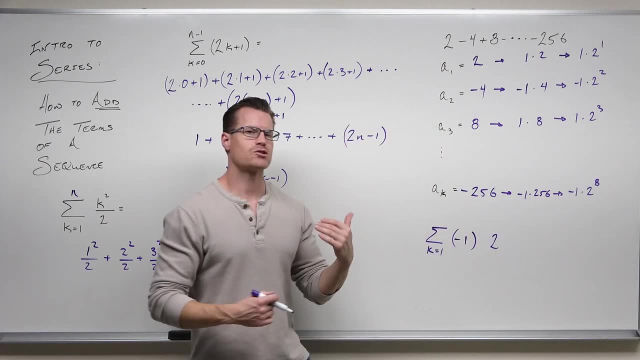 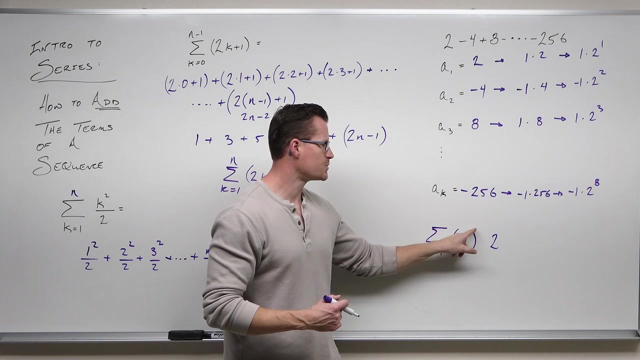 one in it. Our sequence should have a two in it, because the negative one and the two are not changing. What is changing? The sign of the first of our terms, our negative one, to a power that's changing. So the exponent here needs to model that. Well, let's take a look. Our first: 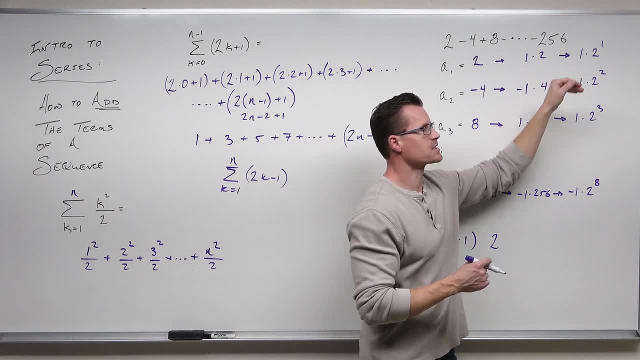 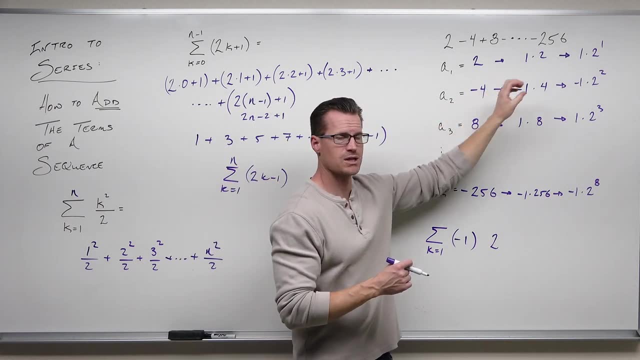 term is positive. So if our first term is positive, it needs to take negative one to some power and give me positive one. It needs to take negative one to some power for a second term and give me negative one. The way we do that is: we take our k. 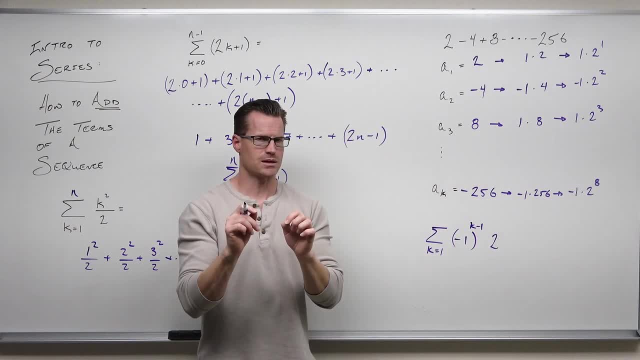 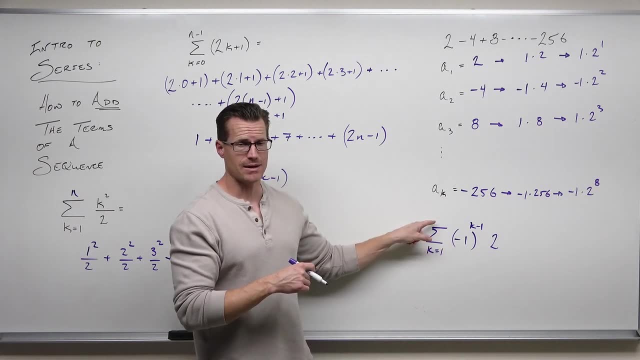 and we take our k, and we take our k And we subtract one. Now please get this. Why k and not n? K is the index for a series, because you show where you end. at the end, You want to be able to plug in that n and get your general term. 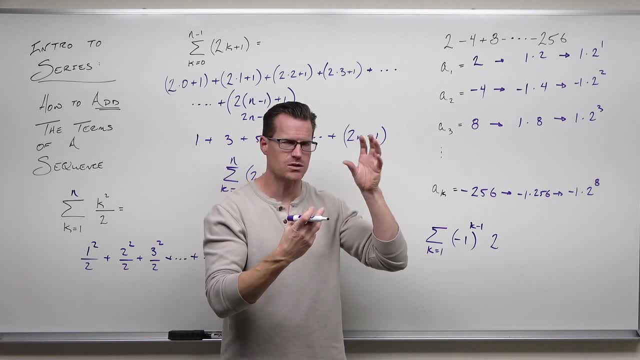 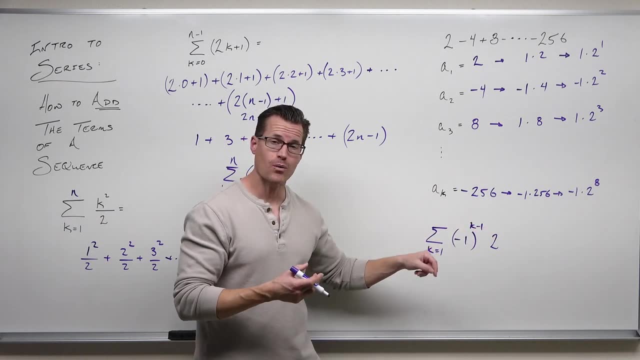 And so we have to have a different index. We can't use n and then plug in n to the n and represent a different n. That doesn't make any sense. So you start at k and you go: okay, k is my index. That way I can plug in one and two and three and four and five and six and seven and eight. 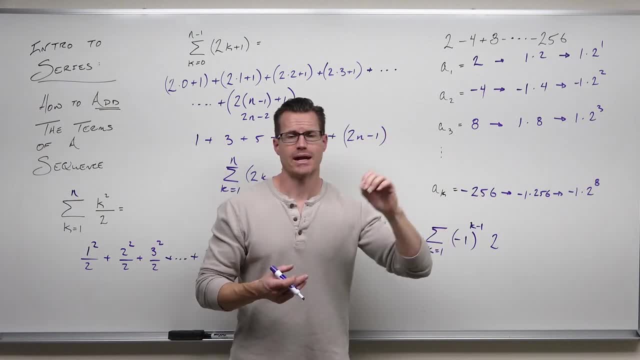 and end at my n. I can plug in my n and get my n. So I can plug in my n and get my n and get my n. I can plug in n later and it actually makes sense. I just need like this dummy index and 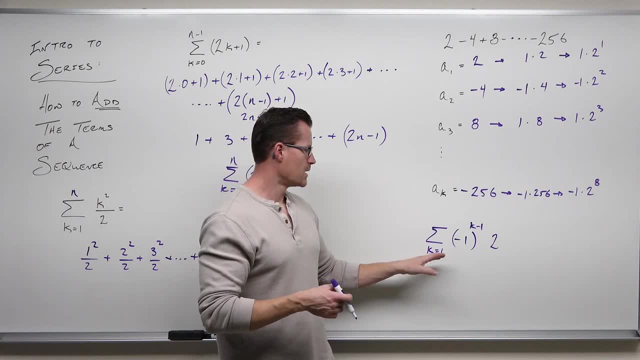 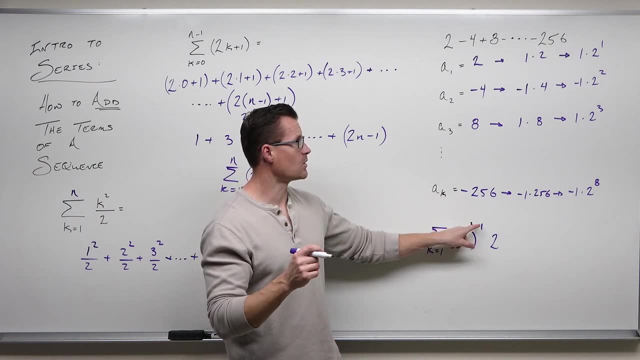 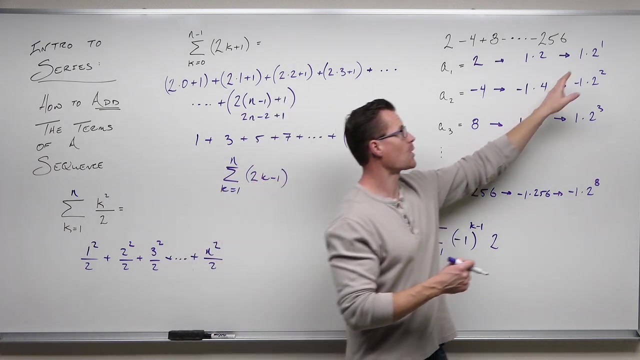 call it k. Hopefully you're okay with that. So plug it in one. Let's just double check this. Negative one to the one minus one. One minus one is zero. Negative one to the zero is one. That works. Two. I have a two in every single one of those terms. And now we relate the other part. 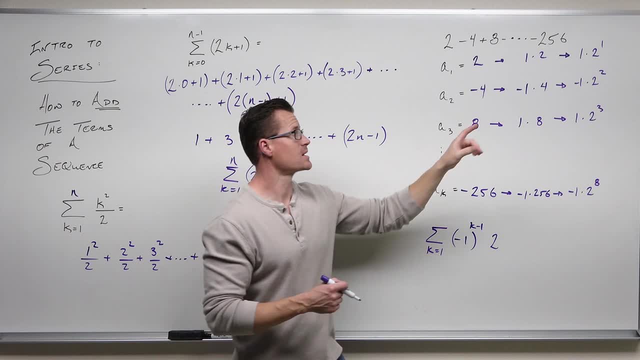 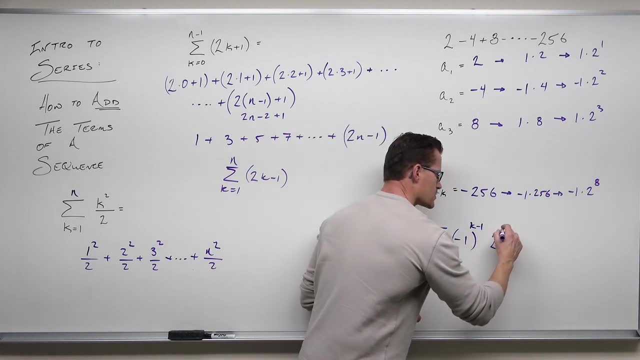 that's changing One, two, three, eight. Back to my index. It appears that one and one, two and two, three and three, This is matching, And so this is going to match my index. Again, it's k, It's not n. You can't do. 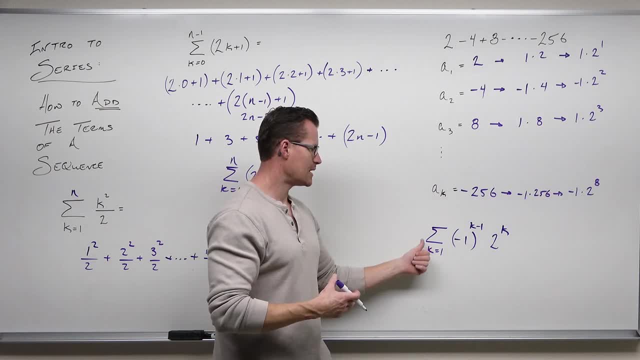 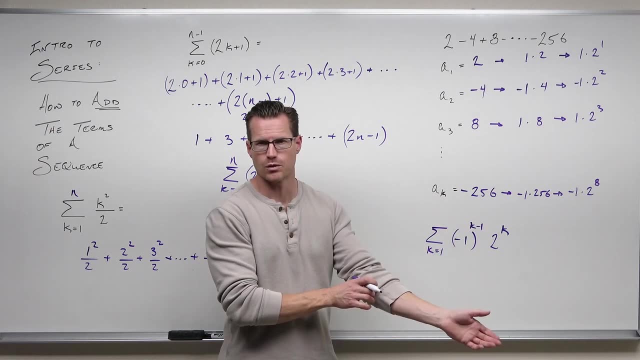 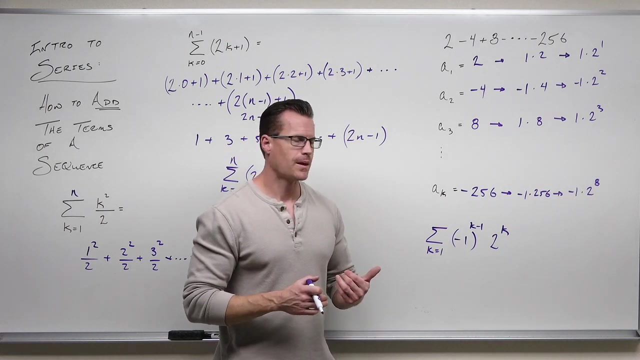 that because you're going to end with an n, You can't say that n equals one, and then two, and then three and then end at n. It's not correct form. You'd have too many n's floating in here. You use a different index. We call it k. Now the last thing. how do you know when you end? Because all 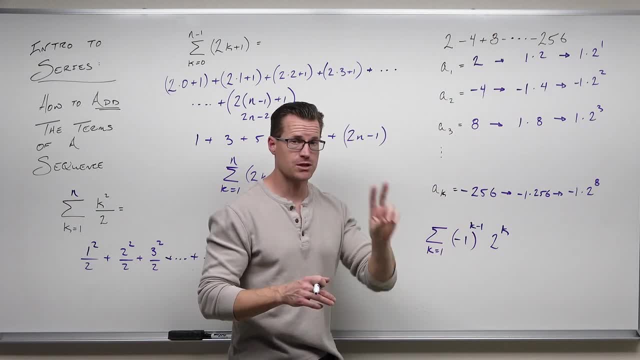 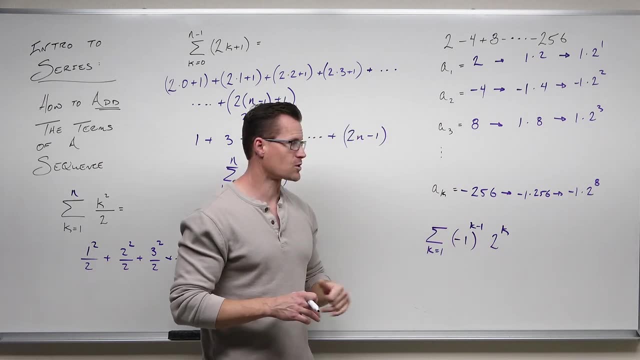 of this stuff. you could have just had this and got this. So I'm going to say two things. Number one: if you were not given this last term- let's pretend that wasn't there- If you weren't given that last term and you didn't have this information, you would just put n and you would 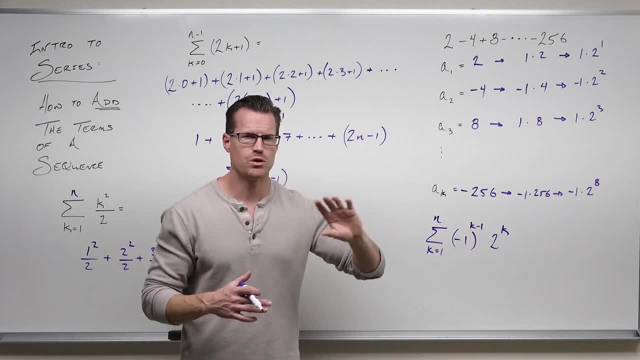 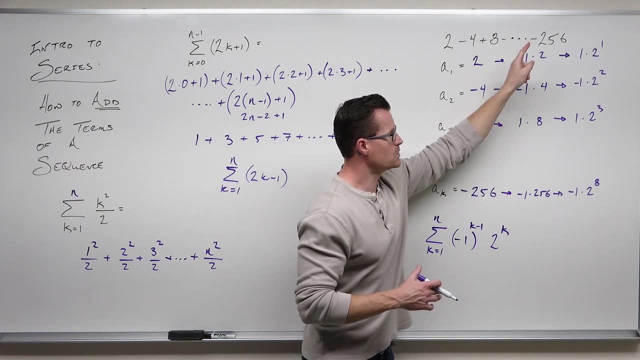 be done because you would be able to represent that series And you would say it has no end to it. So this, this and this, that would give you one negative one, one. two to the first, second, third, You'd have negative one to the k minus one that matches our signs. Two to the first. 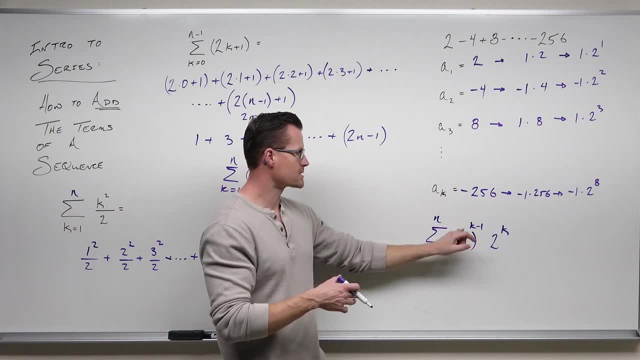 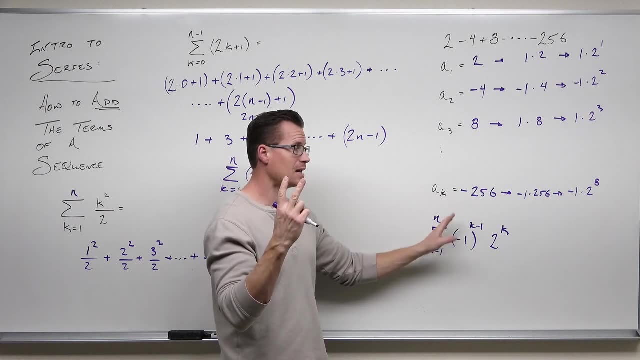 second third, that matches our index. The first term would give us positive two to the first. That's what we got. Second term: we plug in two. I'd get two minus one. That's negative. negative one. two to the second, That's what we have The next term. 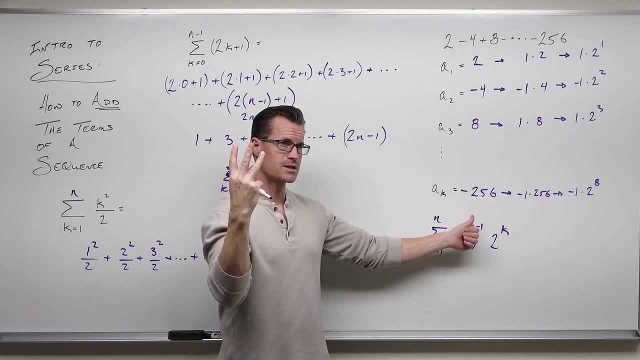 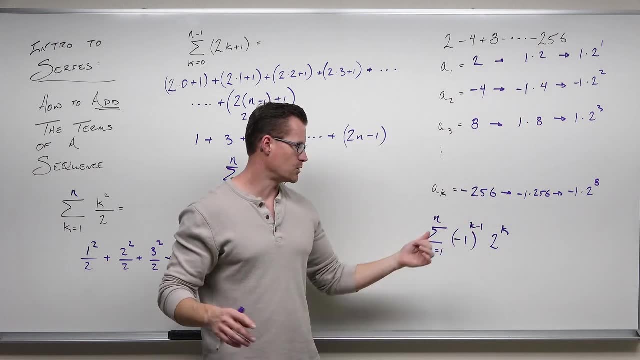 if I plugged in three, I would get three minus one, that's two Negative. one to the second is positive, one, two to the third. That's exactly what we have And we say: if we were not given an end, you put an end there And that end says you go forever until you reach an end. 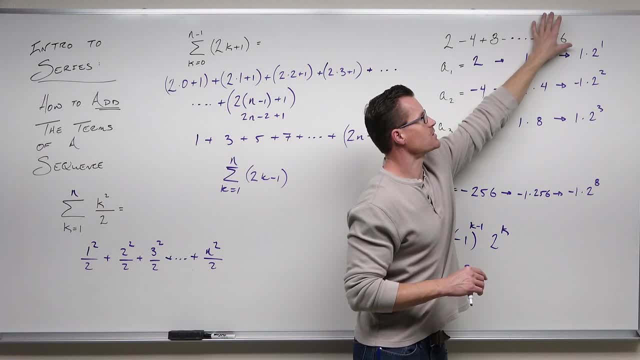 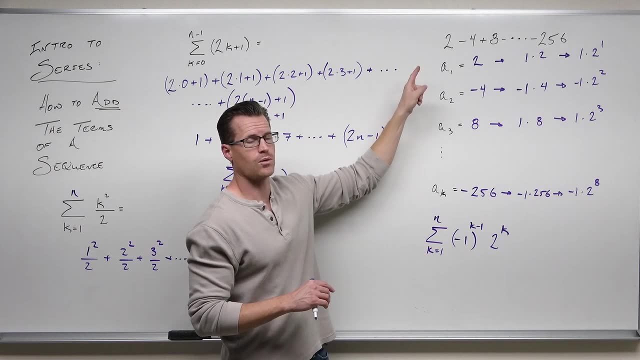 Do you see how you could write? Remember? you could write the same series that we have here And your ending term would be: let's see two negative four, eight, then negative 16, then blah, blah, blah, blah, blah, blah, And you would. 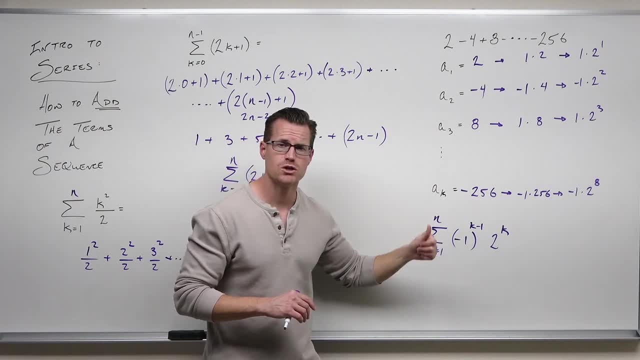 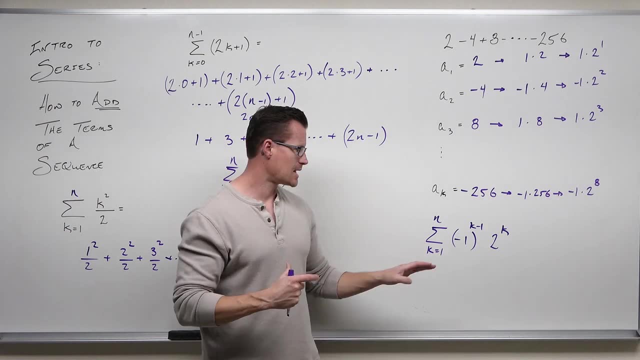 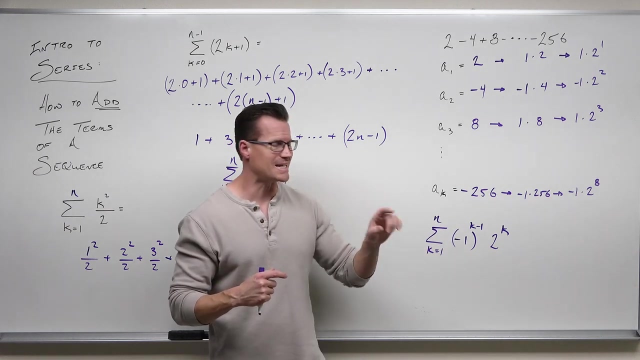 plug in n And you get negative one n minus one. two to the n. That would be your nth term, That'd be your general term. That's why we use two different letters: k for your series and the sequence that the series is based on, and then n to represent your nth term, Because you need a. 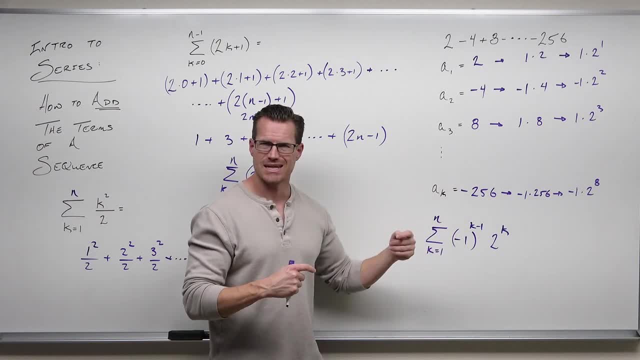 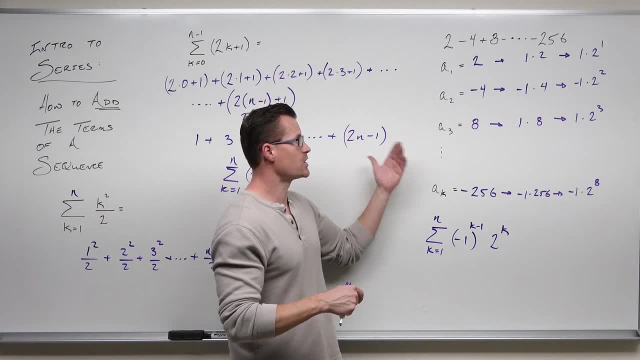 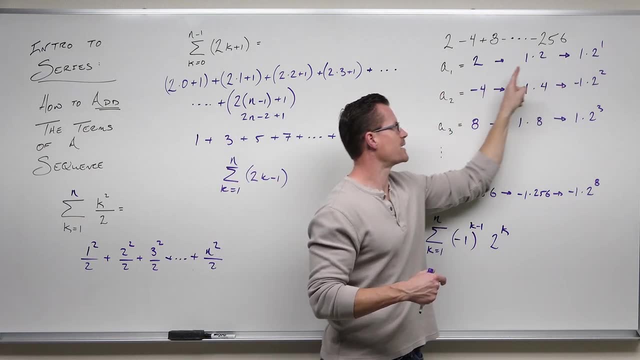 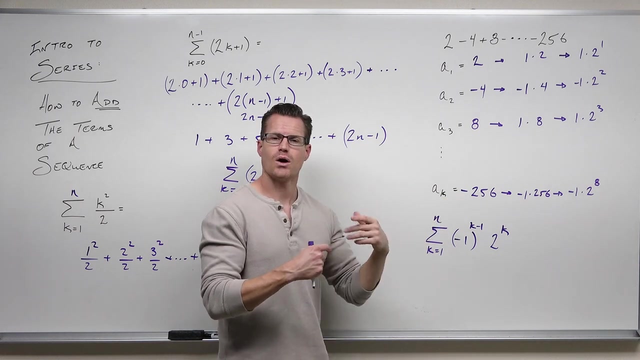 ambiguous. Now we don't. we don't have a general term, We have an end. So what's very nice about this is because, because our index matches our power index matches power index matches power index has to match that power. It's got to be an eight And it says: oh okay, this has to be an. 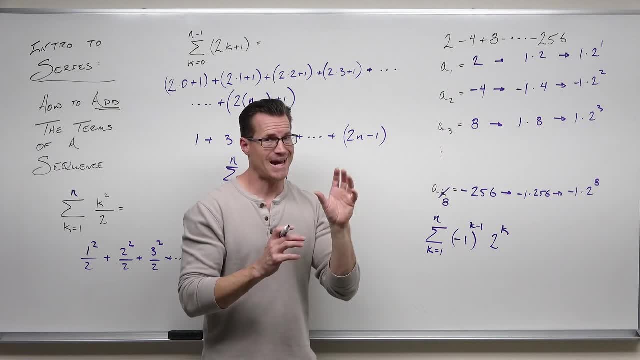 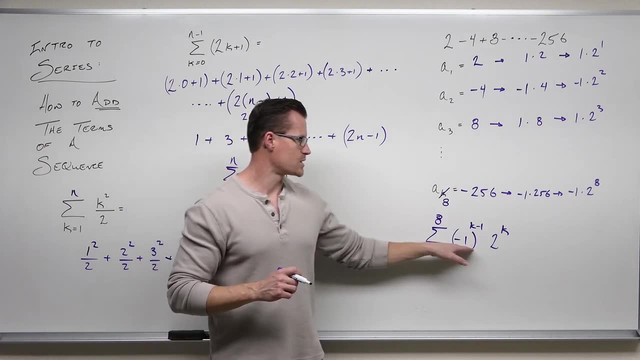 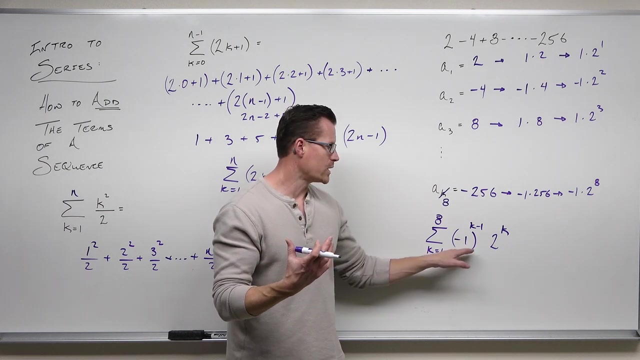 eight, And if it's an eight then you know that's the eighth term. If you know that's the eighth term and it's the last term, you've just found where you end. This series is represented as: here's the sequence. We know it's right. We've just spent like an hour long video finding sequences. We. 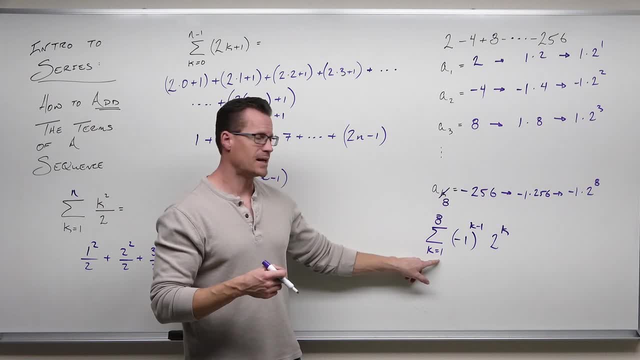 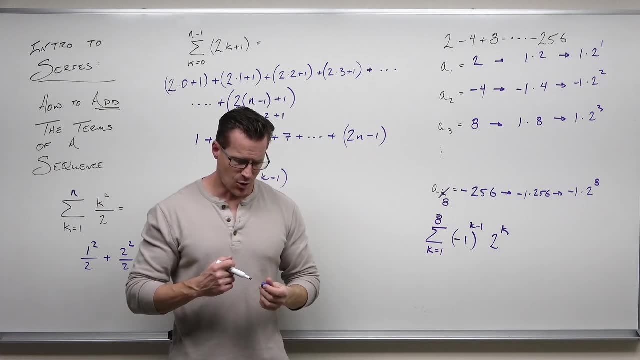 know that that's represents a sequence. We know it starts at one and now we know it ends at eight. That is the eighth term And this is how you would represent that series in series notation. Hope that makes sense. Hope you're seeing the relationship between the. 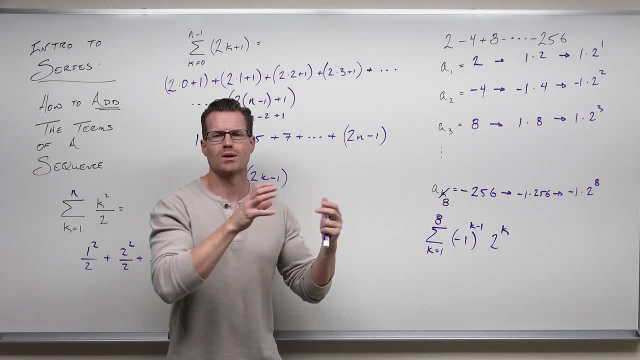 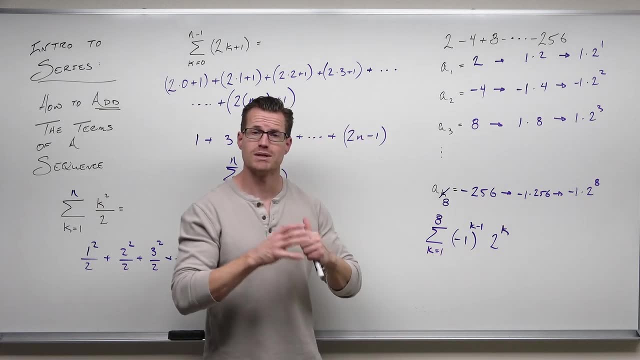 sequences that we already talked about. Now we're just kind of relating it back to the sum and showing that a little better with some different letters. Again, we need those different letters because you need an N to be able to plug into something And we need to end with an Nth. 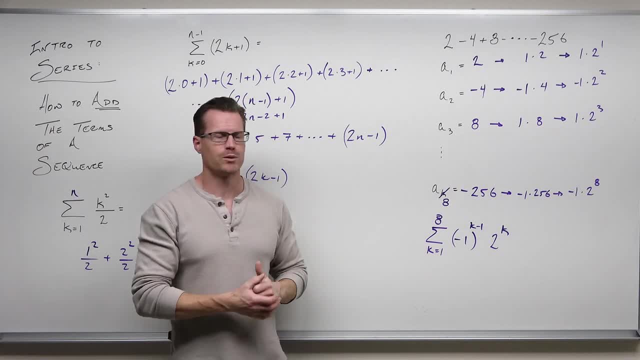 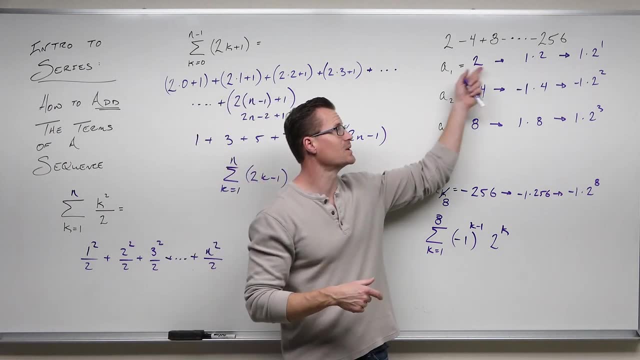 term, a general term in terms of N. So we need a different variable to base our sequence on. That's the only reason. What we're going to do now is I'm going to show you the formulas for how to add series, because we don't want to be doing this with a calculator or something. I'll show you that. 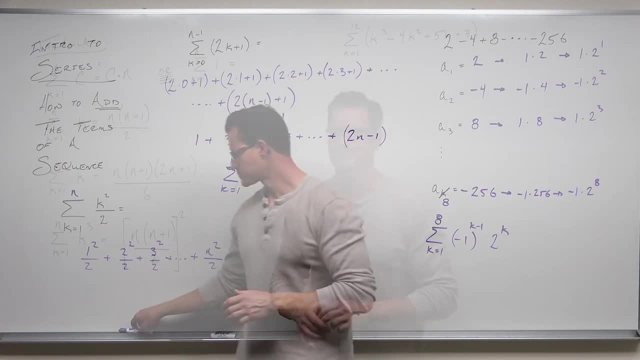 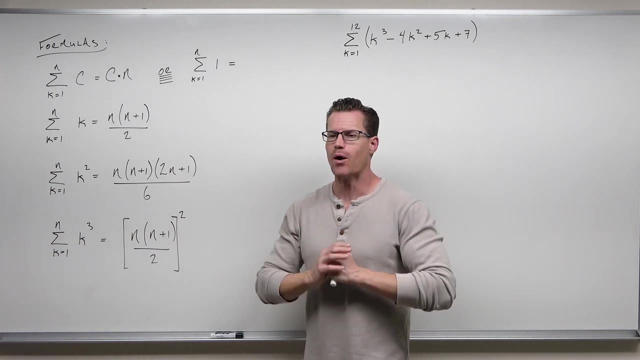 and then what we'll do. Let's practice a couple, Okay. so how do we actually calculate the sum of these series? We don't want to actually write it all out and do it, because that'd be crazy. I want you to imagine. 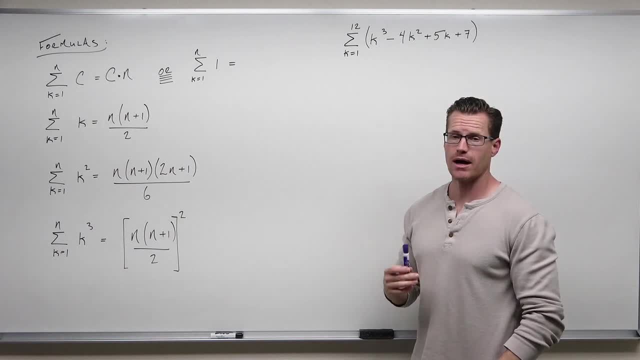 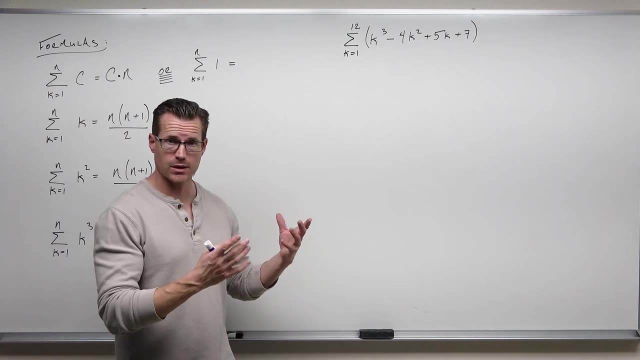 something, because we're going to do this problem and you're going to find out that it's not as bad as it looks right now. This looks horrifying. Why? Because if you had to actually add that series, what would you do? Well, let's look at it. This series means sum of what, This sequence, It is a. 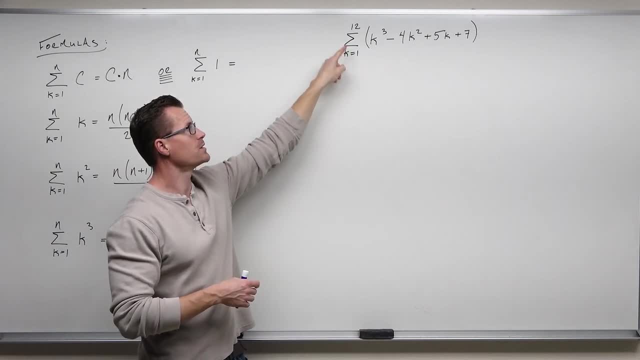 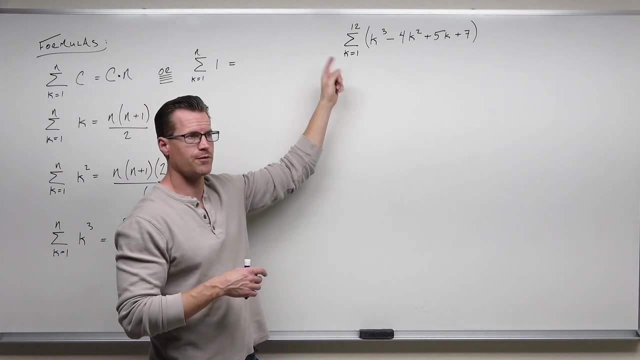 sequence. It's based on an index K of 1 to 12.. So you do this. You plug in 1, figure it out. Plug in 2, figure it out. Plug in 3, figure it out. Plug in 4,, 5,, 6,, 7,, 8,, 9,, 10,, 11,, 12, all 12 terms. You. 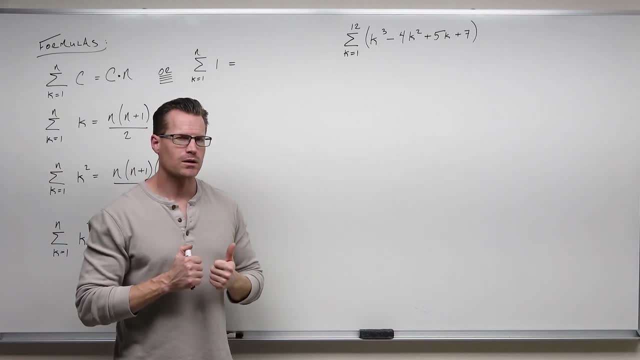 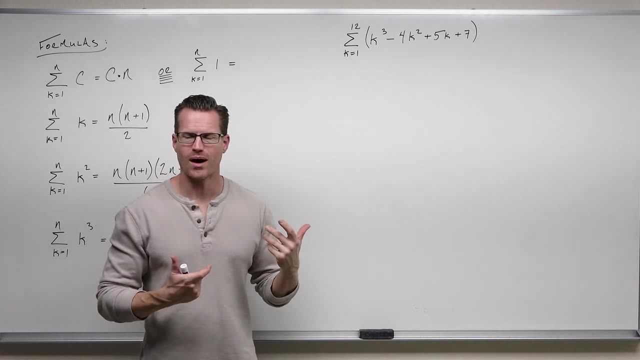 figure that out. and then you add that That's a lot of work and we're going to do something. that's still a lot of work, but quicker work Also, hopefully you can tell I kind of enjoy this stuff. I don't know why. It seems like some sort of a puzzle. I really enjoy it, Don't know. 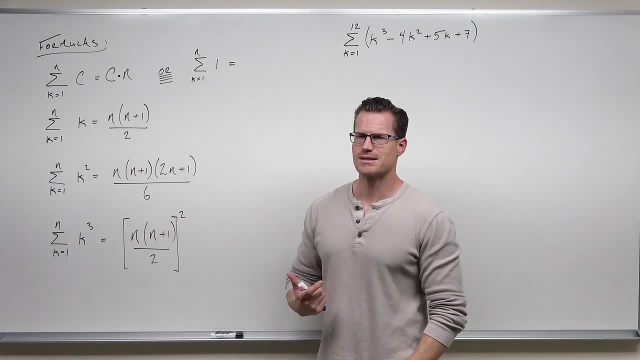 why that is. but this is one of my favorite things is the, the sequences in the series. I like the challenge in it. I suppose There are some formulas that are going to help us solve series: how to add the terms without having to actually add the terms. 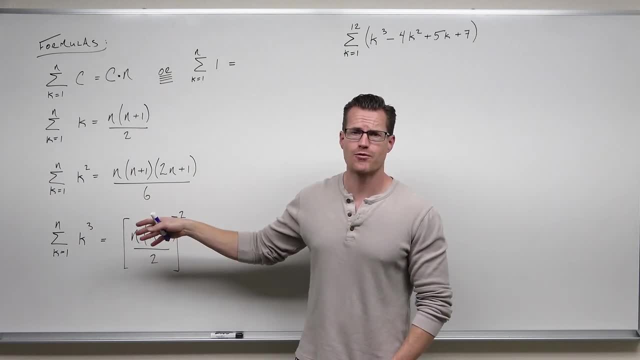 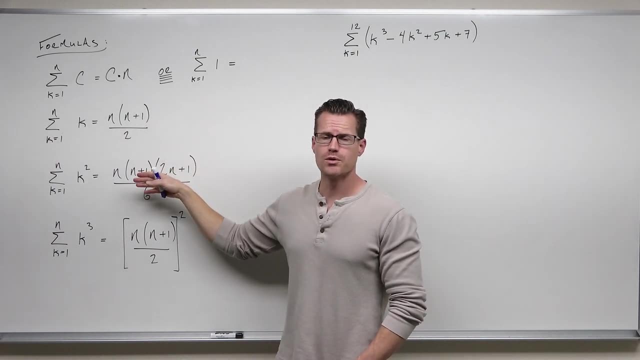 Now you're going to ask the question: where in the world does this stuff come from? One of them is very common sense and needs no proof. Same thing as that one. but the rest of them would require proof. We prove most of these by induction. 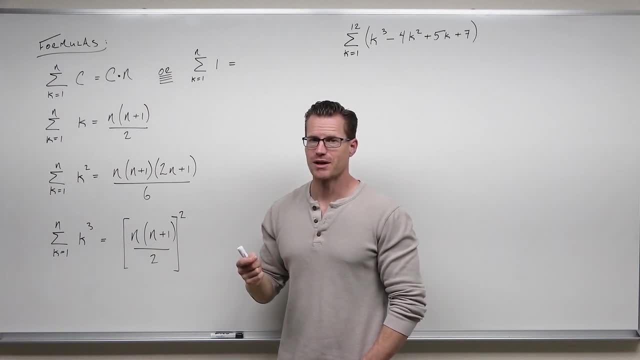 If you want to know where they came from originally, you could ask someone like Carl Frederick Gauss- Well, you can't because he's dead, but if you could. he solved that by himself in like fifth grade or the level of fifth grade, which is insane. He did it in like I don't know. 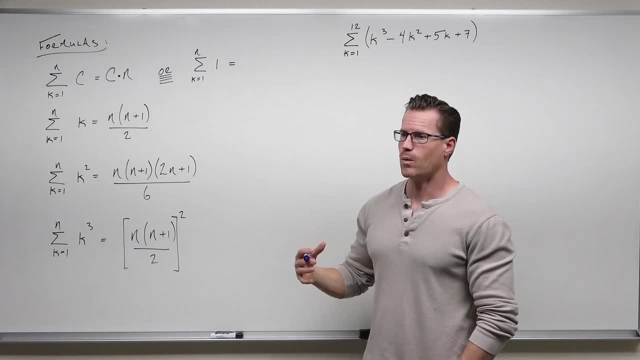 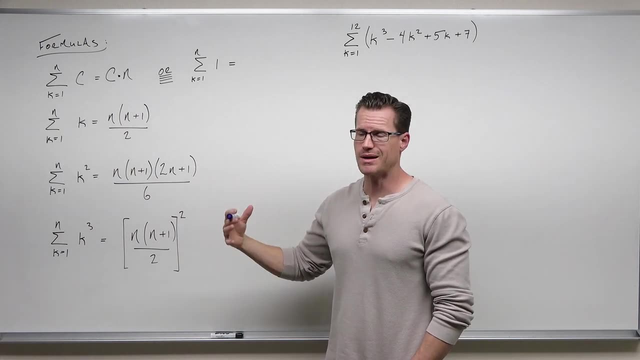 a couple of minutes because he was super genius. But anyhow, a lot of these were discovered by pattern and then proved with with induction, And so I will show you how to do that. There's other ways to prove it, but I'll show you how to do that in the last last video, in. 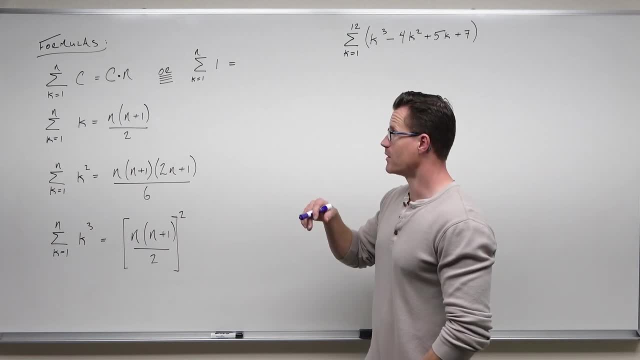 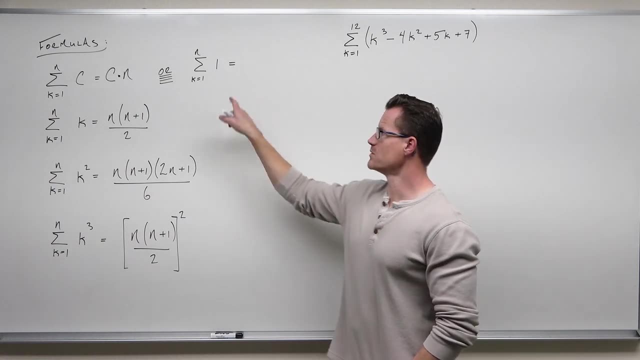 this little, little kind of sub series that we have on on sequences. So here's what this means. Here's what the formulas look like, Cause at first they look a little confusing, I'm going to do this one last. actually, even though it's the most basic one, I'm going to do this one. 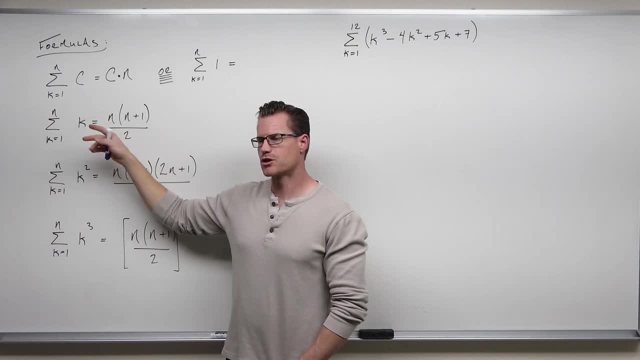 So how, how you can add up the terms of a series without actually doing the addition is with a formula like this: Now I want you to understand how this works. This says: let's suppose that your sequence is based on just K to me. 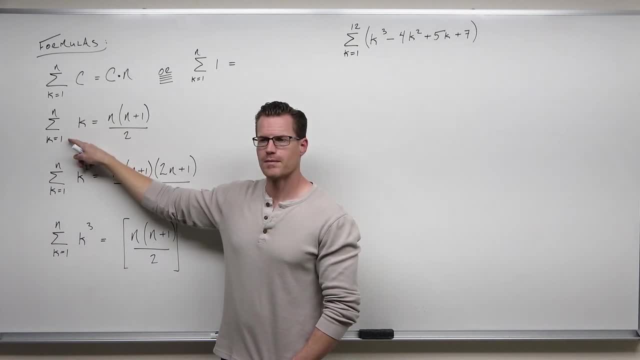 That means that you plug in one, two, three, four, five, six, seven, eight, nine and 10, and that would be the terms of your sequence: One plus two plus three, plus four plus five. If you add it up, we create a series. You stop at N. So if this was 10, here's what this would mean. 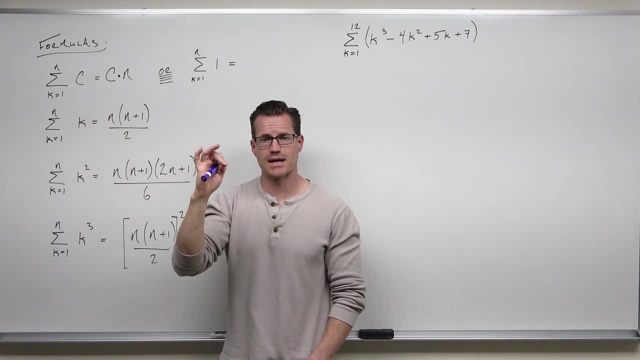 This series would be at one, two, three, four, five, six, seven, eight, nine and 10.. That's what that would be. Now, you can do that pretty quickly on a calculator, but this is actually even quicker than that. 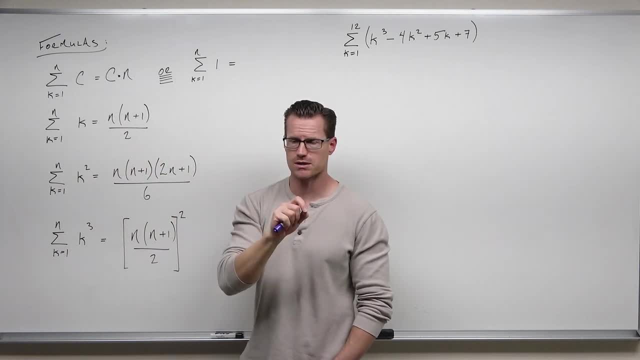 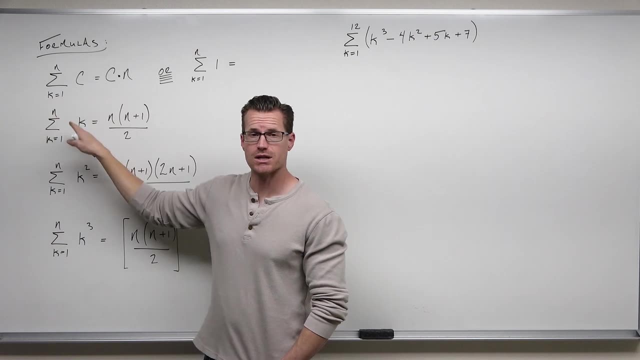 Here's all you need to know in order to find the series. find some of that series quickly, just know where you end. This is the second Reason why we need different letters here is so that you understand that this is based on the end of this series. 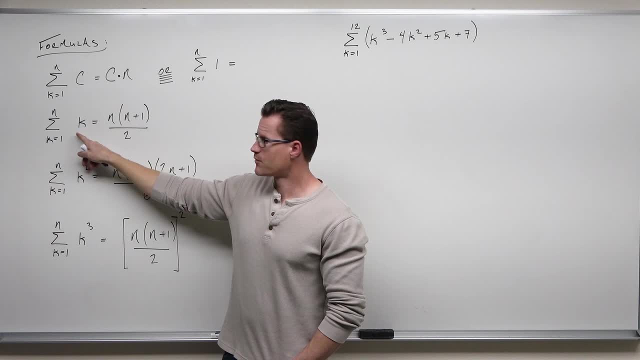 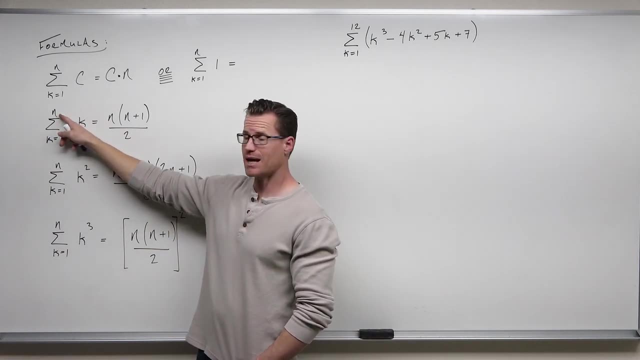 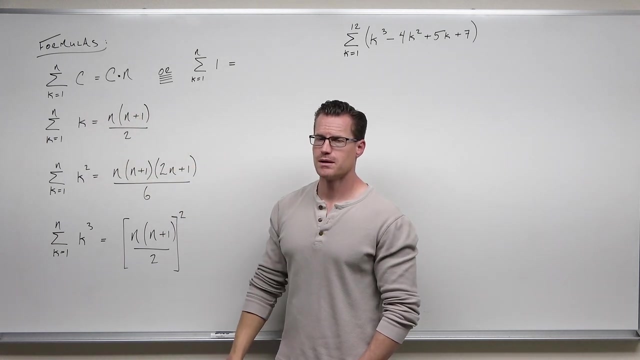 So if I'm adding the series of the sequence K from one to N, I just take my N, I plug it in here and it's going to give me the sum. So if I go from one to 10 and I know it's based on K, then I just plug in 10, 10 times 11 over two, 10 times 11 over two is 55. 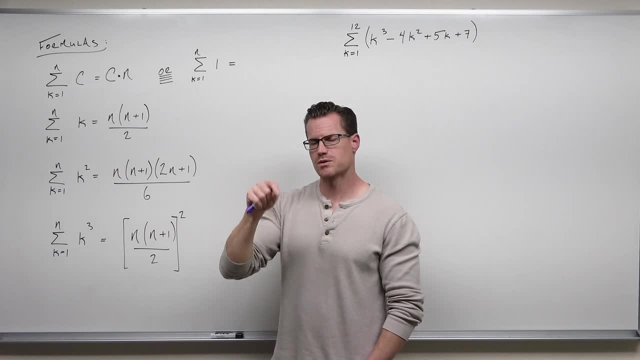 That's going to add to 55. I need to take it out of there right now. Do one plus two plus three plus four, all the way to 10, it's going to be 55. Why? Because this actually works and it's provable. 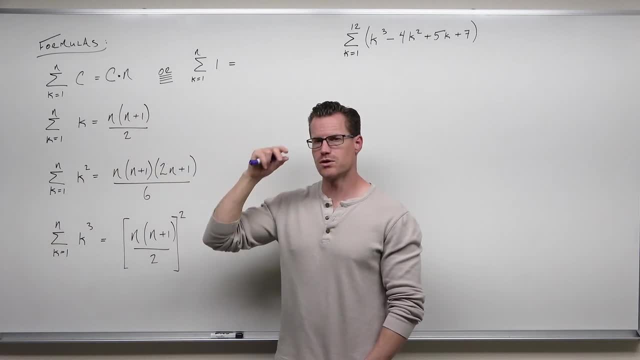 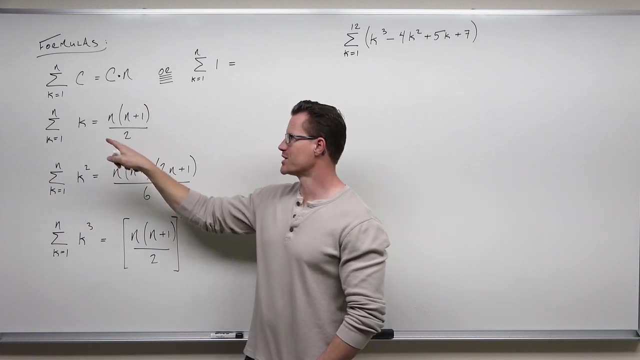 I'm not proving them now because I haven't taught you induction, but I will prove that one to you at a different time. Now there's some other ones. Why are there other ones? Because not everything can be simplified to just having a sequence of K. 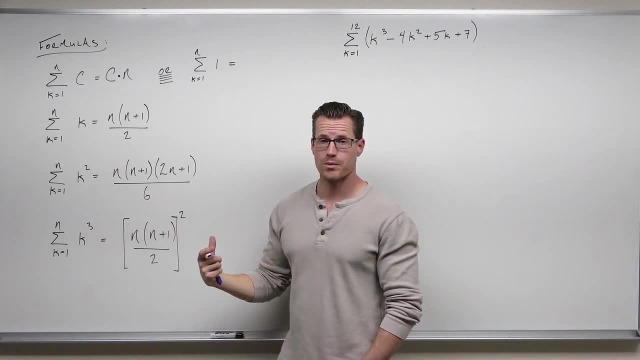 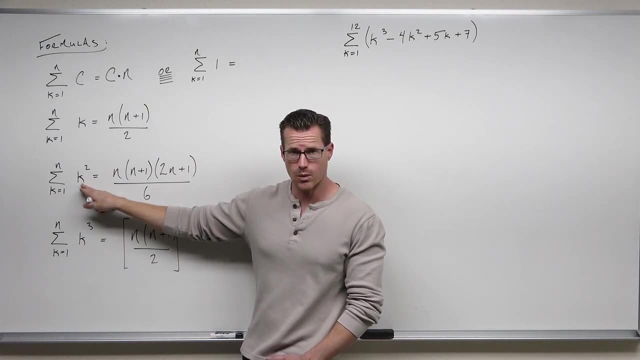 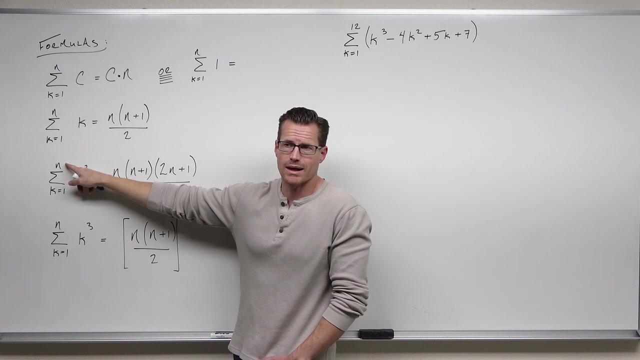 What about K squared and K cubed? We have two other formulas for that. Now. there are other ones out there, but these are the most common ones. So what if you had a sequence based on K squared? Well, what you would need to know is that you're starting at one and that you're ending at whatever, like 10 or 12 or whatever that number is, because if we have that, there's a formula to add it. 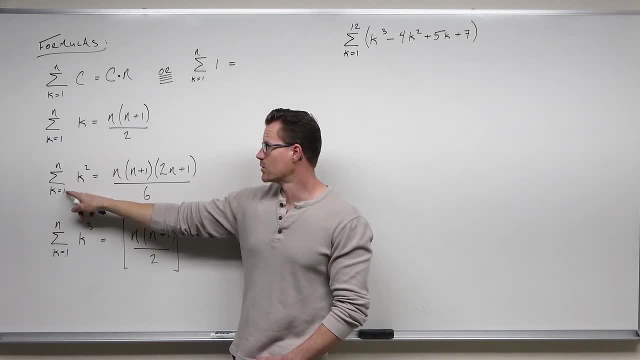 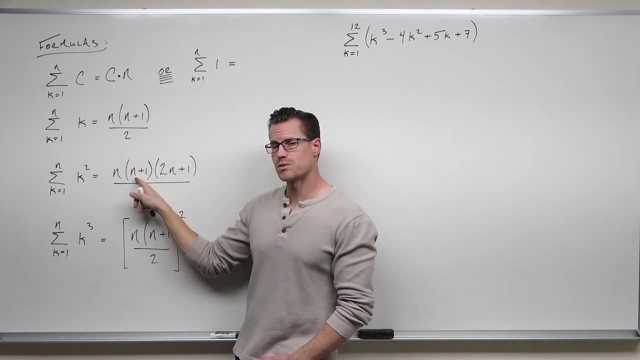 So if we were ending at, let's say, seven or something, so we knew the sequence was K squared. We're starting at one, we're ending at seven. Take your ending number seven. seven plus one is eight, seven times two plus one is 15,. seven times eight times 15, and then divide by six. 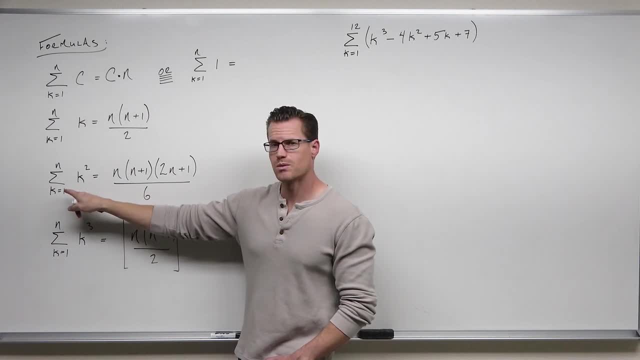 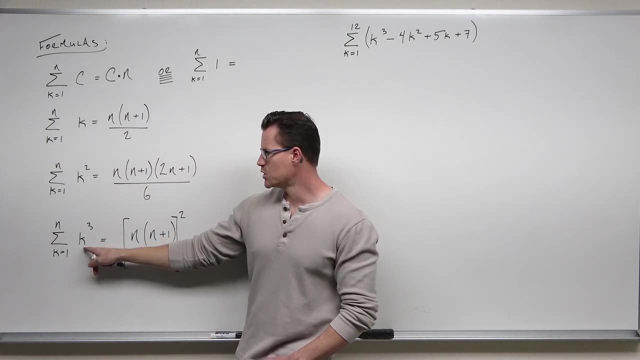 That will give you the sum of one squared, two squared, three squared, four squared, five squared, six squared and seven squared. all added up, It will do it for you. It's pretty fascinating. Same thing works here with K cubed. 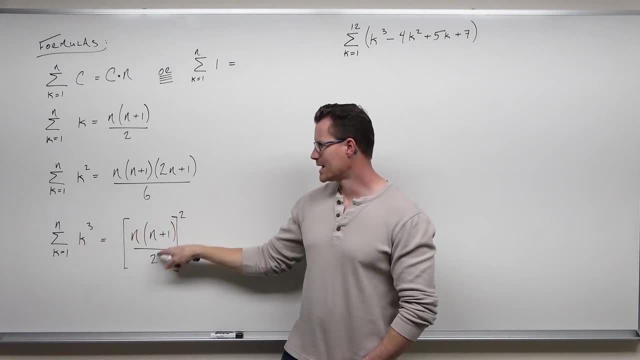 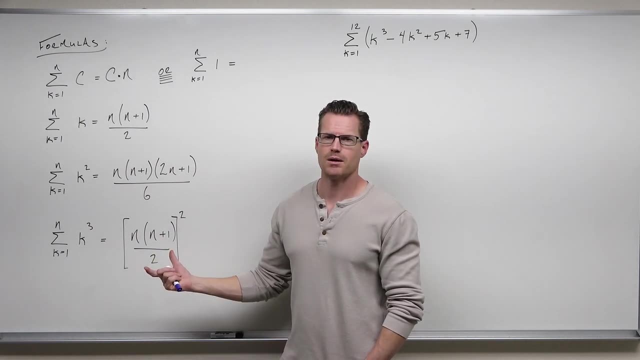 If you know where you end, take your ending number, plug it in and it will solve it for you. Now what if you don't know where you end? Then this is still relevant, but it won't give you a finite number. 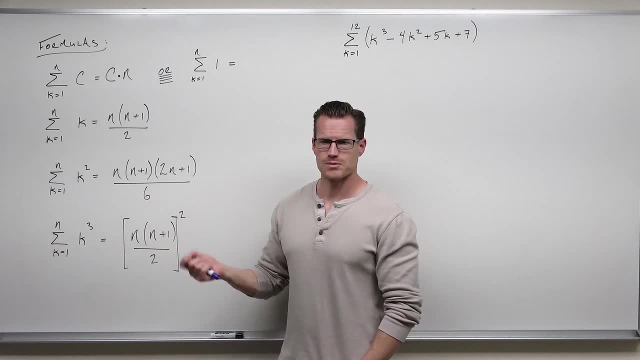 There are some infinite series that will, but they have special names, like geometric series, and there's special conditions, Like you have to have a ratio Of less than one common ratio. So there there are some special conditions. or between negative one one there's some special conditions there. 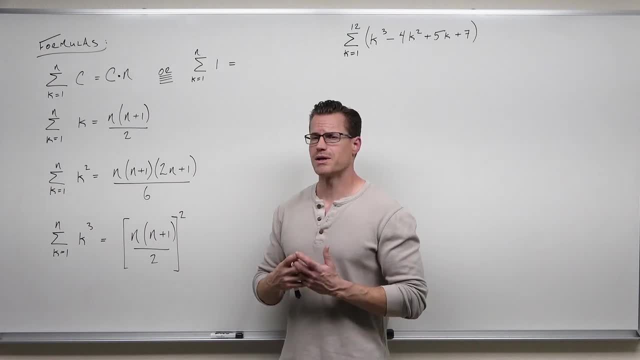 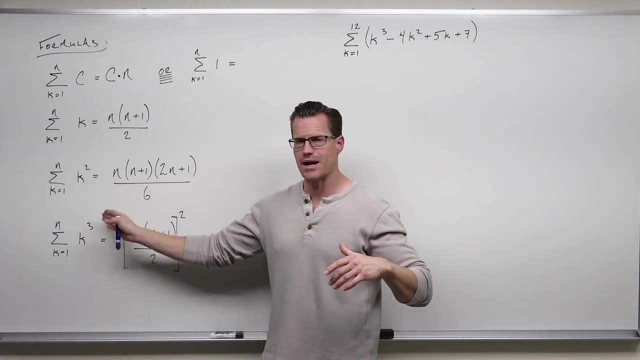 And there's some other series that have the same type of things going on. So, but in general, to add a series you need to know where you end, Otherwise it's going to go to infinity. Do you see that? Like if you just kept on adding this forever? and K was numbers one, two, three and four? it's going to go to infinity. 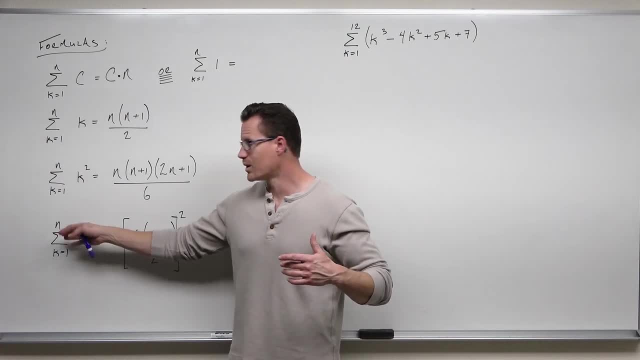 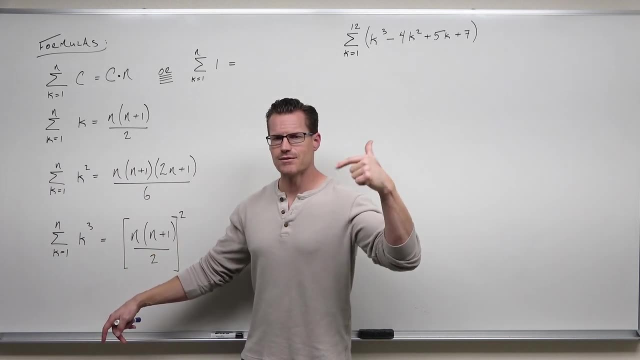 I it's going to be a really, really, really big, even going from like one to 12.. If this was one To 12.. So you add up one cube, two cube, three cube, four cube. That's already big. five, six, seven, eight, nine, 10,, 11,, 12, all cubed. 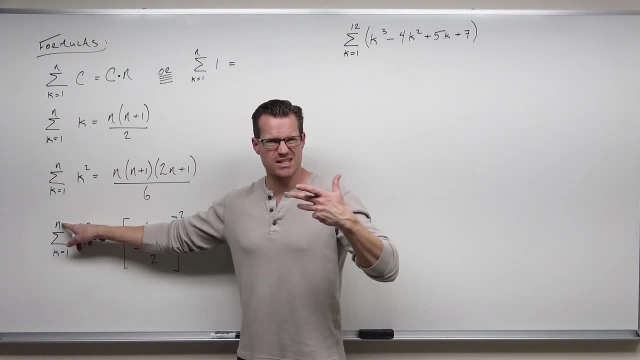 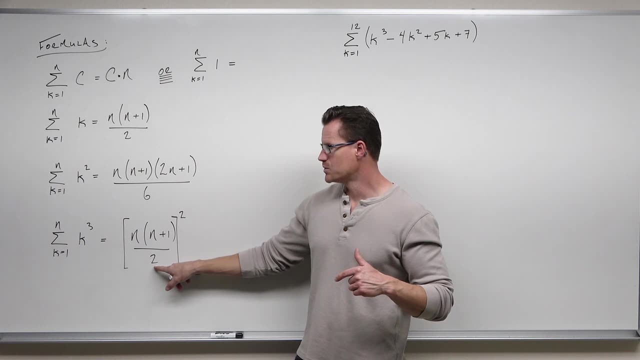 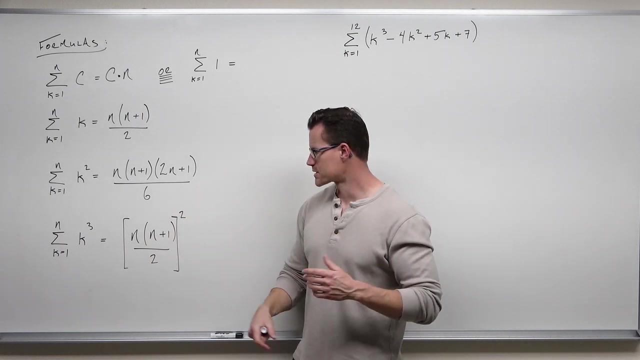 And you added them. We can do the same thing by taking the ending number, Let's say 12, 12 times 13, divided by two, 78 square, and then square that. whatever that is, Well, that's going to be pretty big. 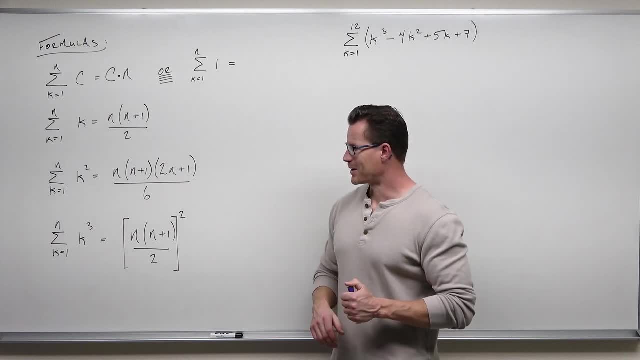 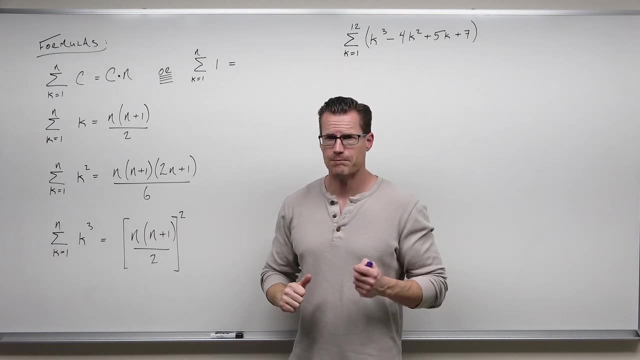 I can't do that in my head. I was trying, but that's a little outside my range. So this is what the formula is doing, how they work. They'll add the terms of your series very quickly, Very cool. Now let's look at this one. 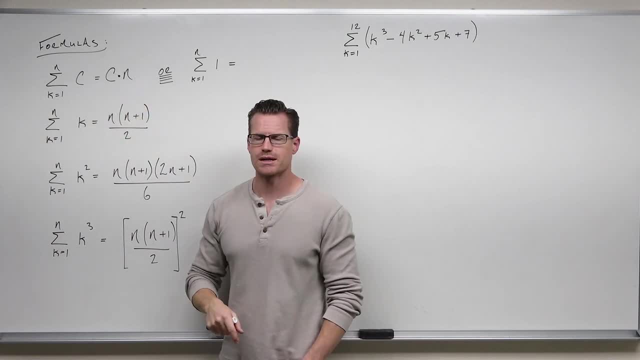 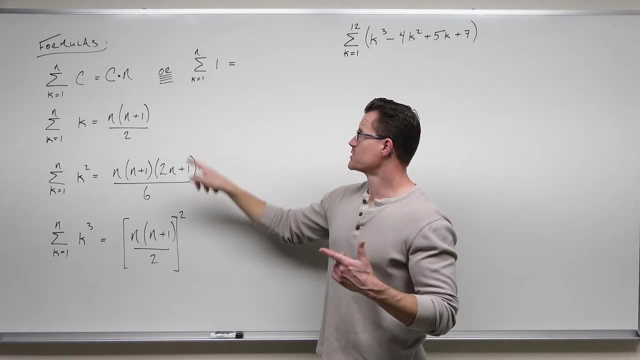 Cause this one confuses a lot of people. We go: how do you get the end? Where in the world is that coming from? I want you to think about it this way first and then see that that makes sense. So one thing that we can do is we can say: if you have a constant in there, nothing would change. 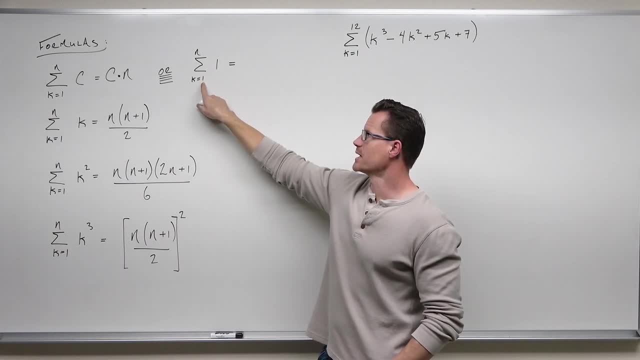 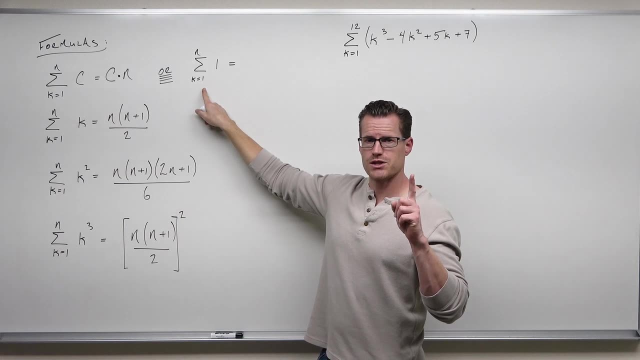 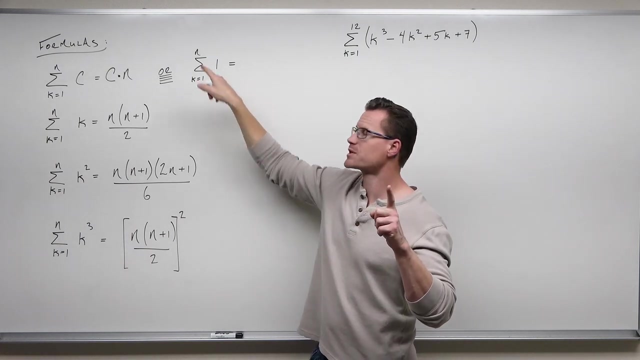 There's no K in there. So what this would This would be. this would say: plug in one. I can't, there's nothing to plug into. So what that would do is say: for the first term, take one. for the second term, take one. for the third term, take one. for the fourth term, take one for the fifth term, take one for the all the terms of the edges, take one and add them up. 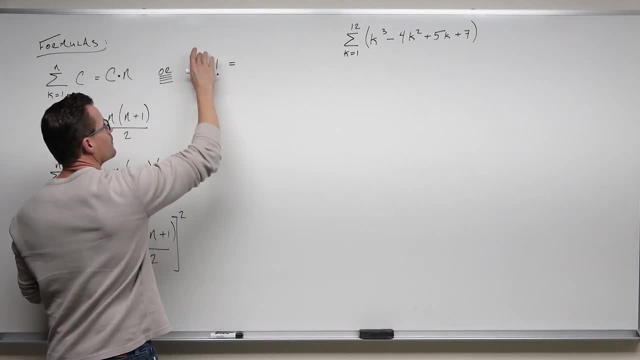 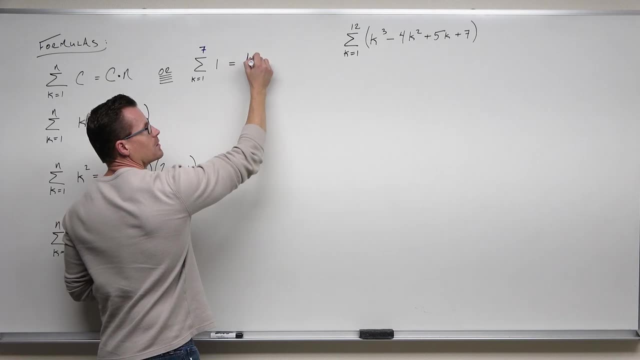 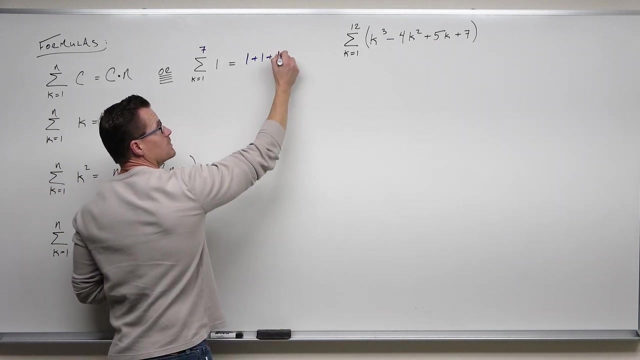 So if I went from one to seven of the sequence one, here's what it would do: It would take one, one, one. I wish I would have picked a smaller number than seven. the right seven ones: one, two, three, four, five, six, seven. 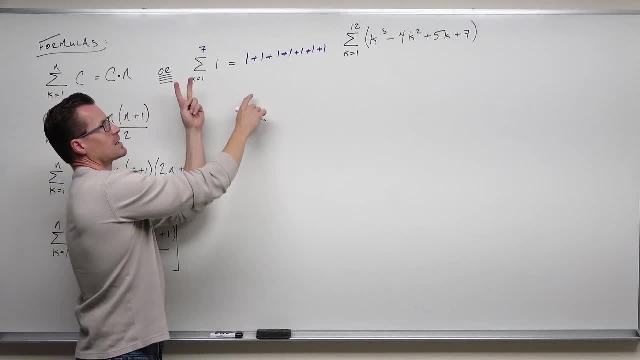 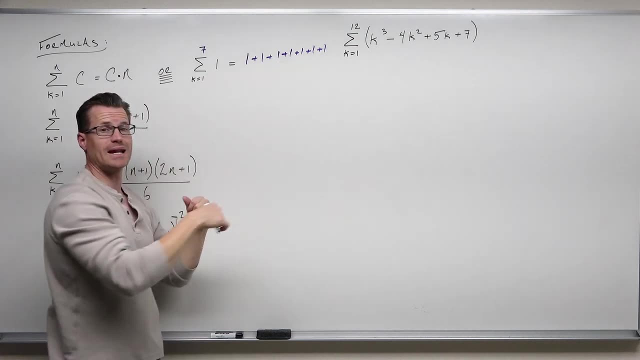 Here's the first term. It's one second term to one third term, one fourth term, one. you're getting it back. Fifth term, one six term, one, seven term one And then I end because it terminates. it says I end at seven, the seventh term, not plugging in seven. 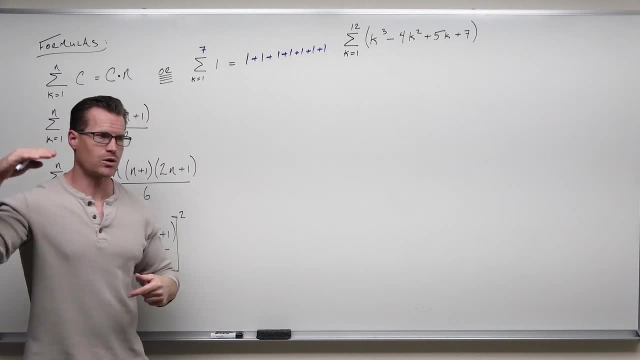 You're, you're, you're trying to, but it's only you're, it's only giving out one. It's a constant. What do constants do? They're the same value all the time. So one, one, one, one, one, one one. 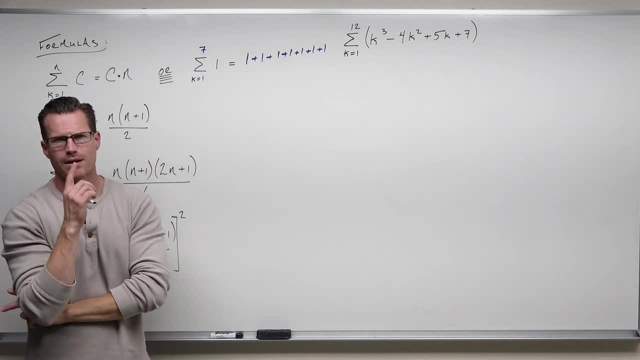 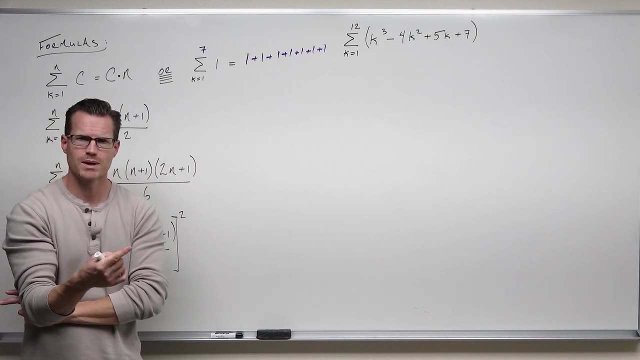 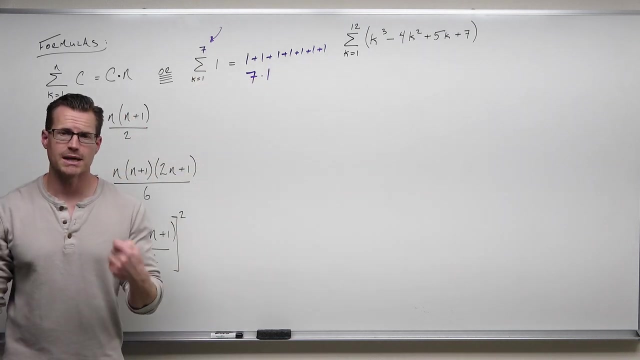 There's seven ones where you get when you add seven ones. wait a minute. That's repeated addition of the same number. Repeated addition is multiplication. How many times have you repeated it? Seven times, whatever is here, that value got repeated. 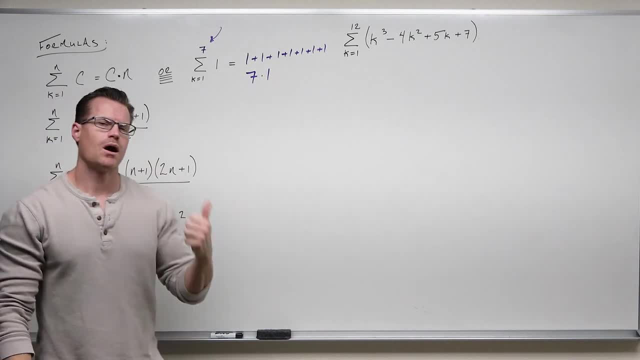 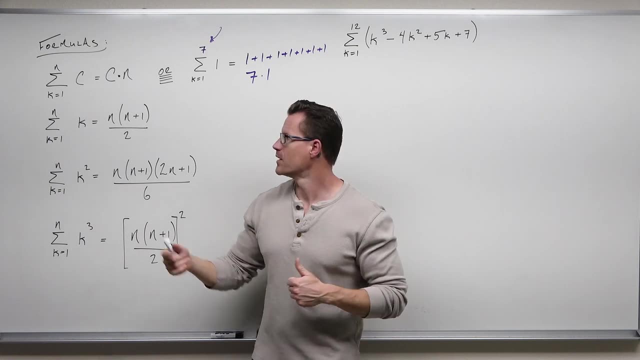 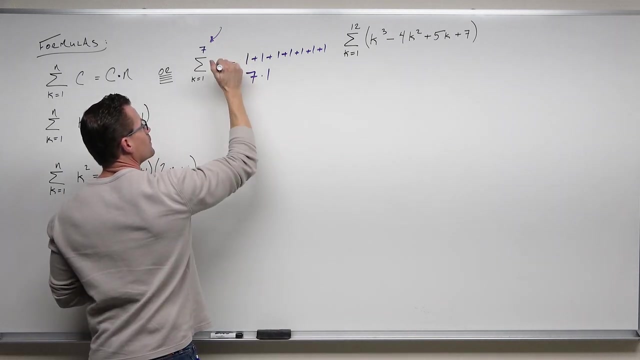 Okay, What would happen here? You'd have a constant. C would be a constant. There's nothing to plug into. the CC would be something like one, Or maybe five, let's say five. What would that be then? Well, if I went from one to seven of, let's say, five, now, these wouldn't be ones anymore. 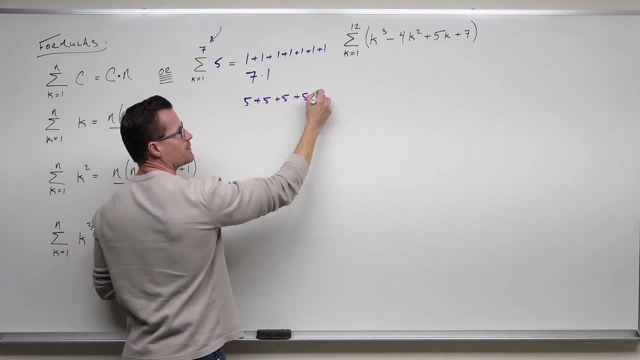 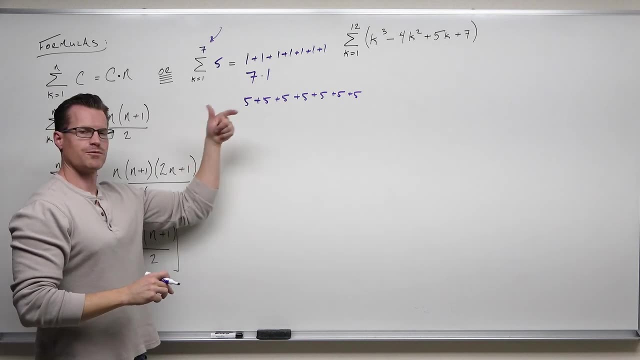 You'd have five, five, five, five, five, five and five, one, two, three, four, five, six, seven. The first term would give you a five, second term five. third term: five. 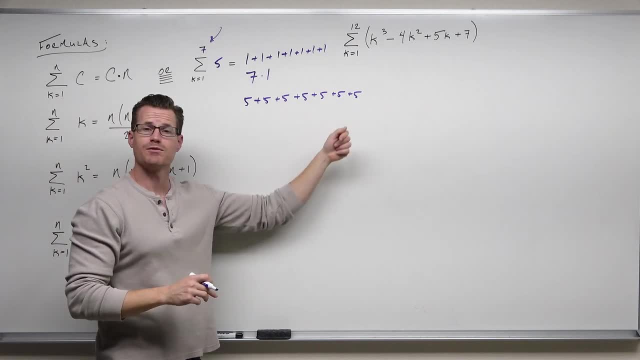 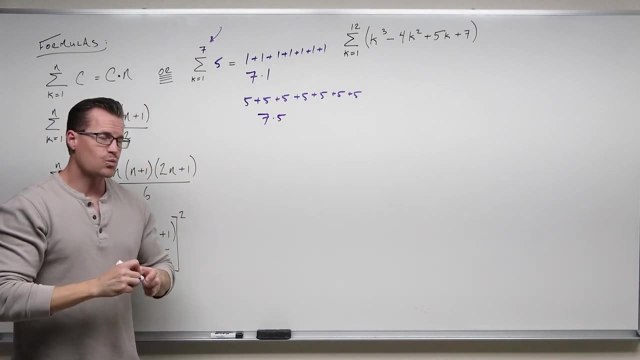 It's a constant. seventh term: five. Well, how many times have you added the five? Well, there's seven terms. Seven times five would be 35.. This is where that comes from. It says: take your constant, That's not changing. 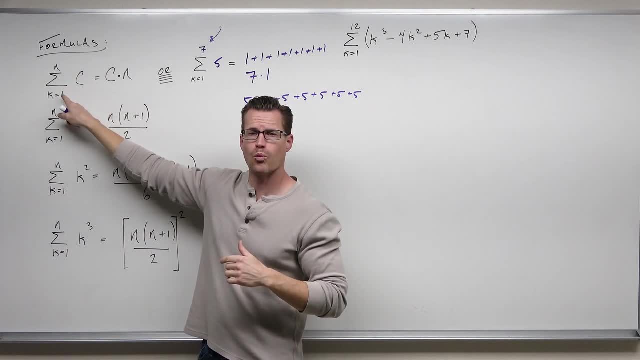 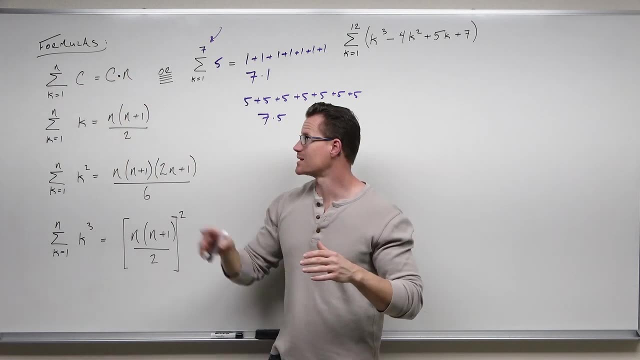 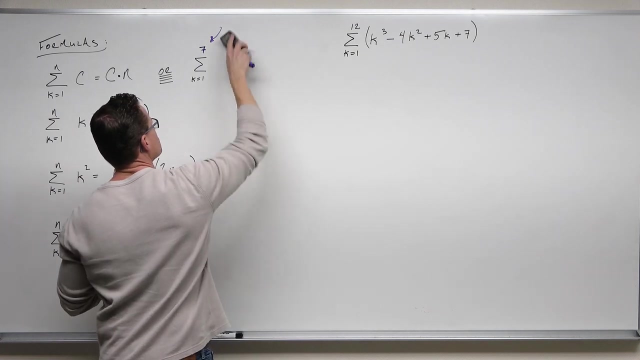 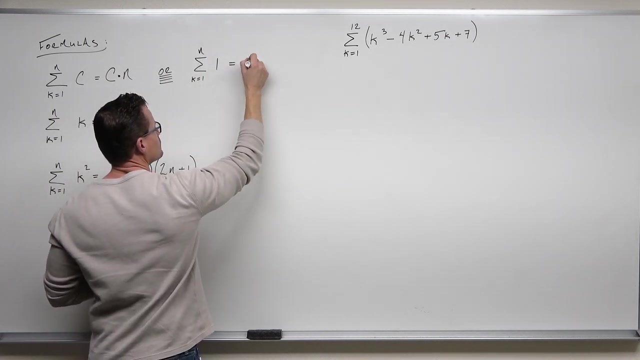 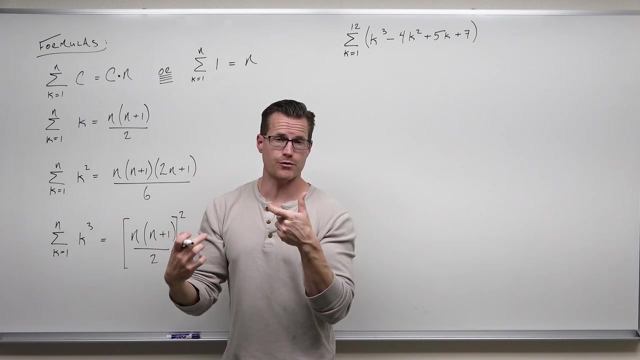 See how many times you haven't repeated. every time, from one to N, There will be N repetitions of that constant. The other way that you can view this- and this is why it says or is- is this: it's quite important: You can always take a constant being multiplied by something inside of your series and move it in front of the series. 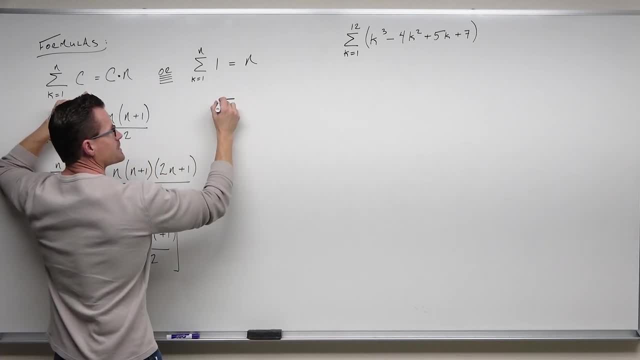 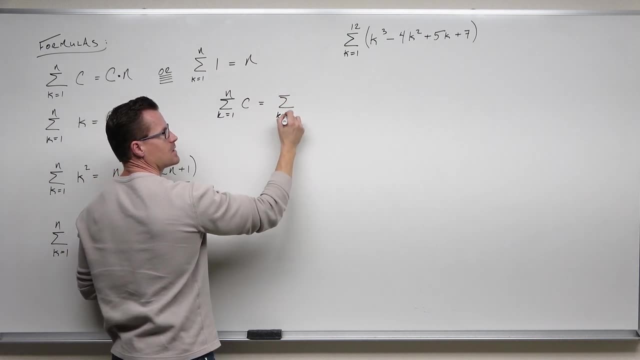 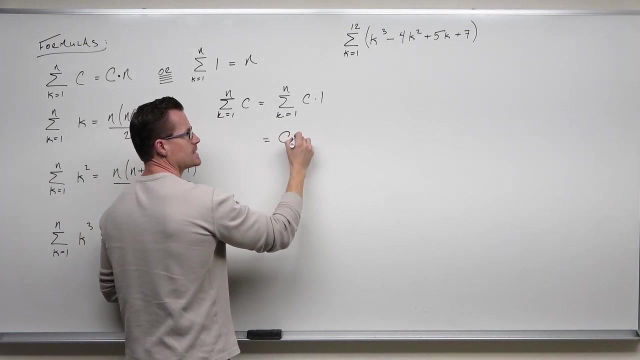 So you could do this. You could say this is the same as same thing, as K equals one to N of C times one, because C is a constant, I could make this C times the series of one to N of one. This would be C times. 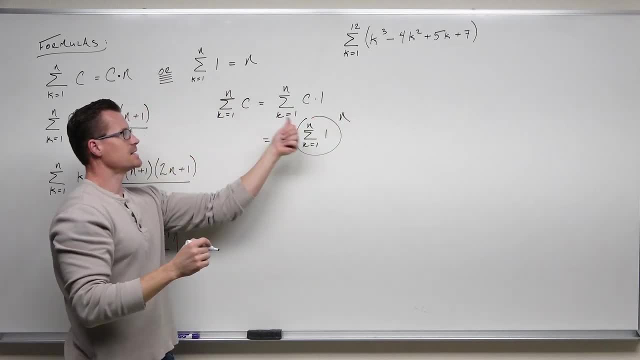 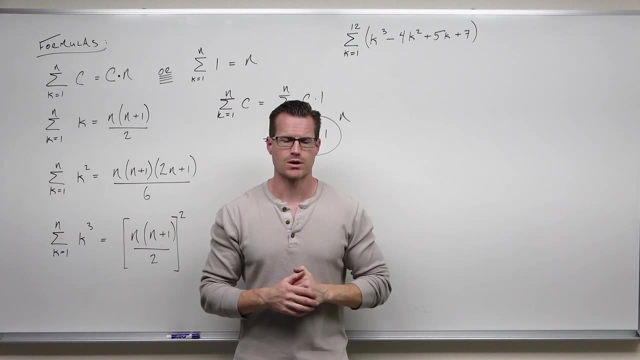 We already know that this piece is N C times N. that proves that to you. So we do get that out of it. We'll see that working through our our one example that we're going to get, because it might involve everything of every one of these formulas in that. 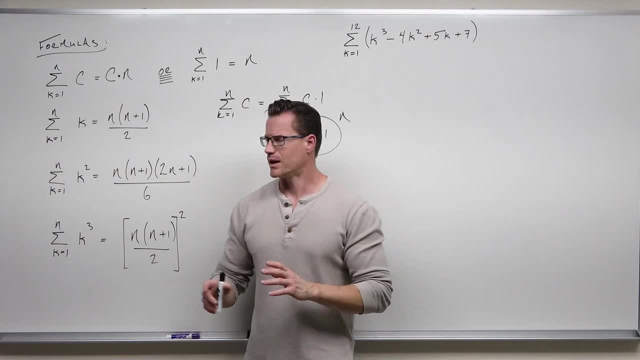 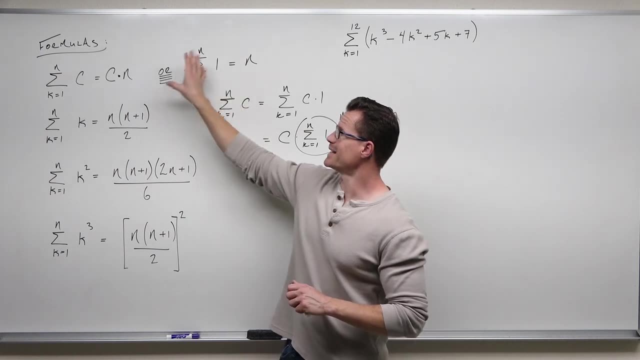 So we'll talk about what you can do when we get there. right now, I just need you to be really, really clear on these formulas. Actually, They're very relevant. We're going to use them in just a minute. This one makes sense, but you really have to think about it a little bit. 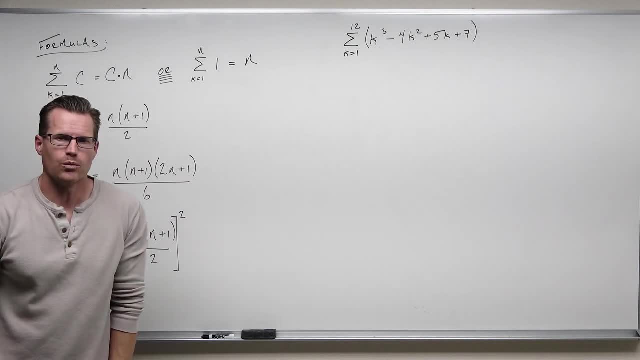 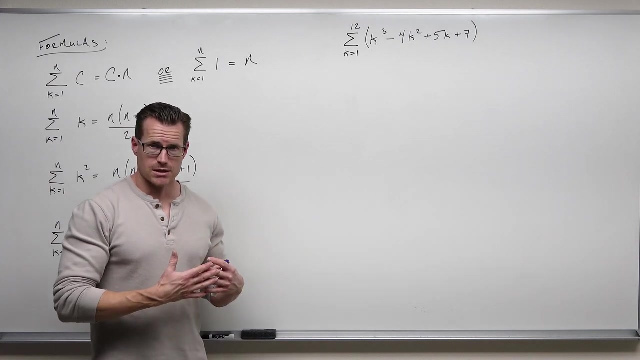 Okay. So back to our example. we don't really want to plug in one through 12 and add them up, because that's really annoying, And we have some formulas that do this for us. So the couple of things that I need you to know in order to be successful at solving that or adding up that series, finding the sum without writing it out- is that you can separate series by addition and subtraction and multiplication. 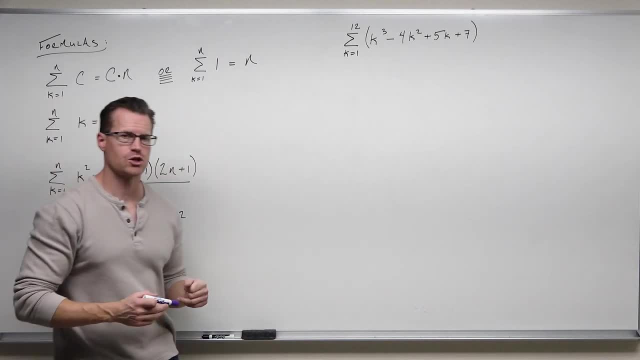 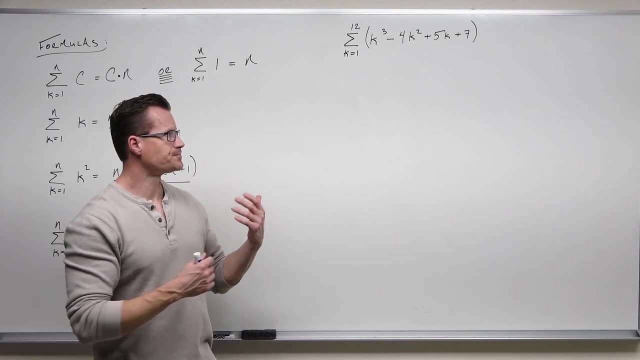 Now get why it worked on what I showed you. If a series means addition- adding stuff up- and addition is commutative, it doesn't matter the order in which you add stuff. It's also associative and separable, which means that I can add stuff separately and add it back together later. 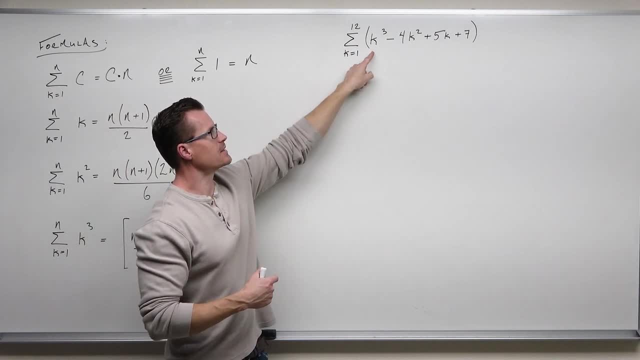 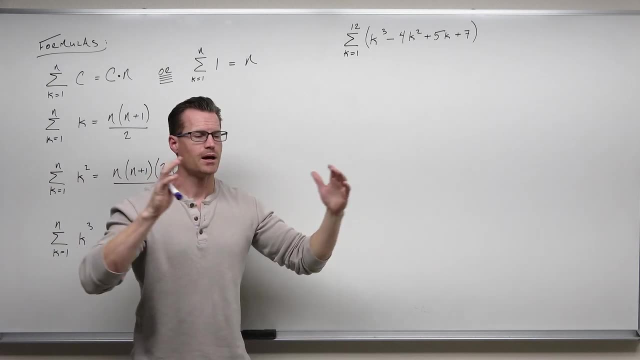 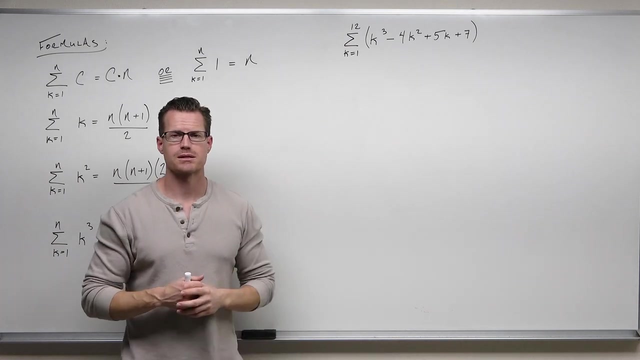 Okay, What? what does that mean? That means I can look at adding these things and these things and these things and these things, Separable and then, or associative grouping and then add it back together. So a long story made short is: I can separate by pluses and minuses. 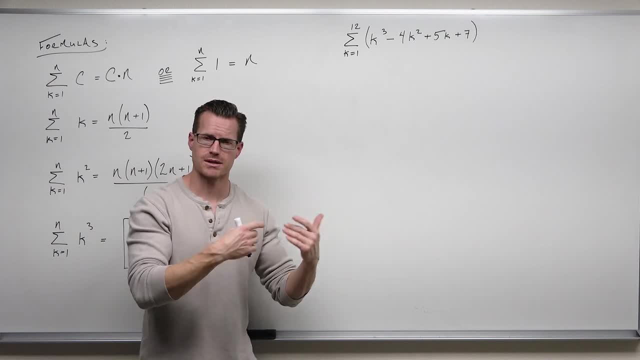 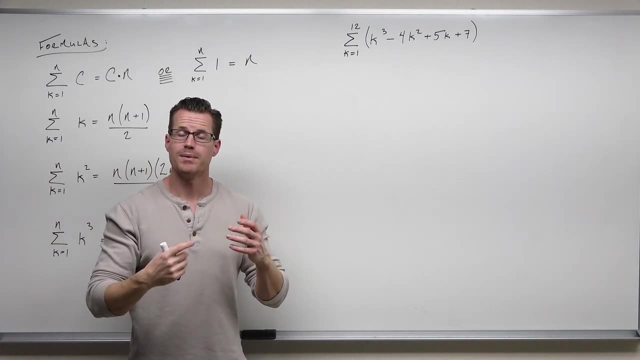 I can separate my series in several different series by pluses and minuses. I can move constants in front of factors in front of my series. Why? Because we know that you can factor out the same thing being multiplied in every single one of your terms: additions, subtractions factorable by multiplication. 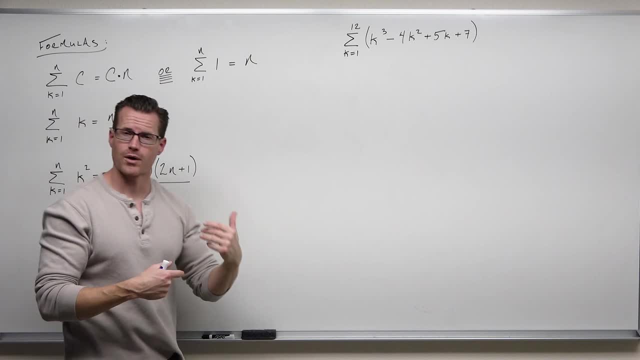 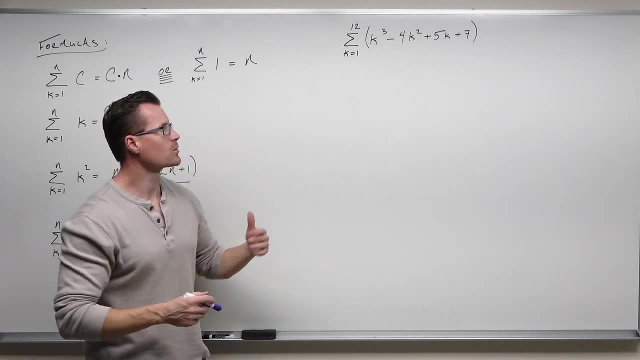 So I can take multiplication and factor it in front of my series. It is factorable, because addition, subtraction is factorable by multiplication. So in other words, I can break this down in some really simple pieces that match up what we have here. 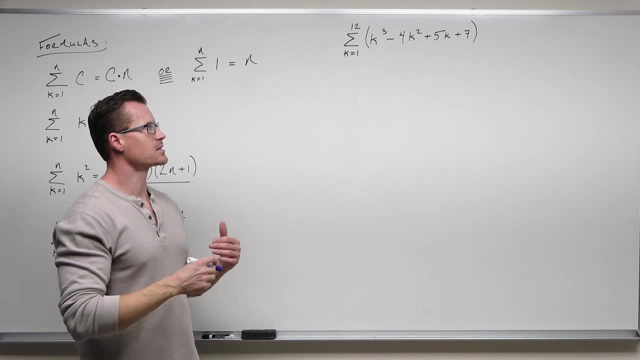 So we're going to do that, We're gonna say: all right, because addition, subtraction is, uh, multiple, it's associative, it's commutative, I can move stuff around, I can separate things. It's also factorable by multiplication. 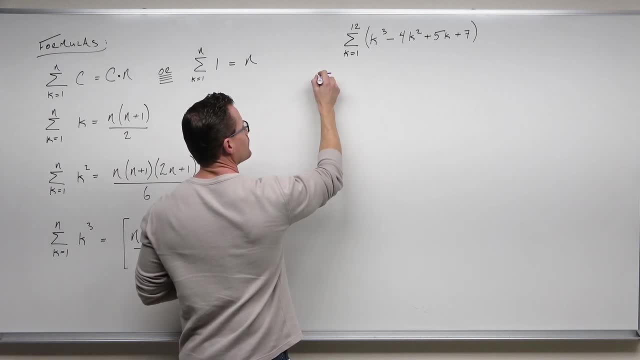 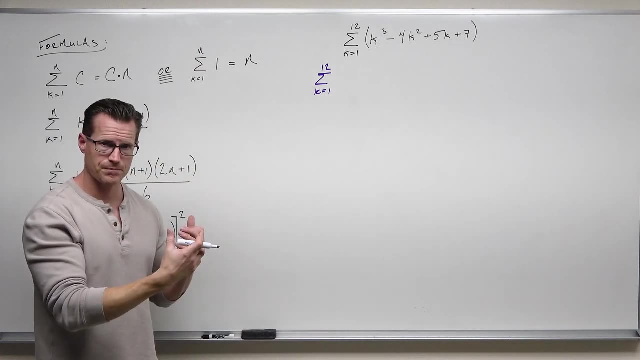 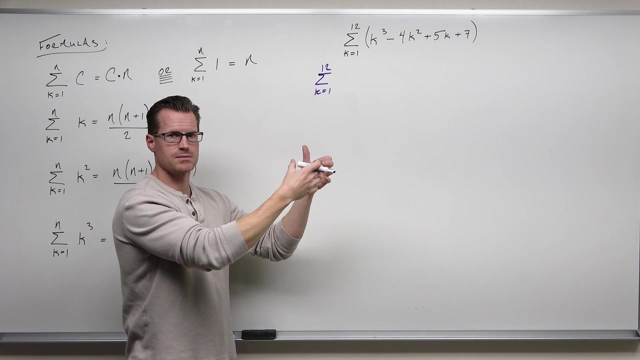 I'm going to start separating this. I'm going to separate it first by addition and subtraction and then pull my factors out, So I can consider one big series to be a sum of little series. adding up different stuff and then adding together is the same thing as adding up all the stuff at once. 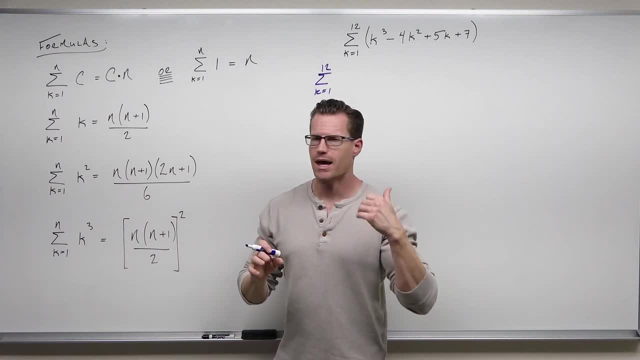 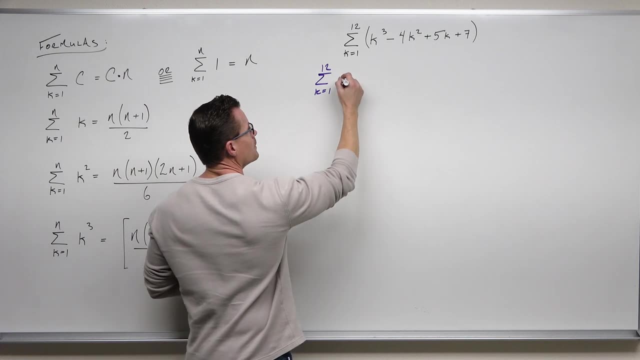 What we're trying to do. our goal is to get the insides of every one of our series to look just like one of these things, And we'll sort of move up and down. but we can sort of, Emma, by adding what's going on in the middle and the part below. I'm just going to 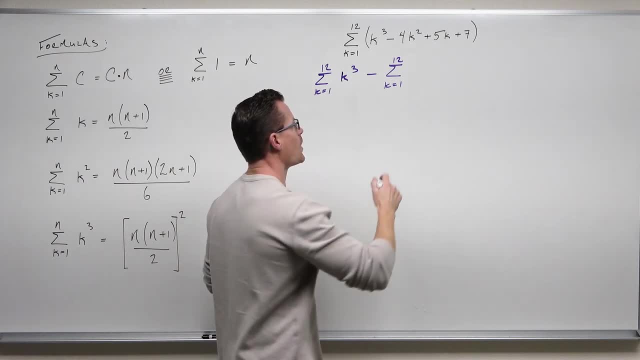 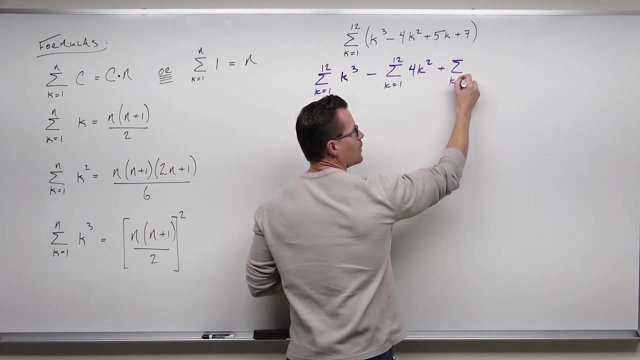 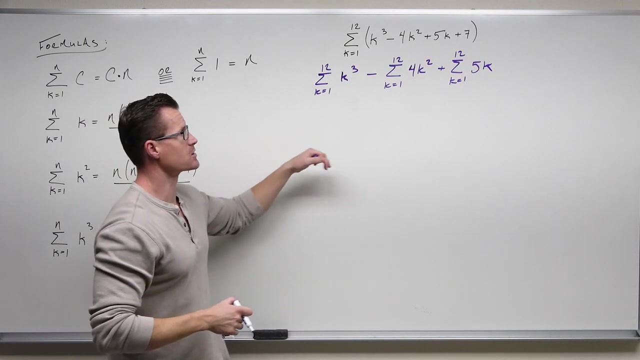 You'll notice that you have to keep the same starting spot and ending spot. You'll also notice I'm not doing a whole lot of work in my head. It's way too easy to start making little mistakes on this, Like forgetting signs or forgetting. 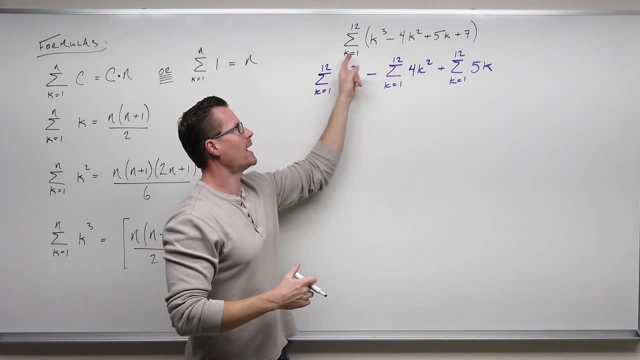 Or if you're, if you want to be smart about it and you'll go. well, I know I can separate that, but I can pull the four out front. That's true, Because the top one has a face. Yeah, There you go. 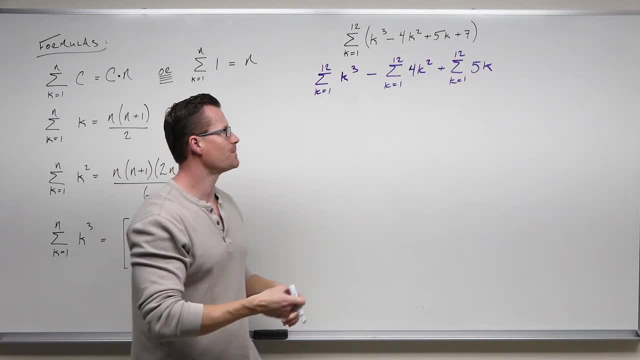 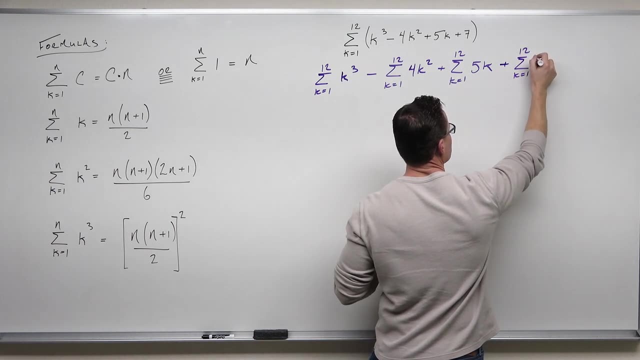 It works well. Yeah, true, but sometimes we just lose the 4 and make a signed error. So I never do it. That's up to you whether you want to. I prefer to write this stuff out, So this series can be represented as 1,, 2,. 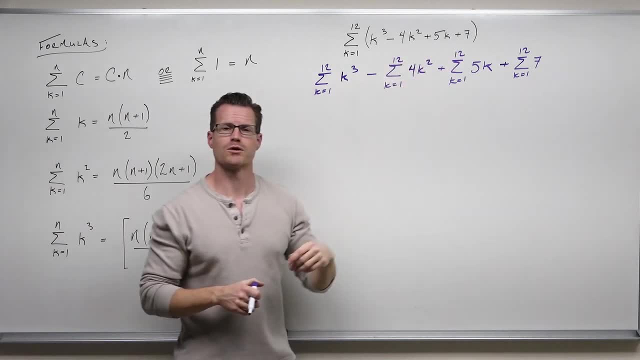 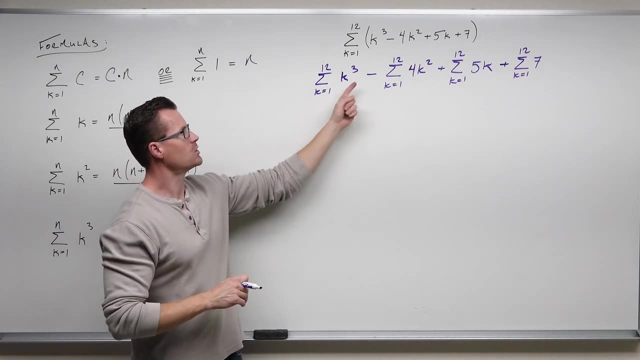 3, 4 different series, because I had 1,, 2,, 3, 4 different terms and we can break that up and we can associate it, group it by addition and subtraction. So k cubed, okay, minus 4k squared. 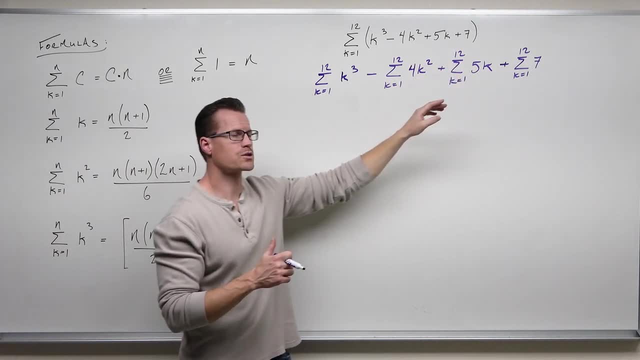 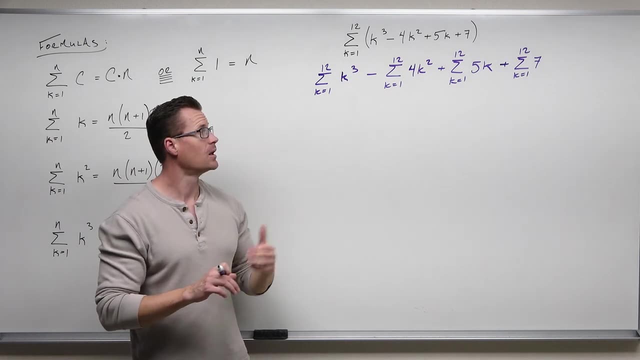 got it plus 5k. cool, plus 7.. You'll also notice I'm keeping the subtraction and the addition. That's fine. We want to make sure that we do understand what's going to happen later, though, that I'm subtracting whatever this gives us. That is important. Now there's some more. 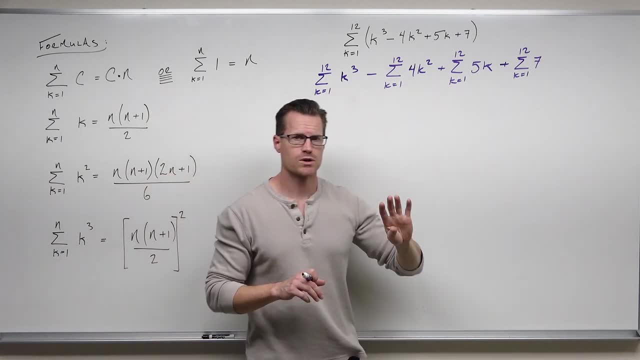 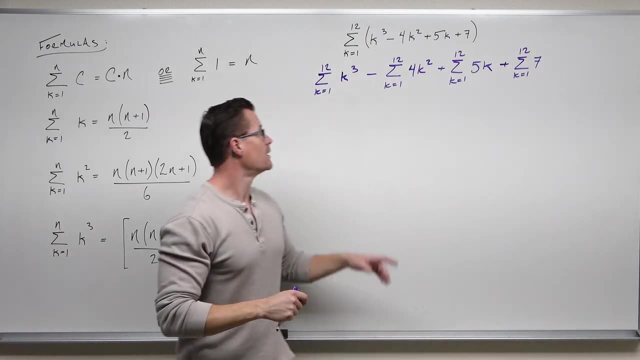 work that I have to do. I need to make sure that the insides of these four series, separated by the four terms that I had, match up with one of these formulas I've given you. So we're going to do that. This is great. K cubed is done. We love that We're going to have a formula for. 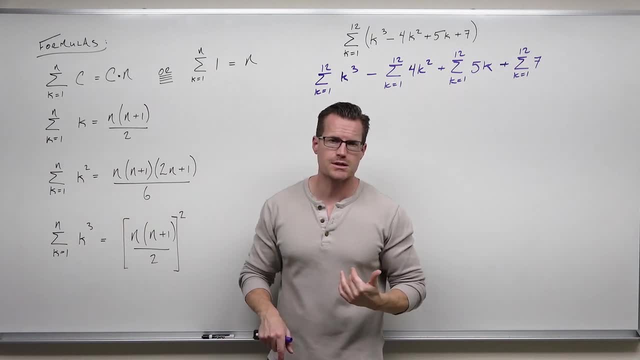 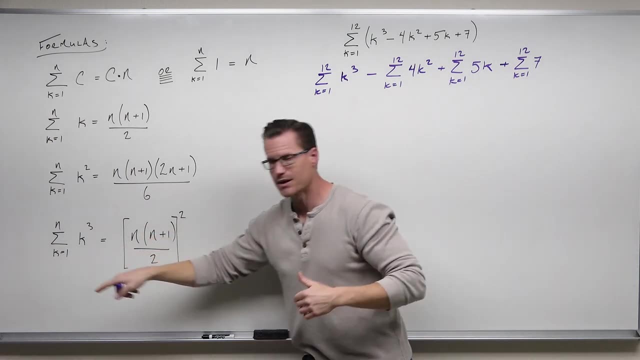 that in just a minute, In fact, it's going to use the 12 that I referenced. I'm going to be putting for this one term, this one series. I'm going to say this starts at 1.. That's what I want. 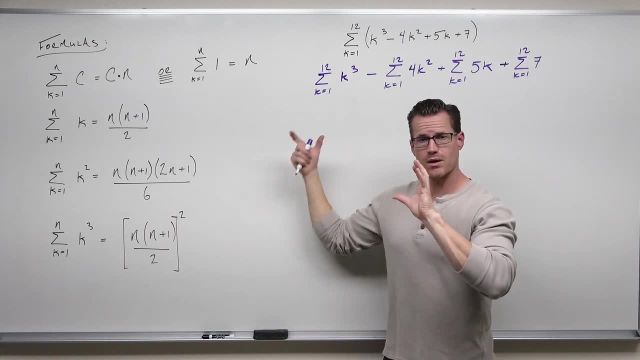 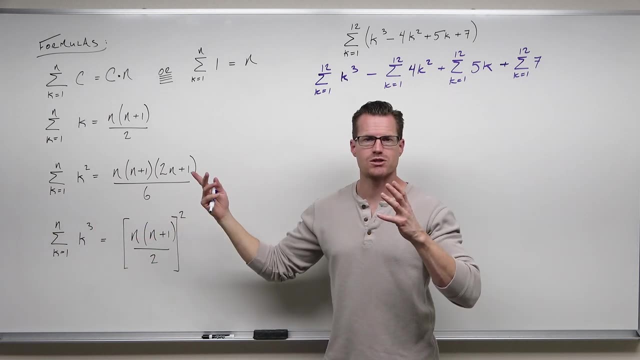 This has a k cubed That matches perfectly. That's the sequence for that mini series- mini series, and then it ends at 12.. 12 is going to get plugged in here and here and I'm going to square whatever. I think it was 78 that I said. 78 squared is what that is going. 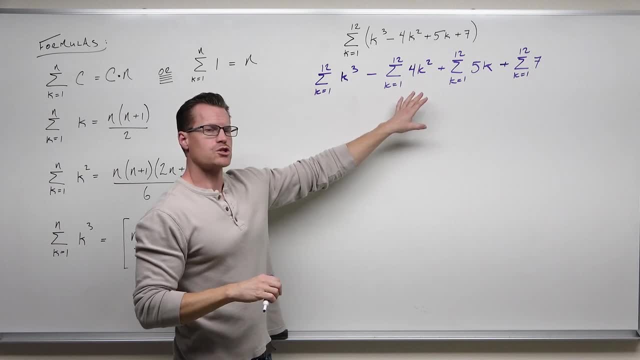 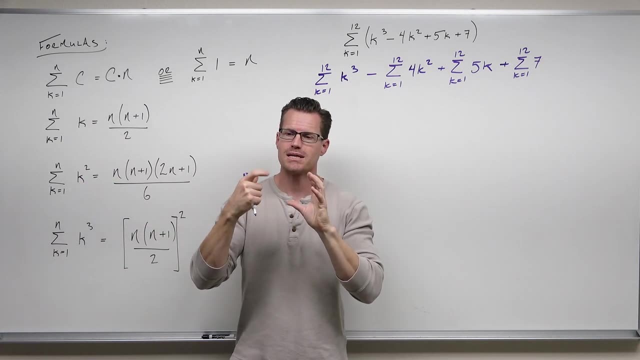 to be. We're done with that one, This one not so much. So this one says: I have very close to what that says, but there's a 4.. That 4, because that 4, man, I hope you see it, That 4 would be on every single term in the things that. 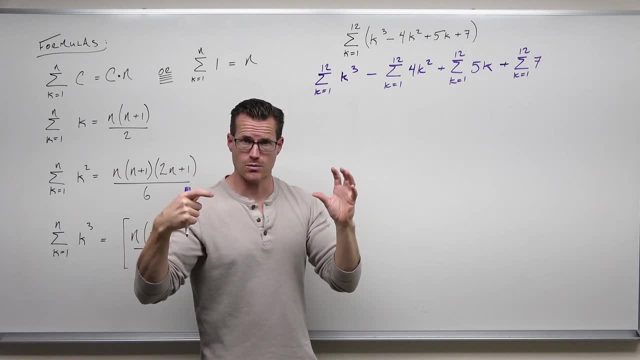 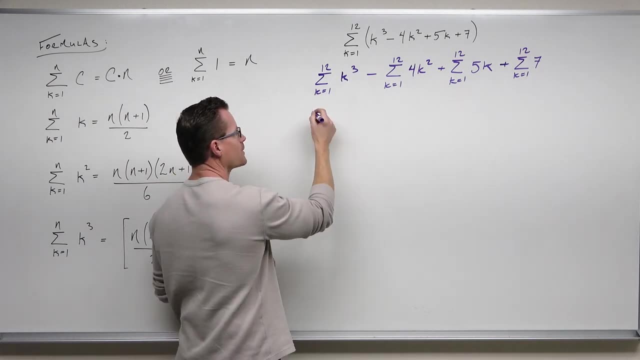 are being added. It's factorable. You could factor it out of every term right. That means you could factor it and move it in front of that stuff that's being added. It's factorable. That means you can move that 4 out front. 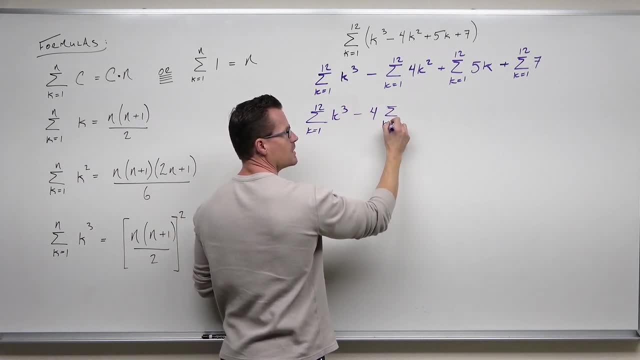 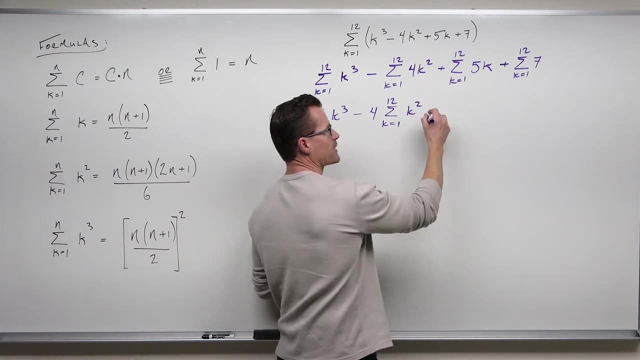 I hope you're all good. I'm also seeing why I'm not giving you lots of different examples. This pretty much covers everything that you do, except for one example, which I'll show you in just a minute. Same thing here. You could factor out a 5 from every one of those terms, so we can move our 5 in front. 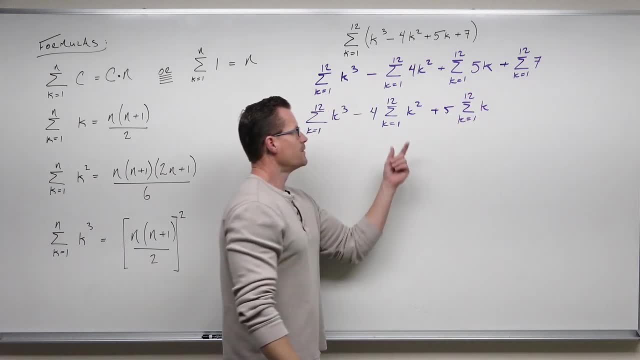 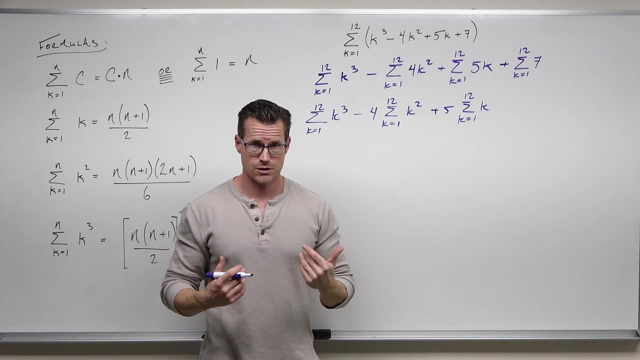 just like a factor does This k squared is what we're looking for. This k is what we're looking for Now. the constant. you can do one of two ways. It doesn't matter to me which one you do. You can leave it as this. 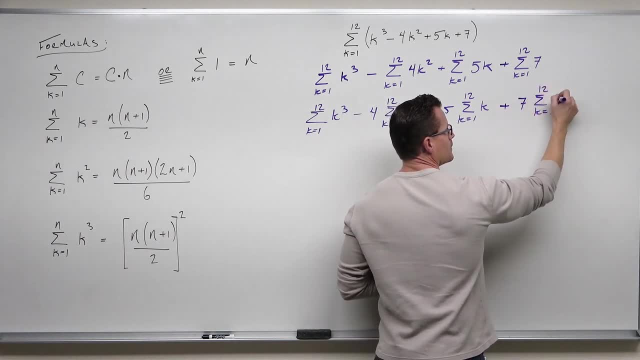 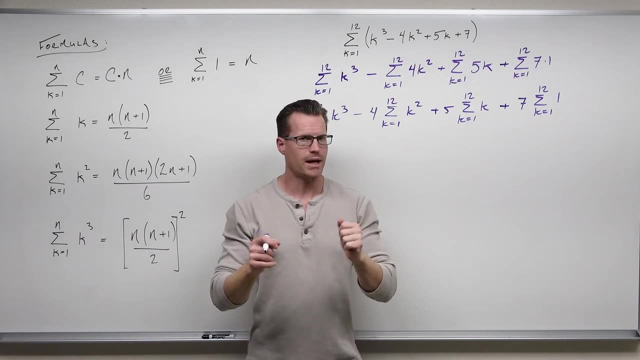 or you can write it thinking of it as 7,, not 71,, 7 times 1.. You can pull out the 7 and leave the 1.. Either way, I need you to see if you do the same thing. If you leave it as a 7, you do 12 times 7.. 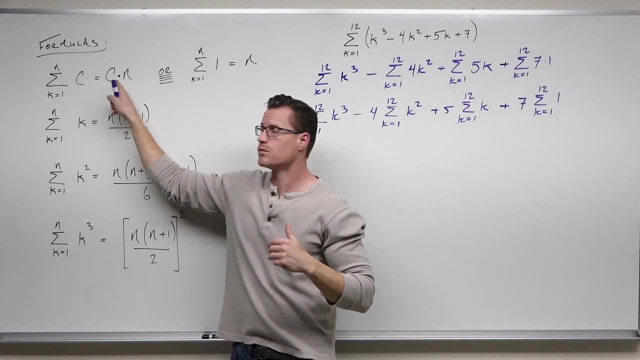 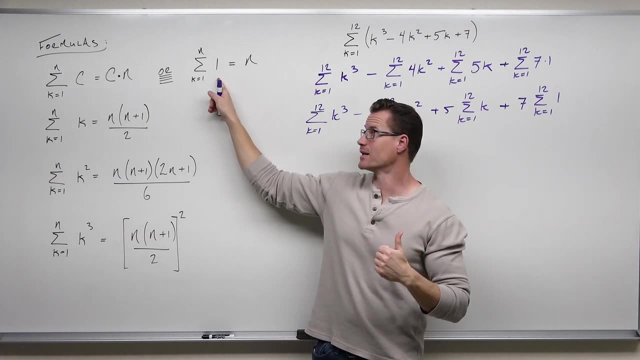 That's what that says. Leave it as a 7, a constant. You would do n 12, times 7.. No problem, If you do it like this, you say: all right, if I am adding up lots of 1s, how many 1s am I adding? 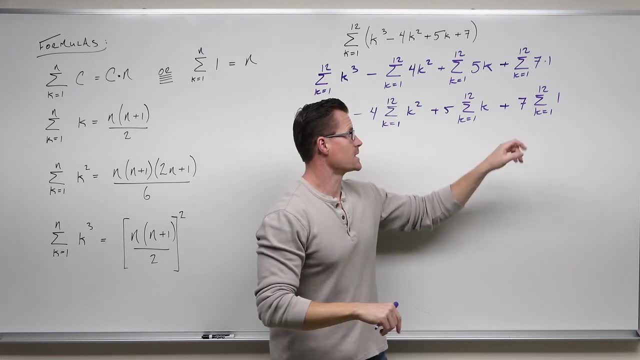 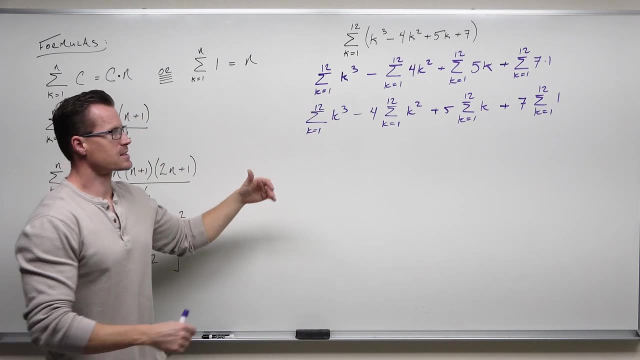 12.. You're n, You're 12.. So you'd say here's 12 times 7.. Either way, you're going to get 12 times 7.. It doesn't really matter. What matters is being able to separate this into our number of terms gives. 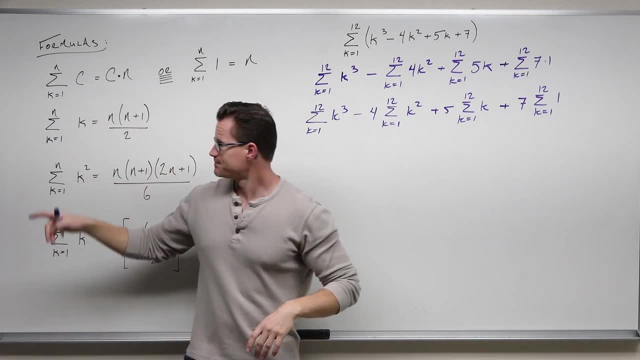 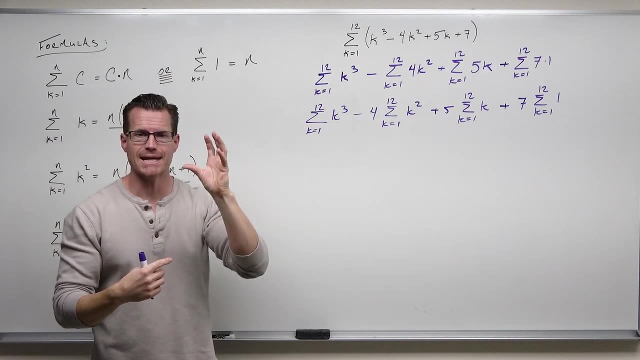 me number of series, Then making every one of those series look like something we have a formula for and then applying the formula correctly. So the formulas are all based on your n. where you end Your n is where you end your series. I know that sounds similar when I say it. 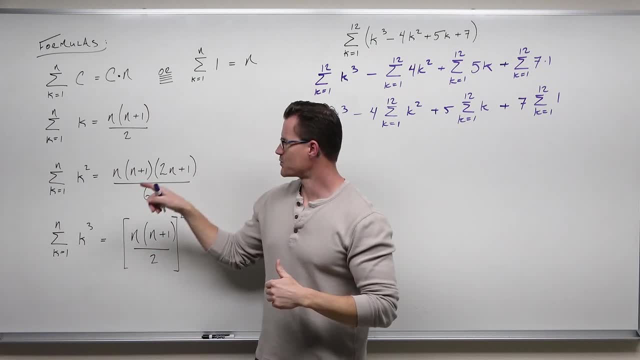 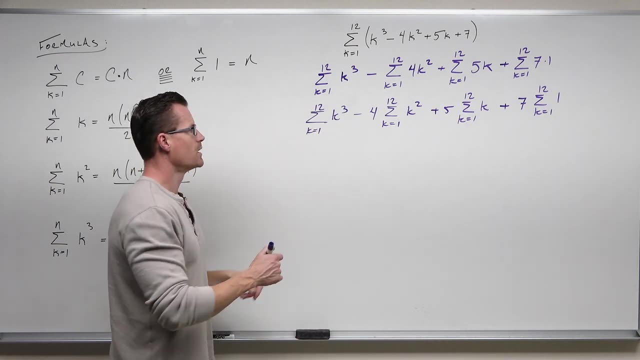 So our k cubed says there's a formula for it. Remember that It's right there. So I'm going to take my ending value, my n. I'm going to plug it in My ending value, my n is 12.. So I'm going to apply this formula and say that this part 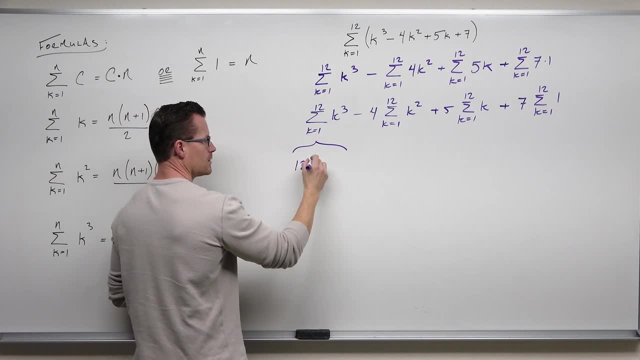 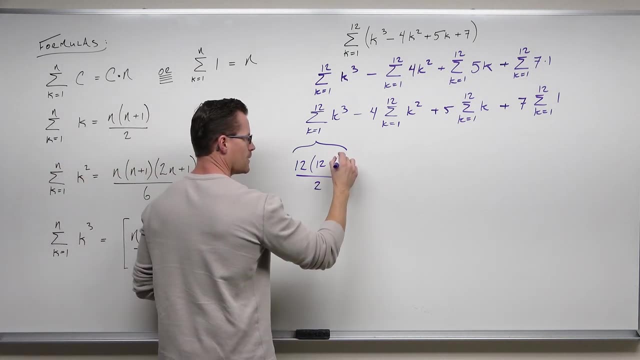 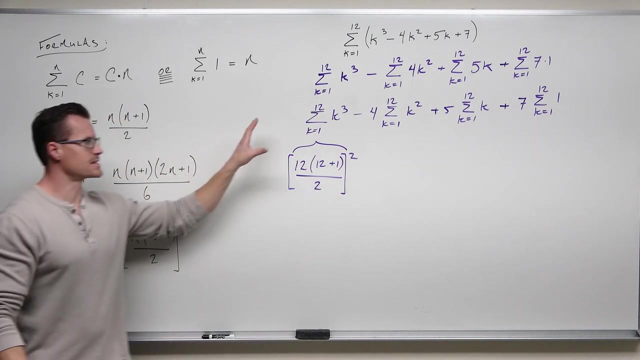 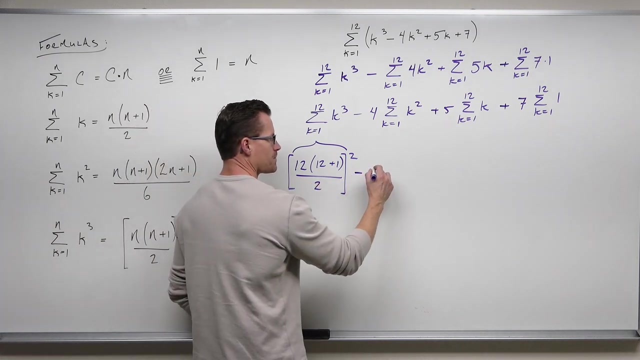 is 12,, 12 plus 1 over 2 squared. This is exactly what that's going to look like. That should be. I should take my n, plug it in appropriately and then we're going to do the math a little later. Minus 4 times, keep that 4.. Don't lose it. Remember that's being multiplied. 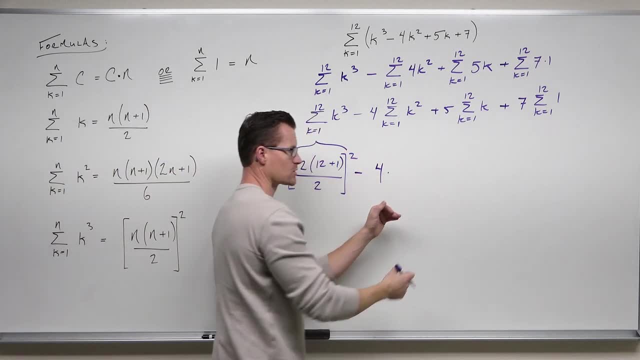 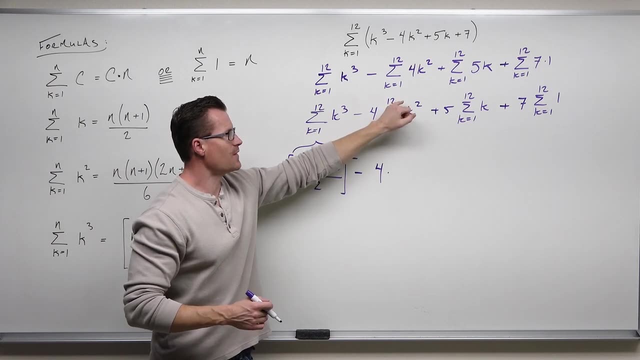 by whatever you get out of this. The sum is represented in this expression that we're about to write, But 4 gets multiplied because that is the factor you factored out. Now, because this is based on our k squared, this is: find your ending value, your n. Here's our k squared, Here's our. 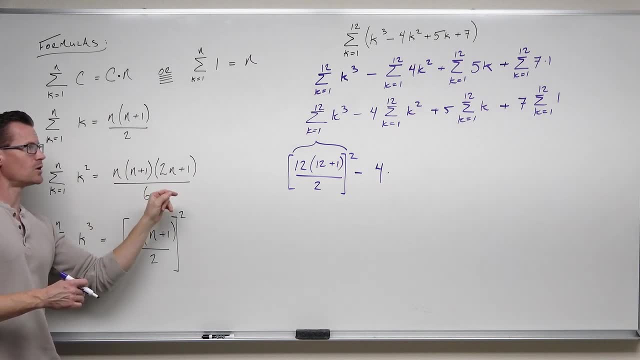 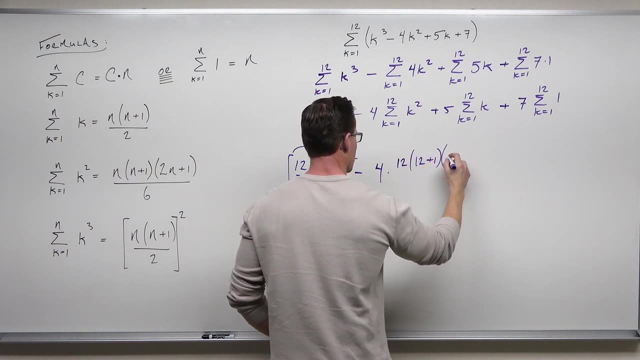 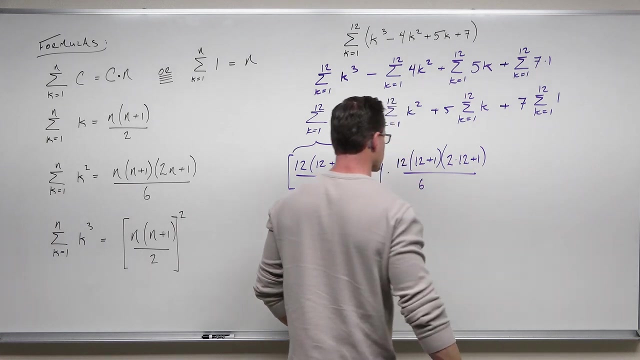 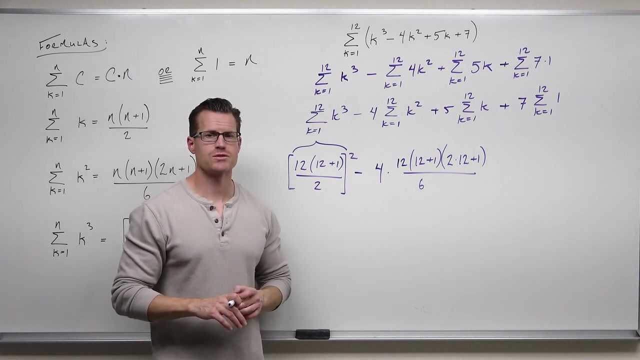 formula for k squared: Just plug in your n, 12,, 12, and 12.. Our n is 12.. A good question would be: will you ever get fractions out of this? Nope, They'll all work out to whole numbers. So if you're getting a whole lot of fractions, you're doing something. 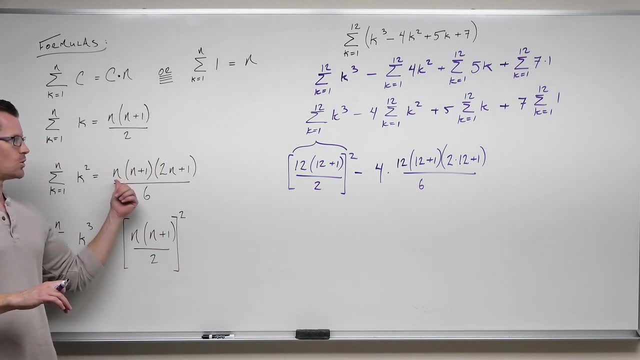 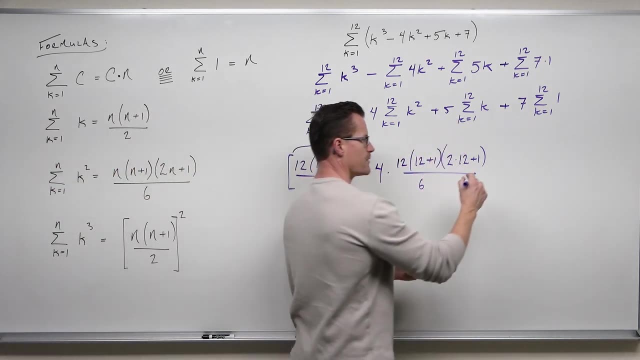 wrong. Those fractions should simplify. So we have a 12,, 12 plus 1, and 2 times 12 plus 1.. That's coming from our n. Then we do our plus 5. So we have a plus. 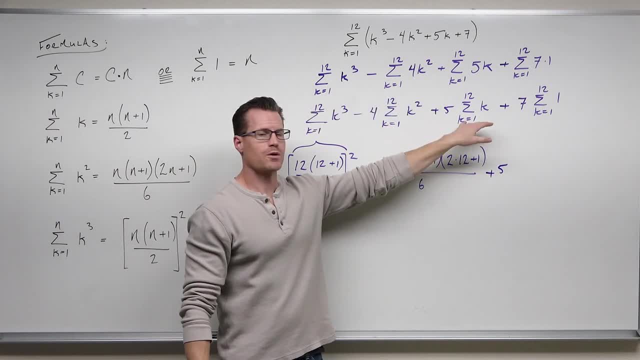 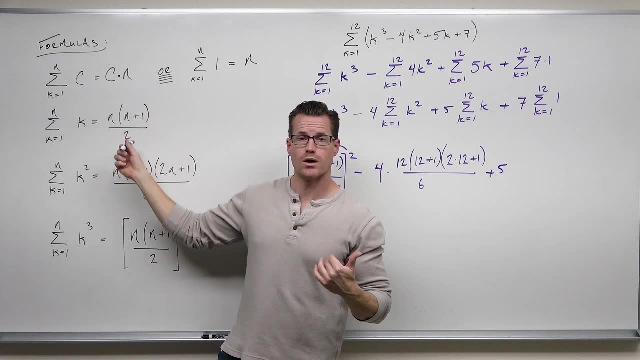 We have a 5.. And then we look at the formula for that series. Since it's based on k, we're going to go all right. We have an n of 12.. I'm going to plug in 12,, 12 plus 1 over 2.. 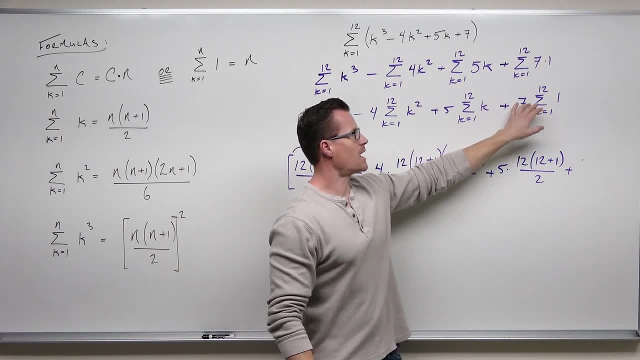 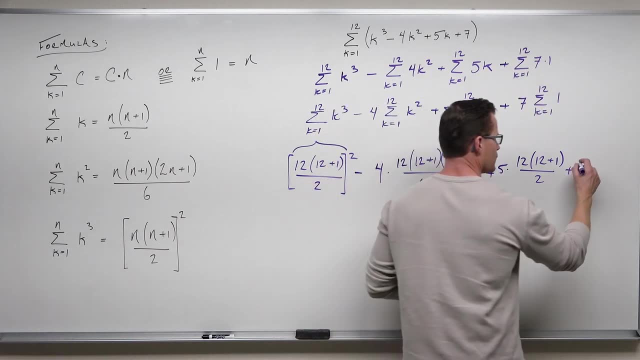 Lastly, no matter what you do, you'll get 7 times n, which is 12, or 7 times 12.. Either way, you're going to get 7 times 12.. And we've already talked about why that is. You're welcome to plug that in just like that. 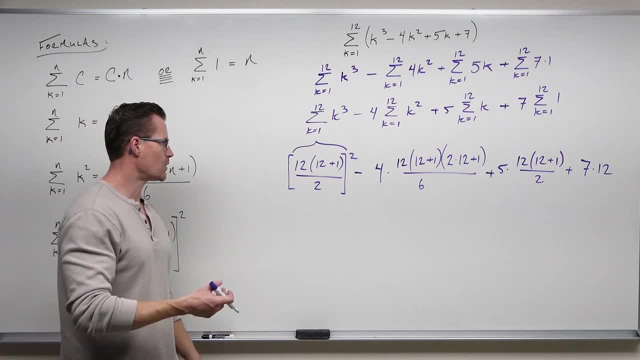 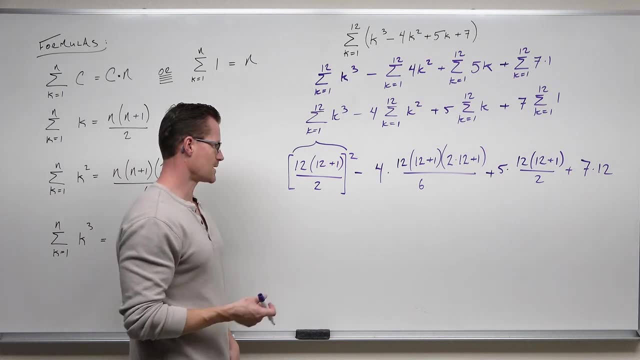 on your calculator and get whatever it is that this equals. You can also- you're welcome- to simplify this stuff, however it seems best to you to do. I'll simplify it, because I don't have a calculator handy. I would do things like this: I'd simplify all of my fractions. 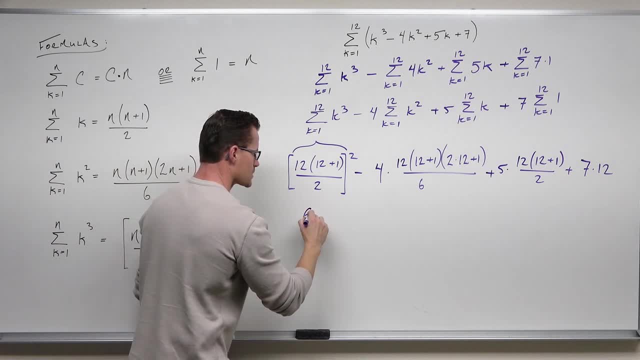 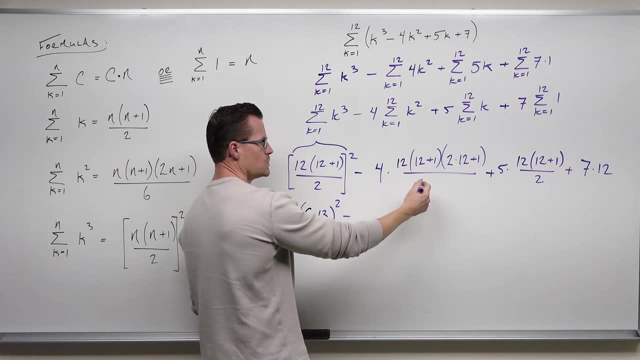 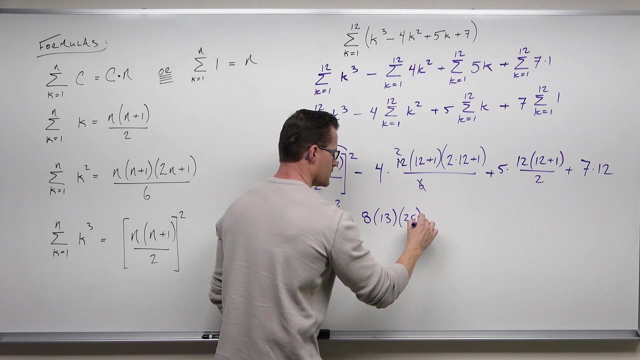 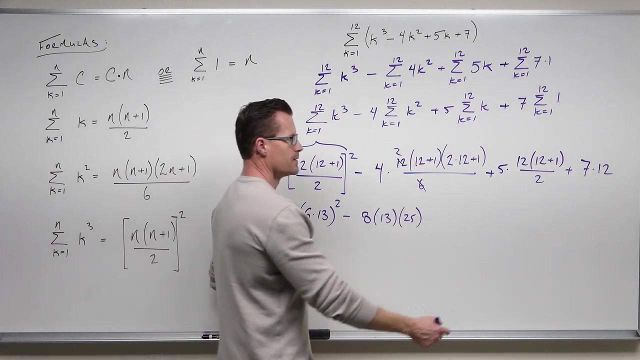 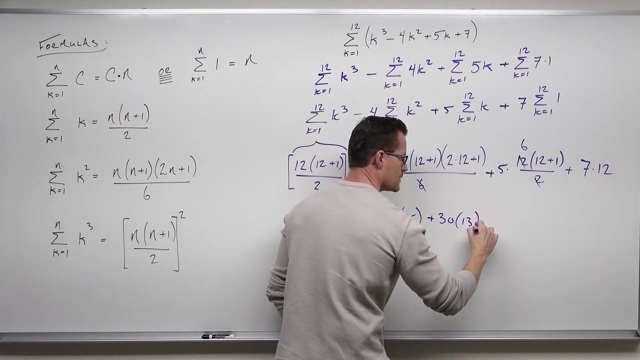 because they all will. So this is going to be 6 times 13 squared minus. This would give us: 2 times 4 is 8.. So 4 times 2 is 8, 13, 25.. This is going to give us 6.. That would be 30.. 5 times 6 is 30 times 13 plus 84. 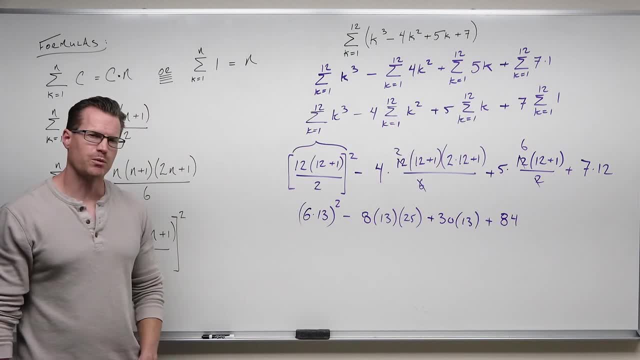 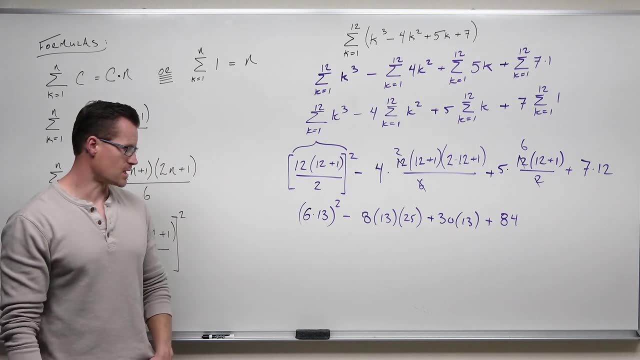 That's probably what I'd plug into my calculator. I might double check it to make sure that I did everything right, But I'm going to come back with the answer here. the sum in just a bit Okay, barring any little mistakes that I've made I could have. I don't know. 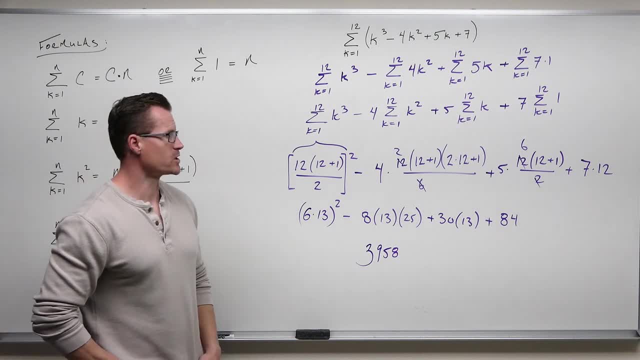 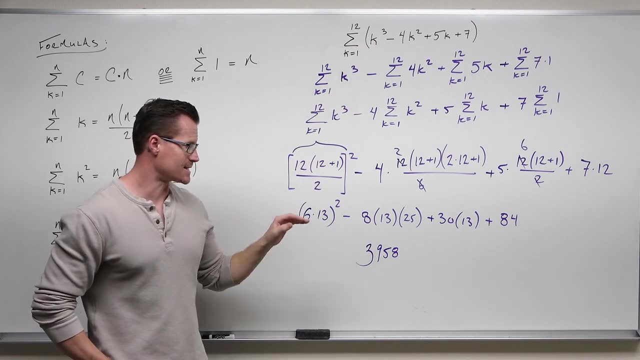 I haven't really looked back at it yet, But if I've made any mistakes, then they should be small errors. But if I haven't, then that is the sum that you get by adding up the 12 terms of that sequence, And that's exactly what you should get there. You can try it, I suppose. 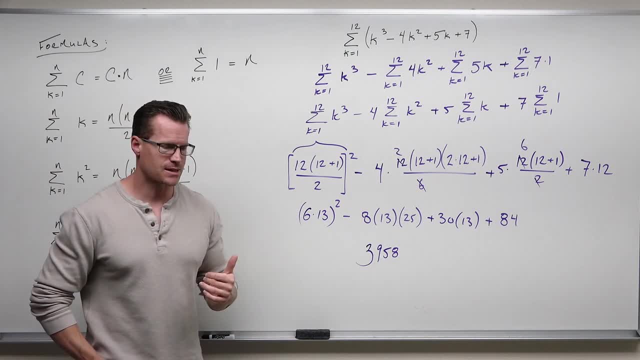 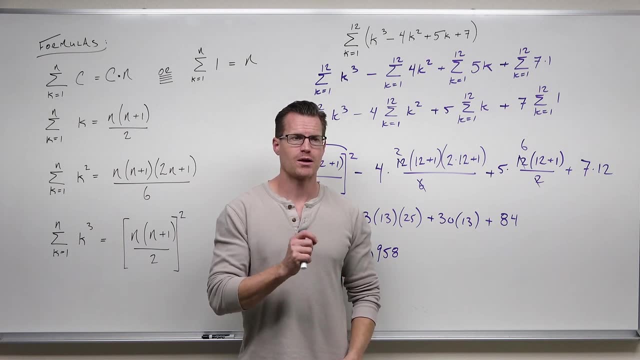 If you really wanted to, But that's what you should get, So I hope it made it make sense. as far as how to manipulate a series in something that's manageable by the formulas that I've given you, I'm going to give you one more example about how to manipulate something that doesn't match. 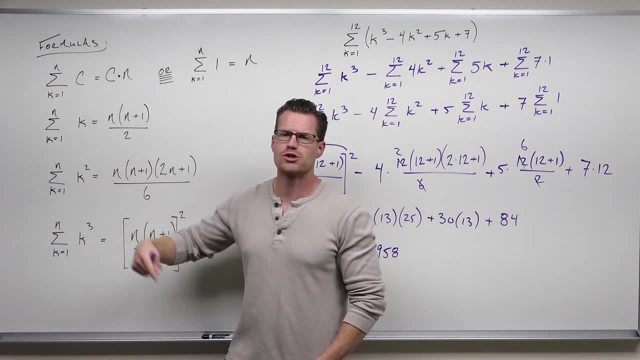 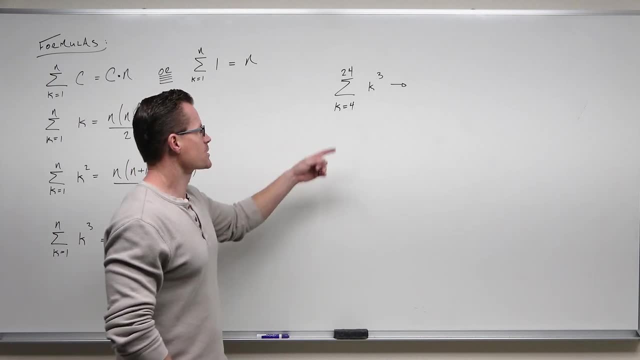 this Like: what if you don't start at 1?? What if you start at like 4?? I'll show you how to do that. All right, so what do you do when it doesn't match up with where you're supposed to start? 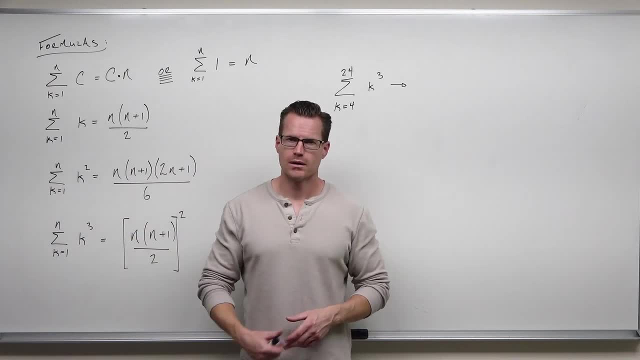 Like, if you start at k equals 4 and you're supposed to start at k equals 1, is this going to work? No, And don't try to make it work. the way it is right now. It will not work. So let's be smart about it. What if it? 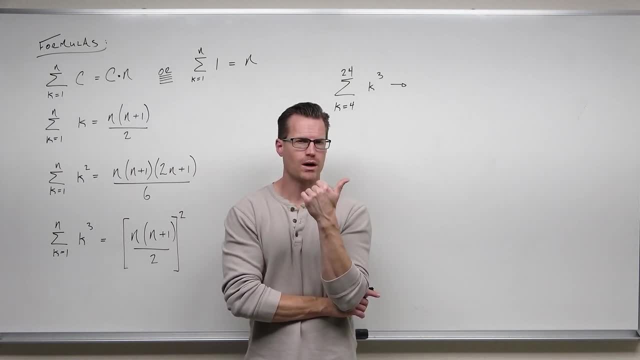 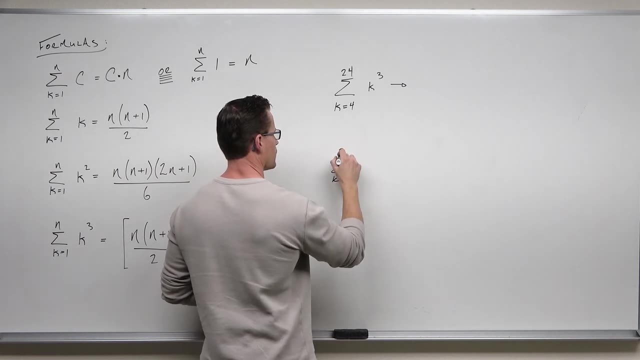 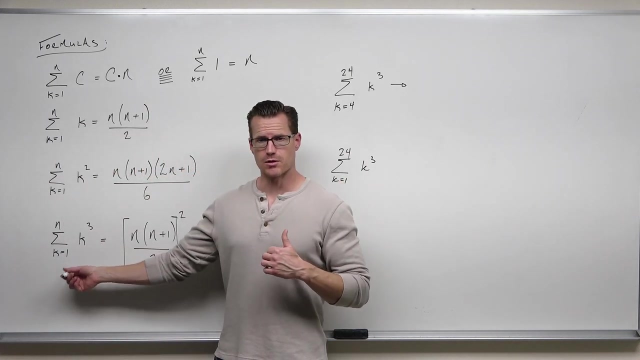 what if it was a 1?? Like, could you make it work if it was a 1?? If it was that, it'd be fine. We could say, yeah, okay, I know that. that matches perfectly this. I know what the formula is, I know. 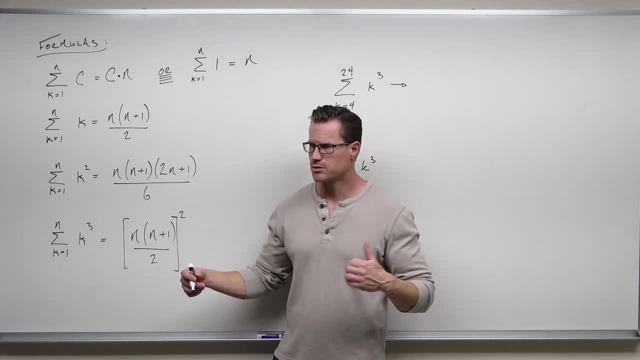 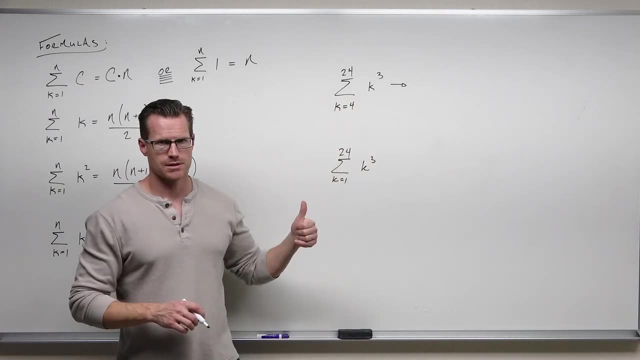 I'm ending at 24.. I'm putting 24,, 24 plus 1 over 2, and then take that and square it. You find the sum of the series Very quick and easy. The problem is is that this is not what this is, So 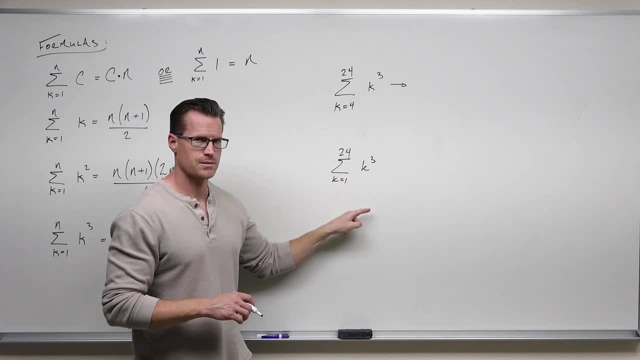 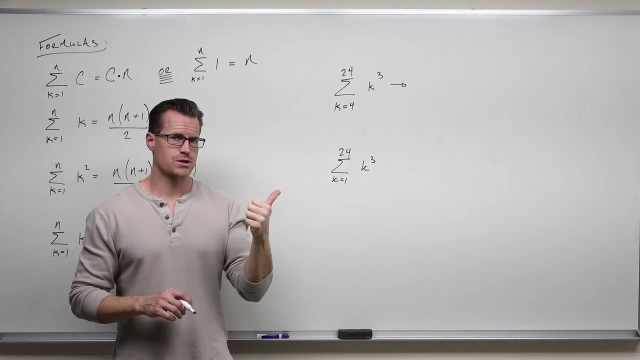 what is this compared to this? Let's think about what I don't want out of this. I don't want the first term, I don't want the second term And I don't want the third term in that series. I do want the fourth, fifth, sixth, seventh, eighth, ninth and tenth. So here's how we can think. 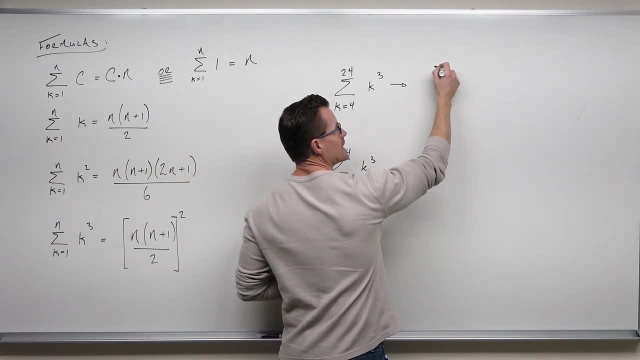 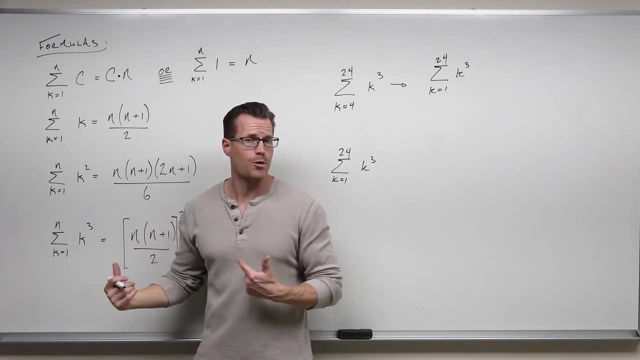 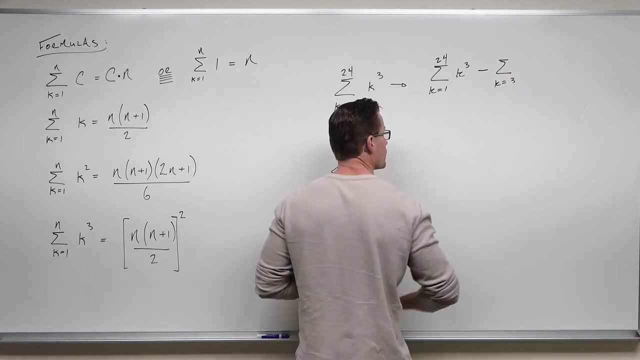 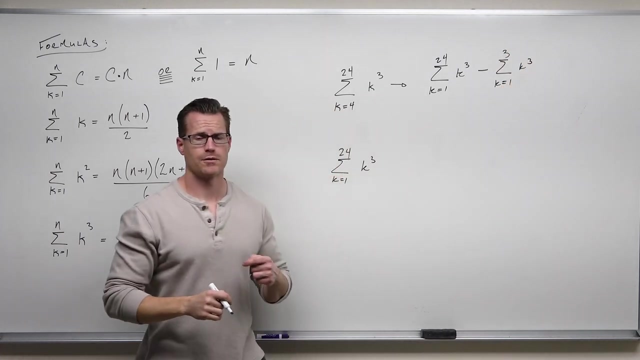 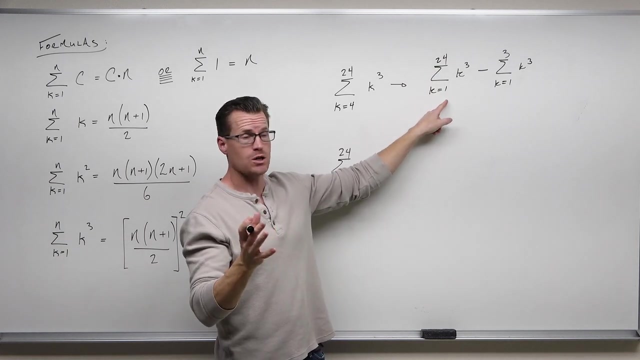 about it. This series is the same thing as taking the whole series that that formula needs and removing the first three terms. I hope that you see what this does. This says: here's my whole series. What don't I want here? I don't want terms 1,, 2, and 3.. This is terms 1,. 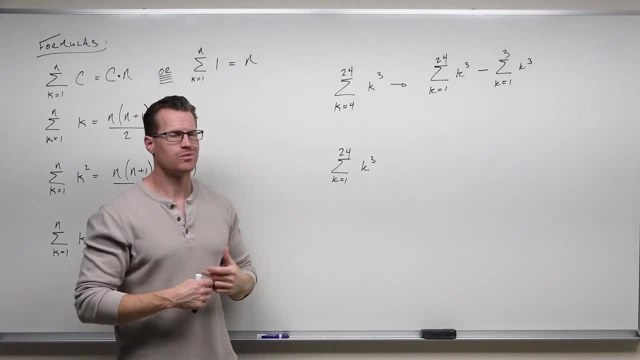 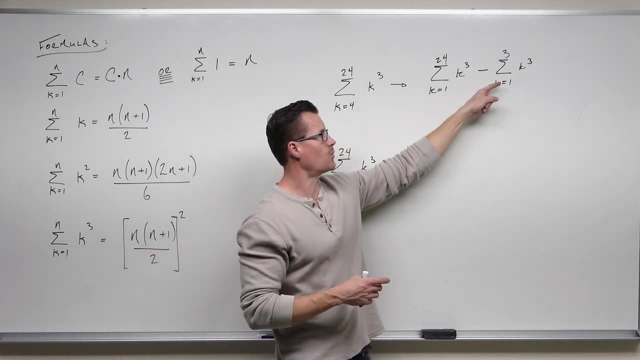 2, and 3 of that series. So we can always always really do that, If you don't start at 1, take the whole series and subtract off, starting from 1 to all the stuff that you don't need. So 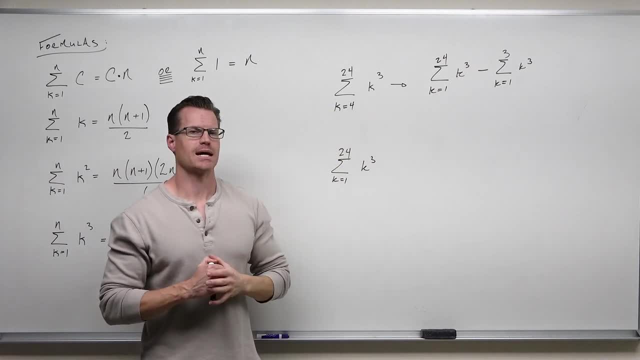 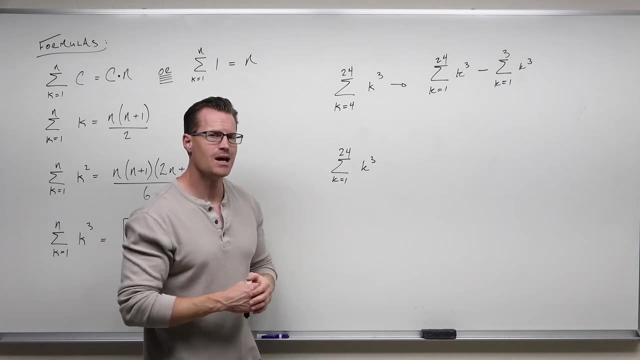 up to, but not including that, that beginning index, that beginning term. So hopefully that you can see that that actually does work. I should kind of make sense. You just have to start at 1 in order for these, these formulas, to work, Otherwise you're going to start subtracting things, And this is the way. 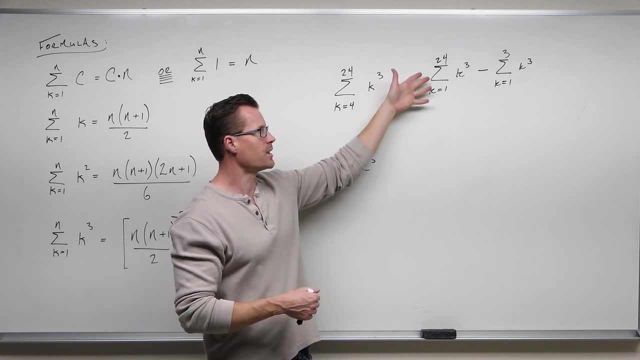 that we do it. You know I want from 4 to 24.. I want the whole thing, but I don't want the first three terms. That's the first three terms. but I can work that out for you. You can easily do. 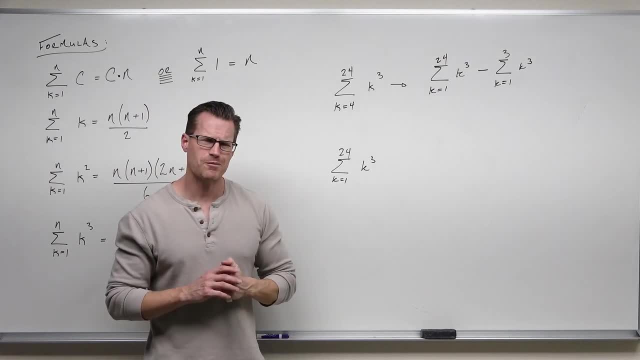 that on your own. I just want to show you. that's the process we're going through, So I hope it made it make sense. I hope now that sequences and series aren't a huge mystery to you. I hope that you can see they're very manageable. We even have some formulas for series that really 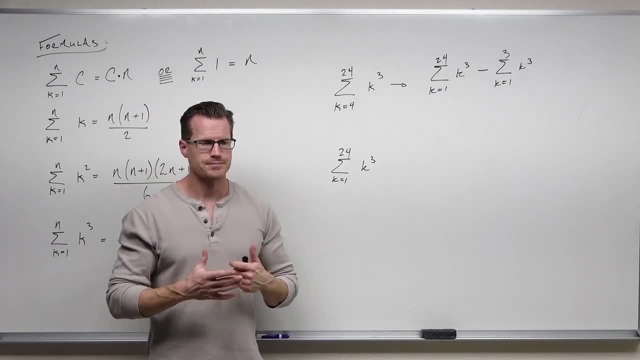 really help us. So we're going to start talking about specific sequences and series. over the next four videos. We'll talk about arithmetic sequences, then arithmetic series, geometric sequences then geometric series and, finally, how to prove some of these formulas with a proof by induction.